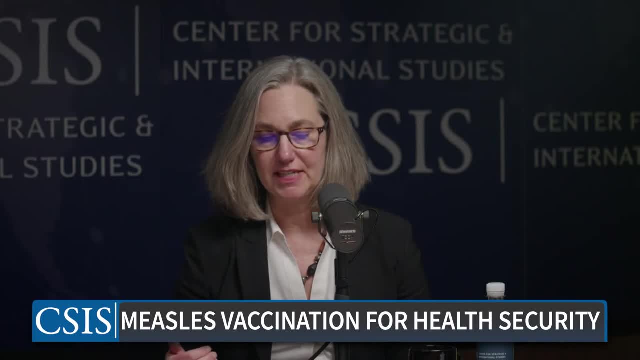 That same year, the Measles Initiative was able to create a vaccine for measles in the United States. Several countries lost their elimination status as they saw sustained measles transmission within their borders. Now, while reported cases of measles decreased during the first few years of the COVID-19 pandemic, when people wore masks and practiced, 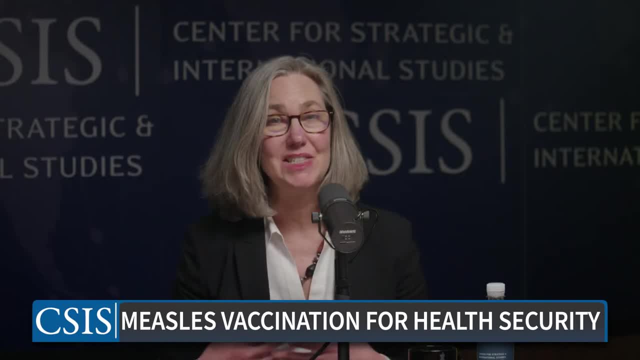 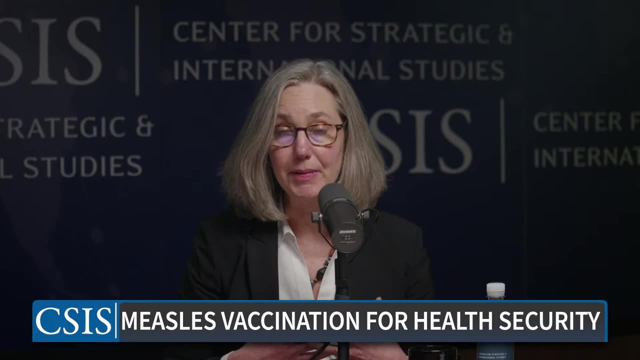 social distancing and often avoided healthcare settings. cases rose again in 2022. And in 2023, there were outbreaks in several countries, including Yemen, India, Kazakhstan and Ethiopia, particularly in regions or subregions where immunization coverage gaps had widened during. 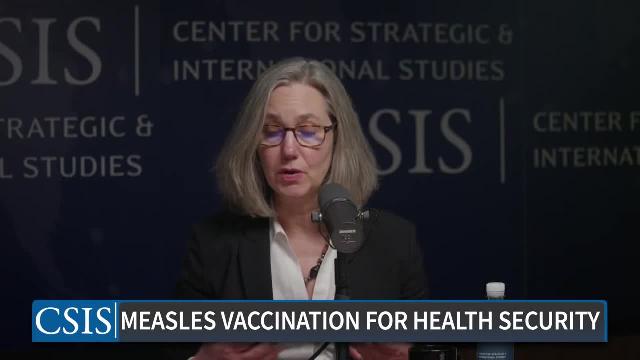 the pandemic And just a few weeks into 2024,. we've seen cases here in Washington DC, at least in the area airports, as well as Philadelphia and Atlanta- and in the United Kingdom, where low coverage and a surge in cases prompted the government recently to declare a. 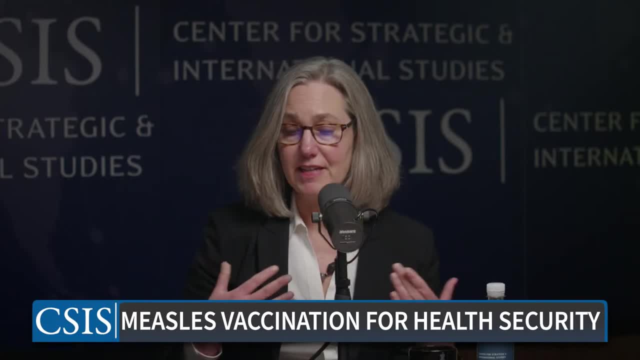 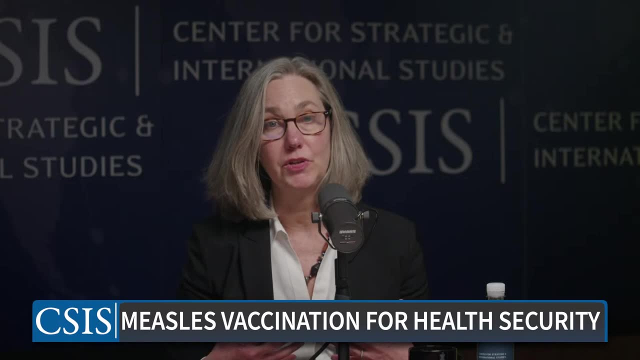 national health incident. Now. preventing measles through effective routine immunization is a lot simpler than detecting an outbreak and then launching a vaccine, But the government has taken a step forward in protecting an outbreak and then launching a campaign to find children who missed getting vaccinated during routine health appointments. It's a lot less expensive. 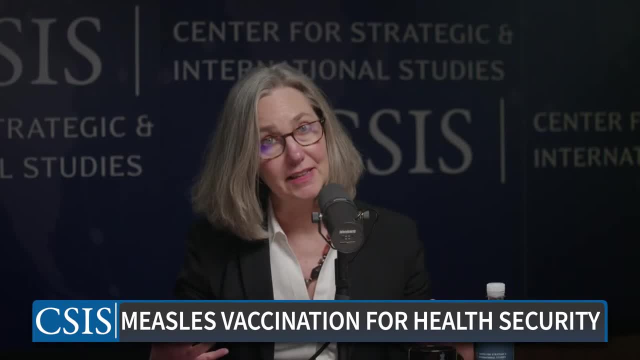 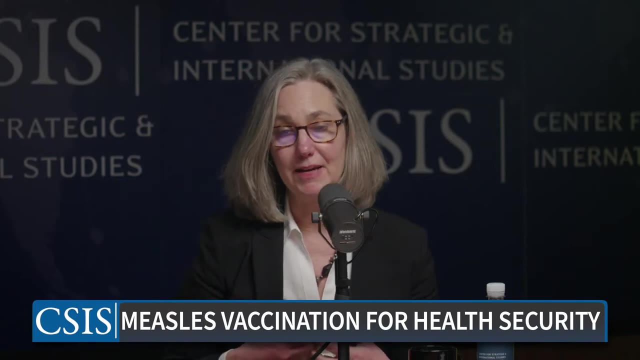 too. So if that's the case, why is it that we're seeing outbreaks now and what can we do to change the situation? Hello and welcome to today's event on increasing measles vaccination coverage to improve global health security. My name is Catherine Bliss. I'm a senior fellow. 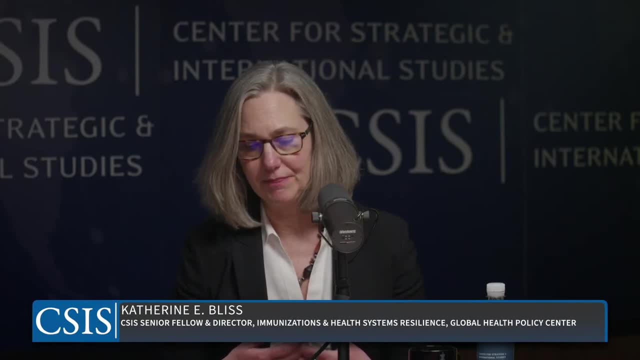 with the CSIS Global Health Association. I'm a senior fellow with the CSIS Global Health Policy Center, where I lead work on immunizations and health systems resilience under the Bipartisan Alliance for Global Health Security. It's my pleasure to welcome our three expert. 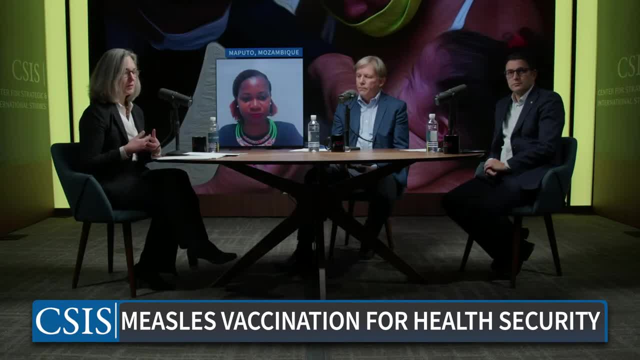 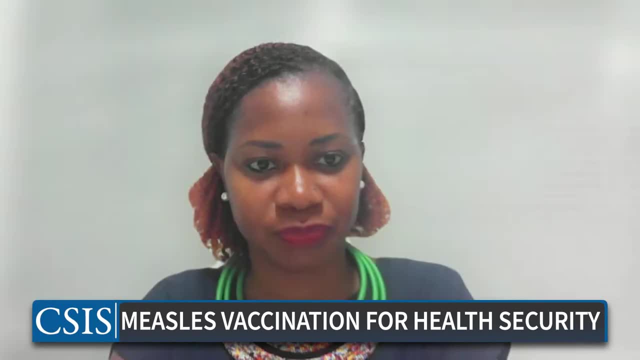 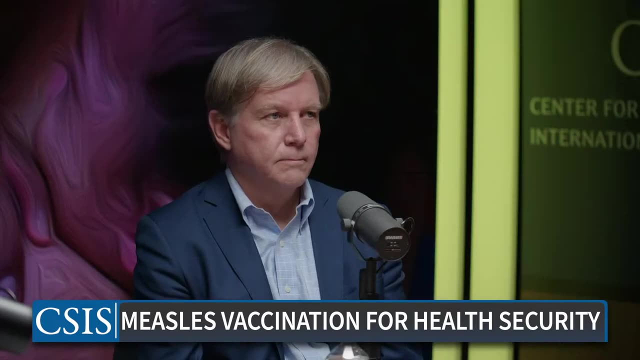 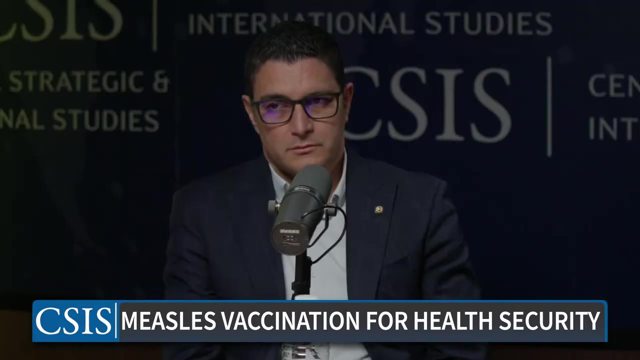 speakers today: Graca Matsinya, who leads work on the Momentum Routine Immunization: Transformation and Equity Project in Mozambique. William Moss, professor and executive director of the International Vaccine Access Center At the Johns Hopkins University Bloomberg School of Public Health. And Daniel Salas-Perasa, executive manager of the Comprehensive Immunization Unit at 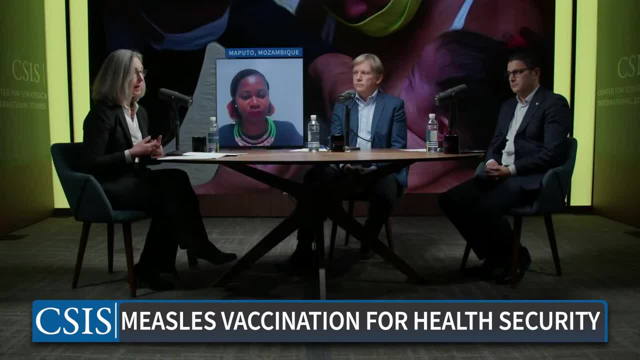 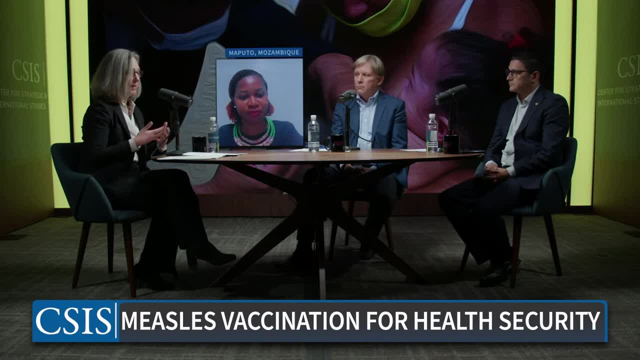 a lot of progress. We've seen a lot of progress. We've seen a lot of progress. We've seen a lot of progress in working to increase immunization coverage In key areas around the world. we saw these outbreaks in 2018 and 2019.. Now, after a bit of a lull during the pandemic, 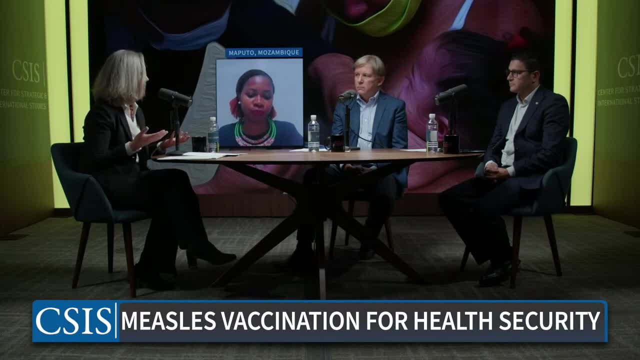 we're seeing another rise in cases. The data last year that suggested that there's been a bit of a bump up and improvement in coverage globally. But we know that that masks a number of challenges at national level and at sub-regional levels as well. 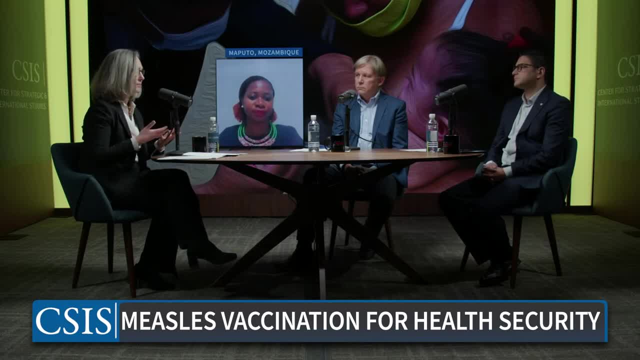 So I want to ask you, kind of looking at the countries where you're doing research or where you're based, from your perspective, what is driving these current trends and what are your greatest concerns as you look at the areas that you focus on over the next couple? 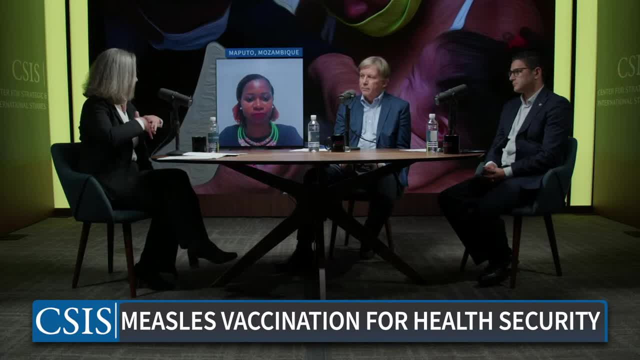 of years. Bill, let me start with you. You're with IVAC, which really kind of looks at these issues at a global level, but you've been working on measles in Zambia and elsewhere for several decades. What are you seeing kind of globally? that's really kind of driving some of this. 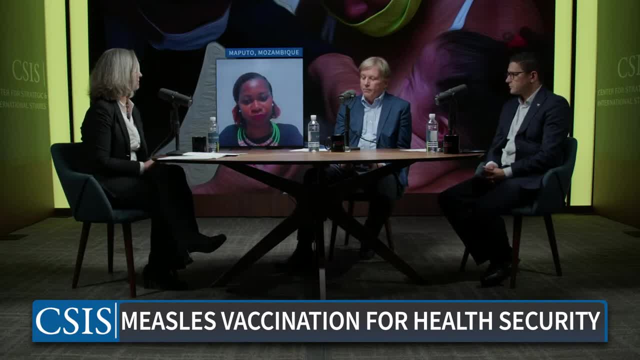 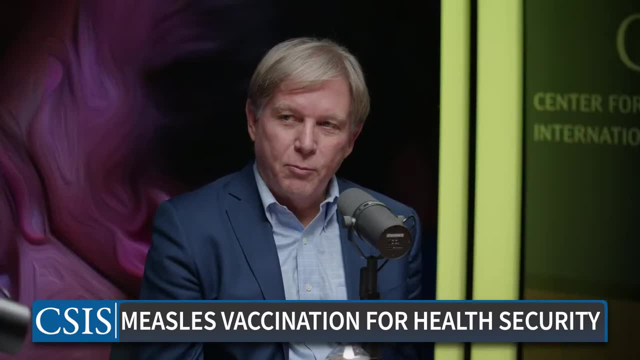 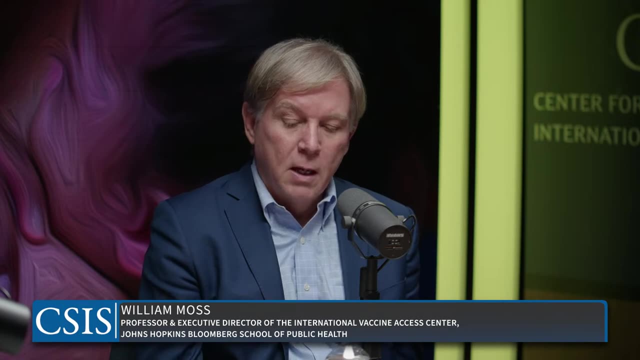 Yes, Thank you, Catherine, And I think this is a really important seminar to talk about these issues. It takes two things: to have a measles outbreak, You have to have a susceptible population and you have to have the virus introduced into that susceptible population. 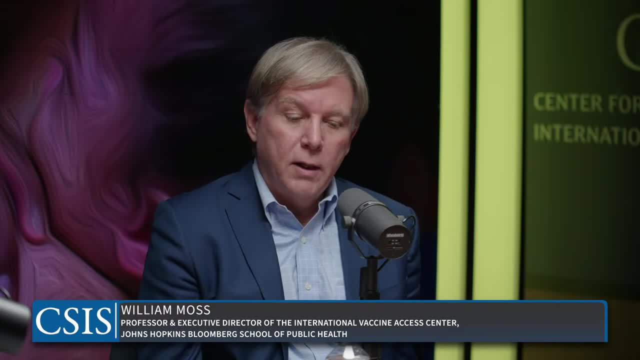 And you know the way I kind of look at this is really global measles vaccine coverage with the first, The first dose has really stagnated at about 85% over the past 15 years. So we've really had this problem of reaching those 15% of children who have not received. 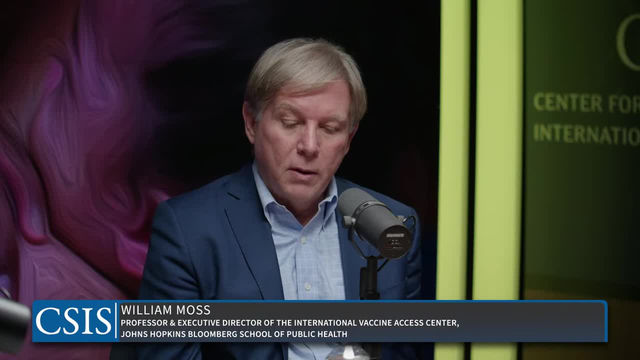 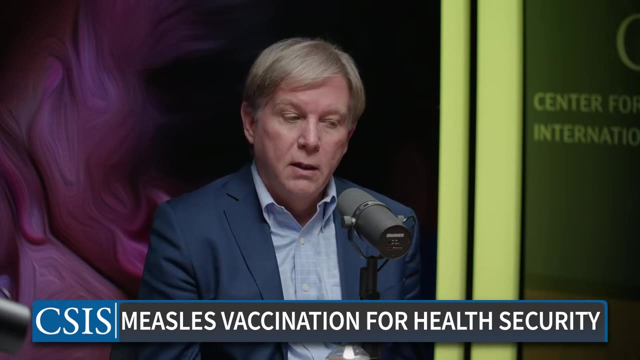 the first dose of measles vaccine. So, yes, we've made enormous progress and, yes, we saw a resurgence of measles in 2019, and particularly globally and here in the United States. This is actually, I think, a longer standing challenge of reaching the hard to reach children. 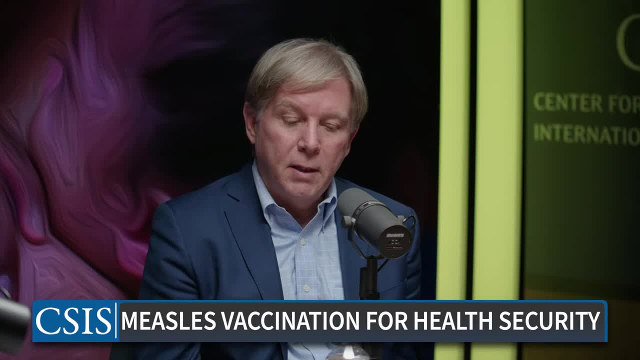 those 15% with measles vaccines. As you said, the epidemiology during the course of the COVID-19 pandemic very really interesting. We had this big resurgence, global resurgence, of measles in 2019.. Pandemic came. We had historically low reported numbers of cases in 2020, increase in 2021 and then increasing. 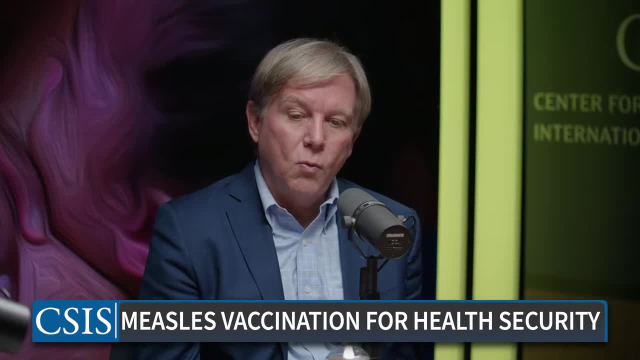 since then, There have been a number of hypotheses as to why the numbers were so low in 2020.. I sometimes think that maybe that was the time to eradicate measles, But it was, you know, some of it. some speculate that perhaps there was just greater immunity. 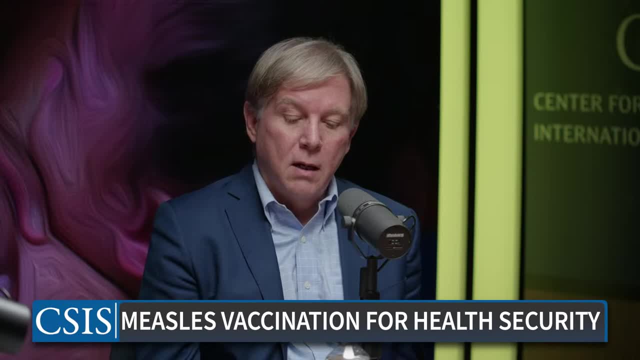 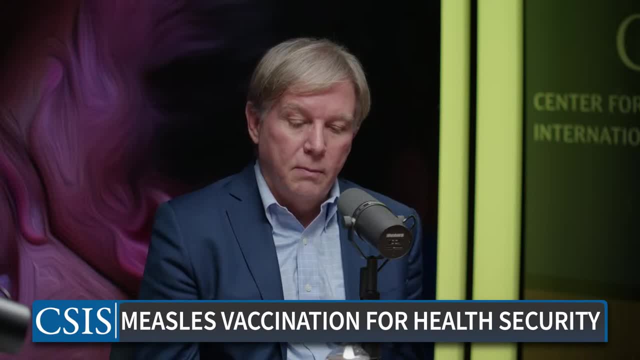 you, as you, as you suggested that you know the, the, the restrictions that were put in place, the masking that all the efforts that we went into to reduce the transmission of SARSCoV-2 had an impact on all respiratory viruses and measles of virus in particular. 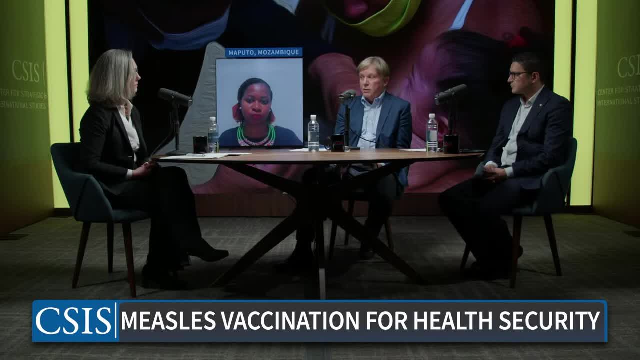 And the COVID-19 pandemic impacted vaccination services on the supply side, on the demand side, And so we ended up with more unvaccinated children. And so we, we, why, why, why, the why, theRIS cosa ーャ? Privacy is always why, why, why, why we're still in the House. 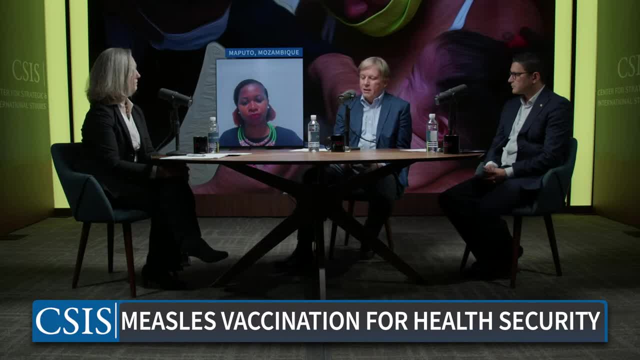 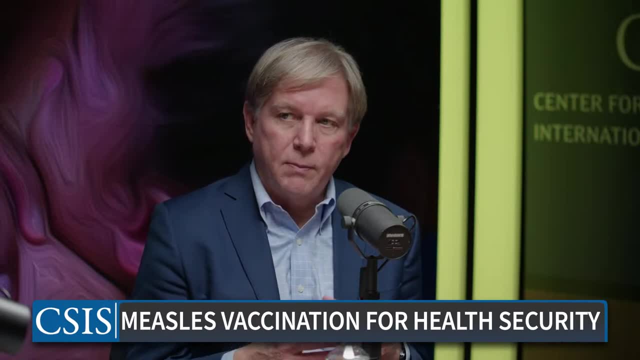 It didn't happen in your country. What we're seeing is kind of coming out of this, coming out of the COVID-19 pandemic: more susceptible individuals, more susceptible children And once the virus starts spreading globally and gets imported into those communities. 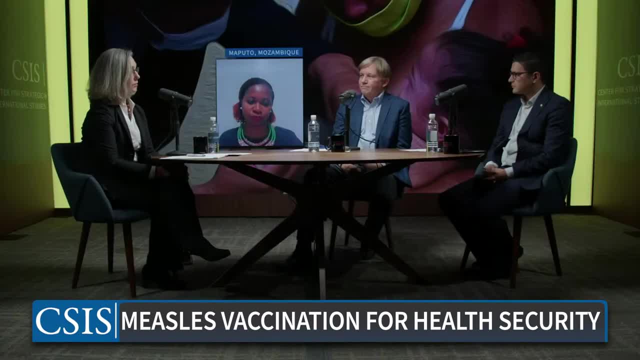 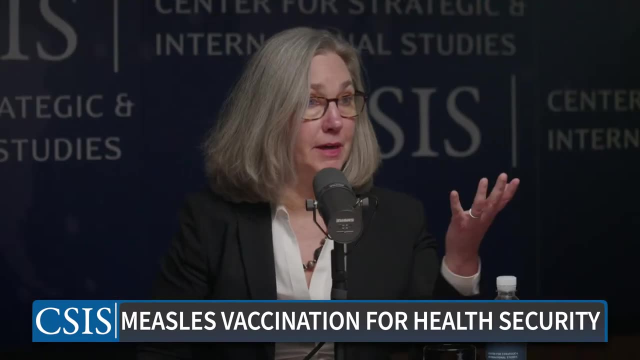 then we get outbreaks. So, thinking about what's happened, we saw this uptick in 2018, and then this global outbreak in 2019.. Danielle, you're looking at the region of the Americas kind of as a whole, and the Americas had kind of been declared eliminated. 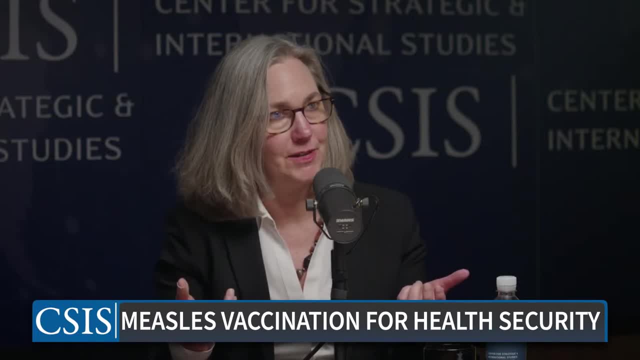 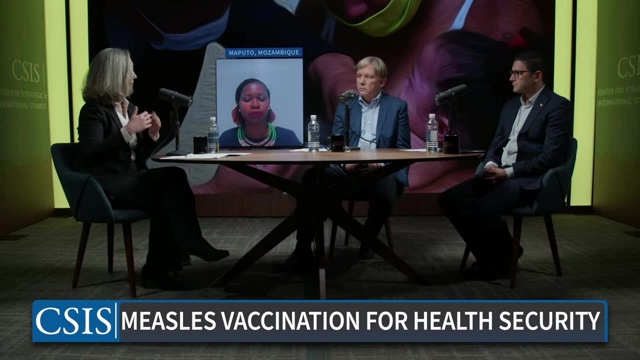 or that measles had been eliminated in 2016,. I think it was right. But then you did see a number of cases in 2018 and 2019, although I think things have been a little bit calmer in the period since the pandemic. 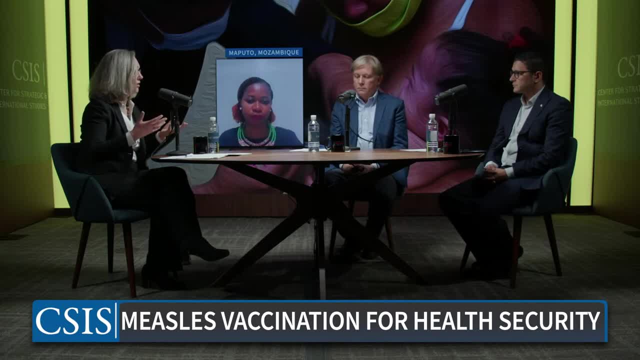 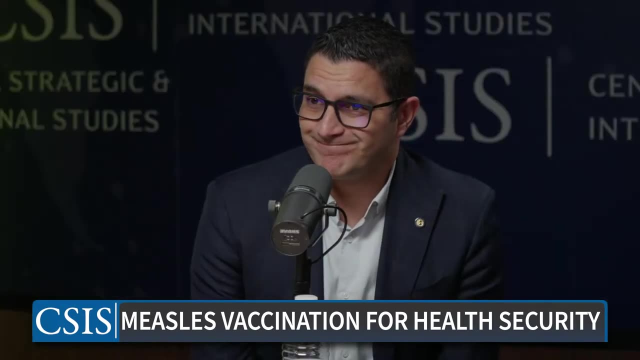 What do you see kind of shaping the current outlook in the region of the Americas and what are you most concerned about as we kind of look ahead? Well, I think, as Bill mentioned, as long as we have susceptibles, and I mean that's going to be part of the scenario. 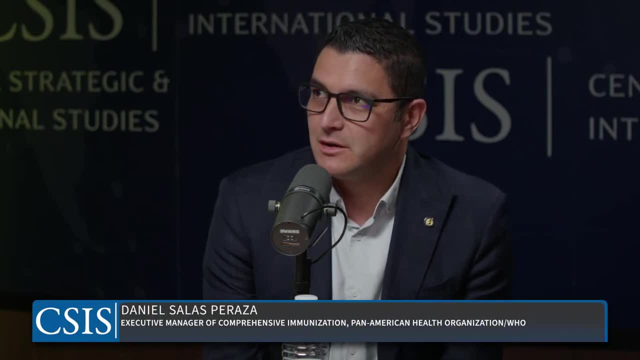 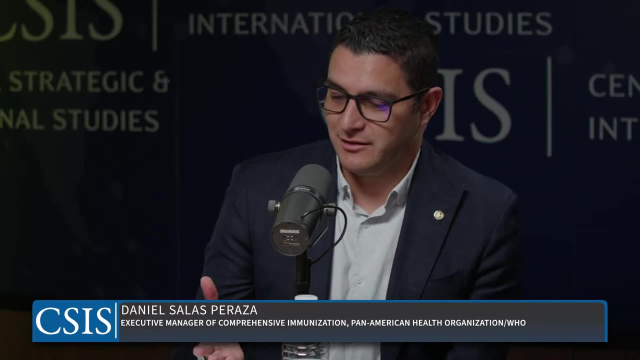 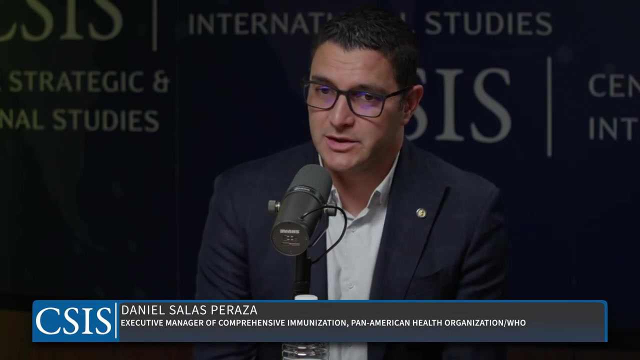 it's probably impossible to not have susceptibles. But the problem is, when you have that 15% that you are leaving behind and that percentage, that percentage accumulates and then you have, like you know, the perfect number to have large outbreaks. 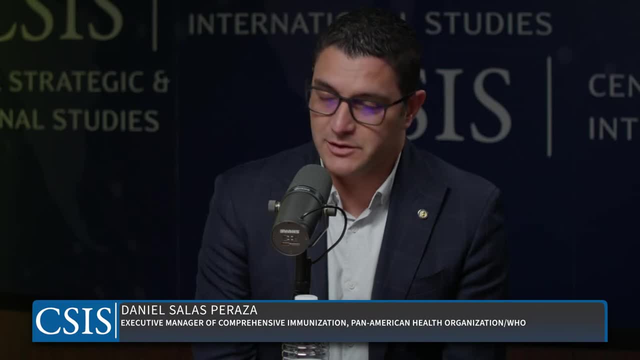 And in the Americas, as you mentioned, we were getting close to the 10 years of not having or having been declared free of the transmission of measles, But unfortunately, in 2019, we had a large outbreak in Brazil and in Venezuela. 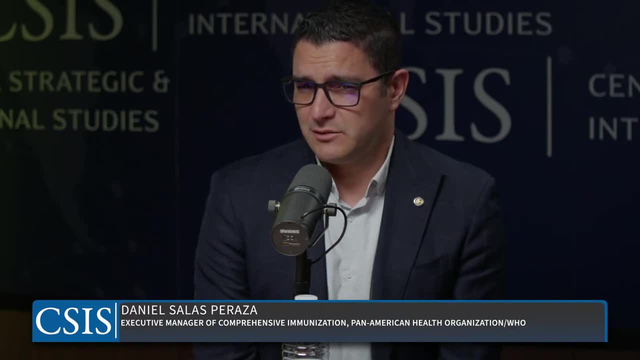 And even we had like in 2019, I think it was like 87 deaths For measles in the continent And of course it required a lot of effort, you know, from those countries to really get the conditions to neutralize the transmission of measles. 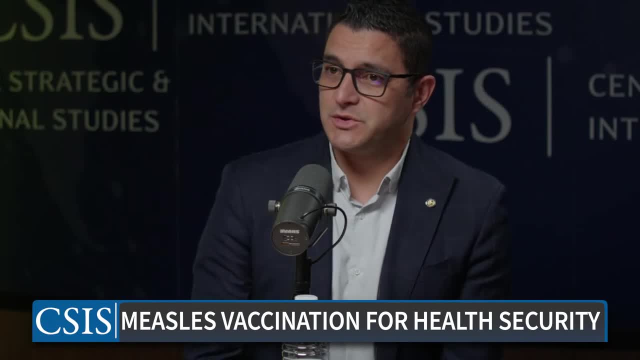 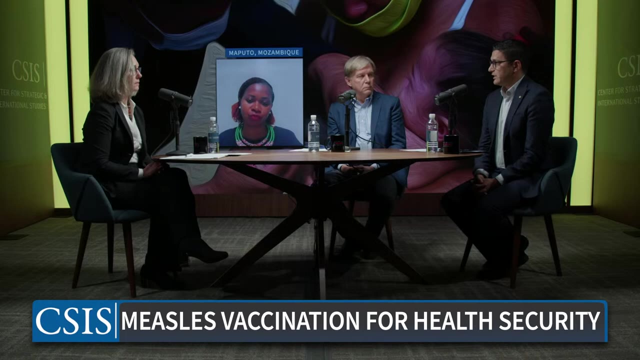 And the last year we have RVC, which is the commission, the regional commission, that certifies, or, you know, review the verification or re-verification of the elimination of the transmission, The transmission of measles in a country, And Venezuela got the re-verification. 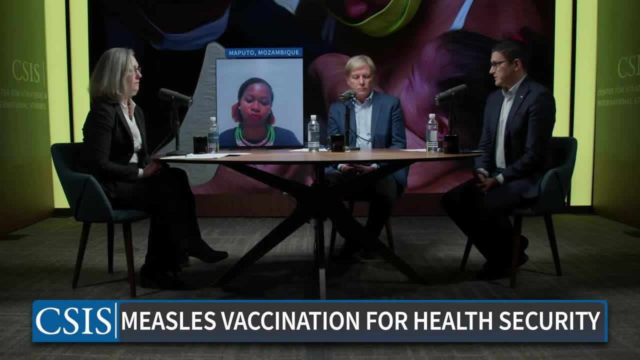 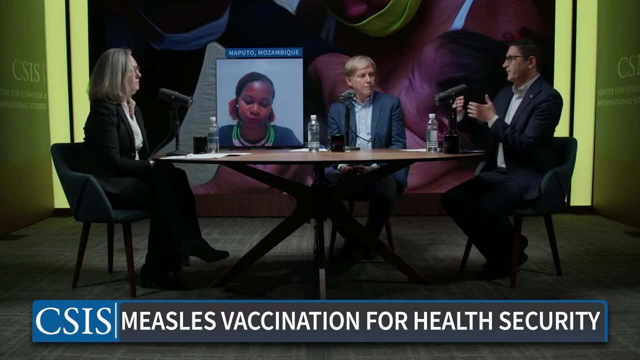 after losing that condition And Brazil is pending, but Brazil has made important steps forward to reach that condition of re-verification. And of course we have importations, isolated cases that they block. I mean they find a block, a wall. 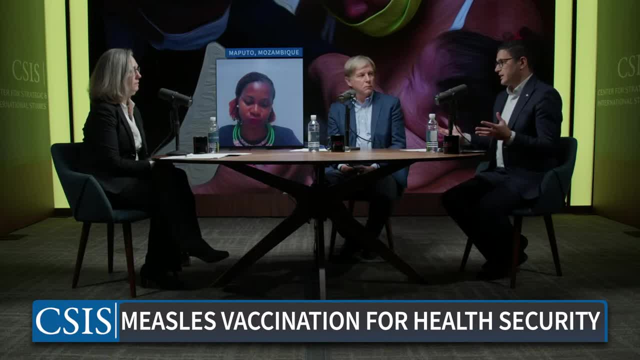 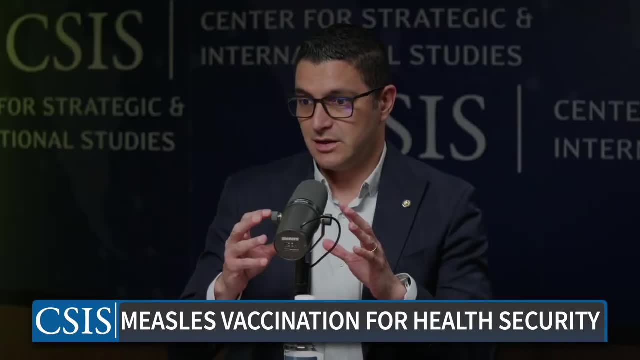 that don't allow them to really spread. Of course, the surveillance: they have a timely, you know, detection of those cases, an acute system that can really identify the cases, And then we proceed with all the epidemiological help, aid or support for those countries. 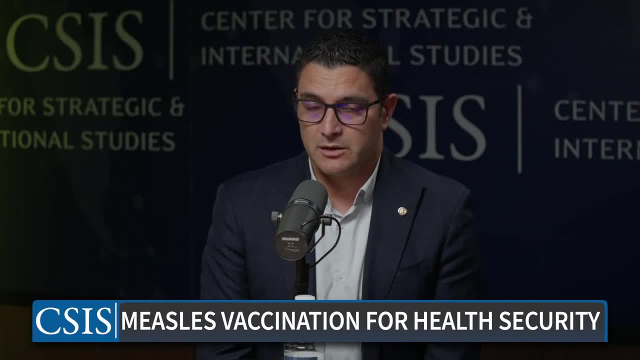 to neutralize the situation. That's very important as well. And of course, the laboratory, because we have a lot of arboviruses here And we know, for example, for the acute test, that we have the IgM. that can be a false positive, if sometimes it is, you know. 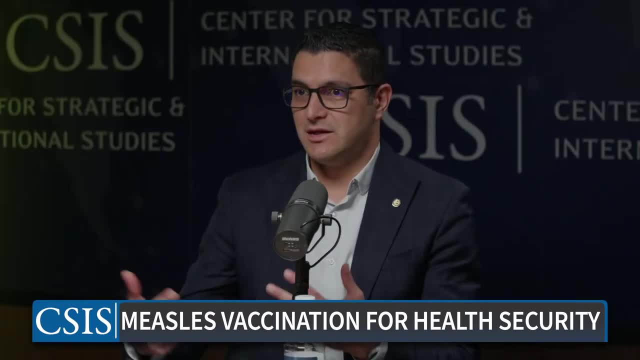 it's a false positive. It can be like another disease, dengue or something different, But that's something that requires training, constant training. That's something that requires a lot of- you know- support to. we have framework of verification. 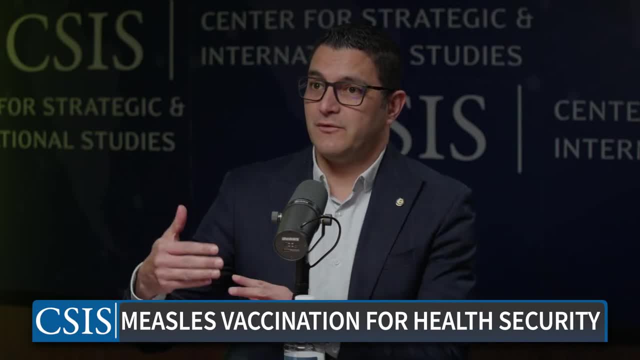 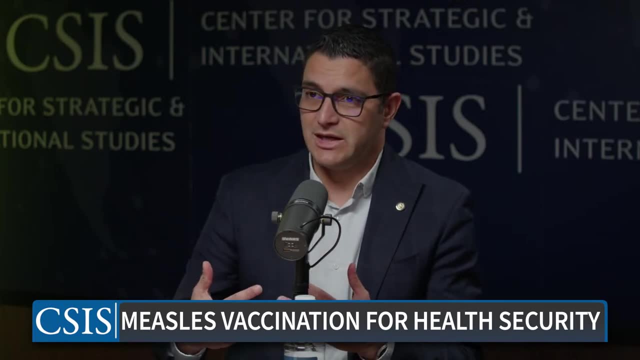 of the elimination of measles And that framework has helped a lot. And we have counterparts for this regional commission in the countries national commissions And they work very intensely on trying to get the report. Every single year we have several meetings re-reporting. 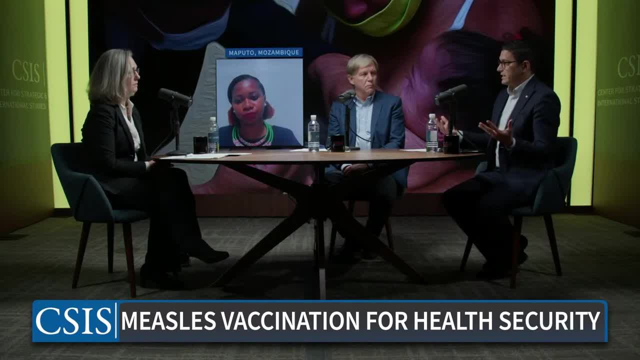 We're the countries exposed, their conditions, what is lacking, what is leaving behind. And this regional commission is very important to have that condition of re-verification. It is. and of course we have the regional tech, the technical advisory group. 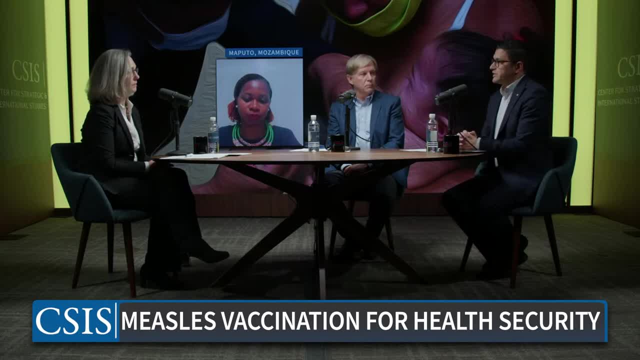 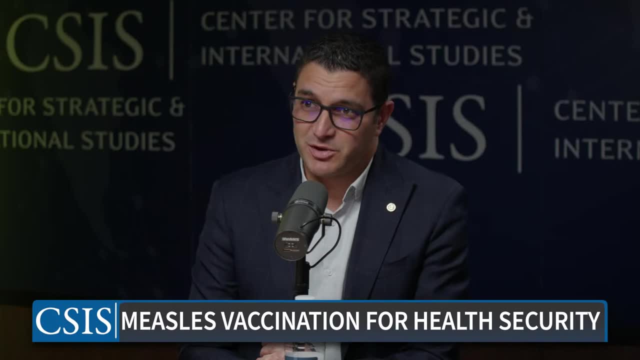 which is always encouraging. countries, to you know, proceed with the strengthening of the programs, the regular programs, And we conduct here follow-up campaigns which probably they are not like the ideal situation, But we- since 2021, we have been implementing. 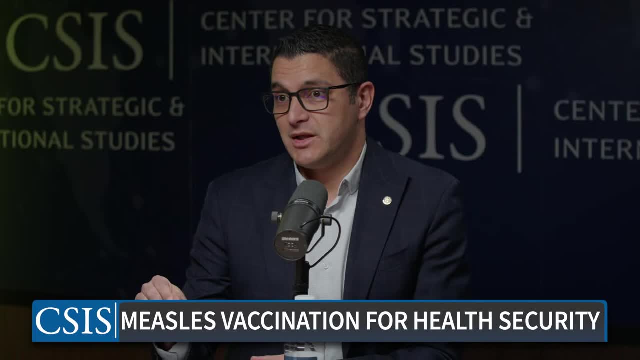 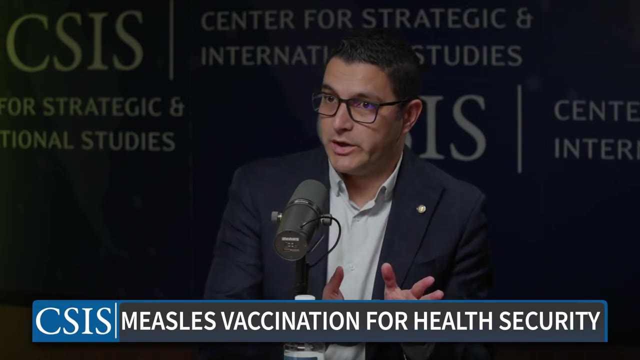 at a high quality follow-up campaigns methodology to really try to identify which are the ones that are not vaccinated, And even to vaccinate those children during the vaccination campaigns and add those children to the regular coverage reports so that we can really know what is happening. 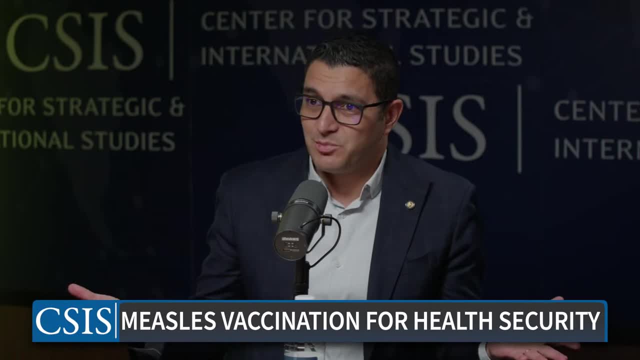 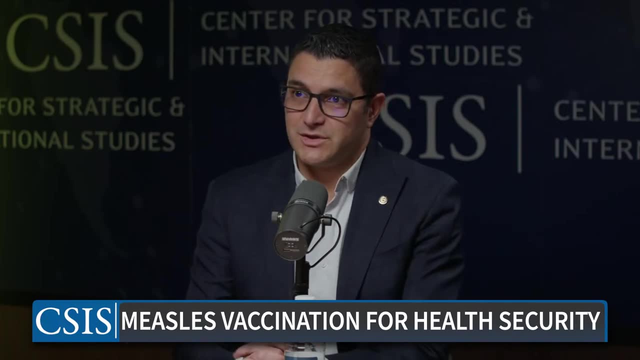 Because before that date the problem is: you conduct a campaign, you conducted a campaign and you vaccinated, And the ones that have been already vaccinated? of course, that's not effective, So we have been migrating to this high quality methodology. that is, of course, much better. 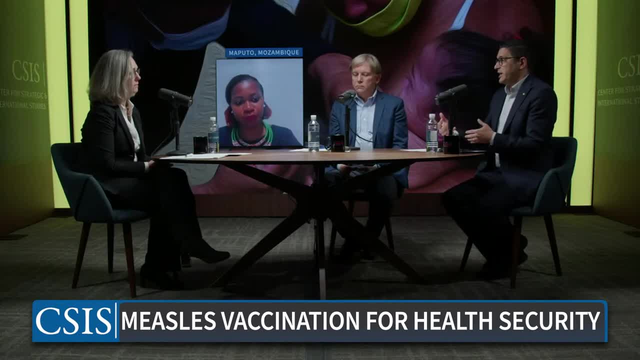 And that's what we have. I mean, it's impossible to not conduct a campaign when you don't see that you're reaching 90 or 95% of coverage for both doses of MMR. So, Graca, I'll look at you here. 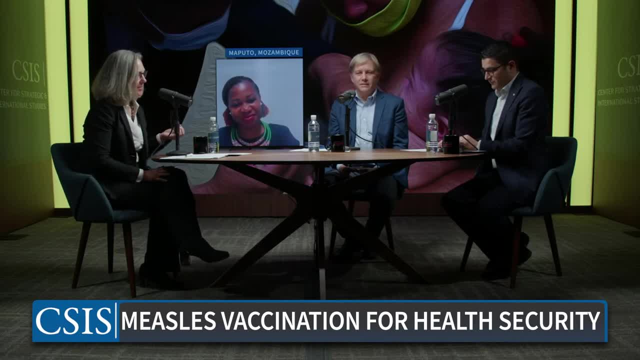 Thank you for joining us from Mozambique. So both Bill and Danielle have really, you know, pointed to the importance of, you know, really reaching this last, you know, 15% that has been, you know, missed, at least at the global level, you know. 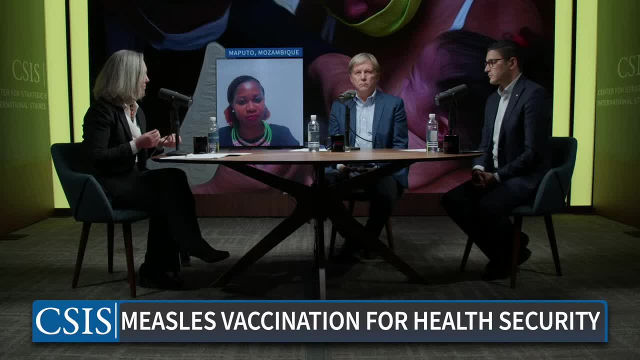 in terms of access to measles vaccine, But also just the real importance of micro planning and really understanding where the children who are missing out on these doses are. You're with the MRIGHT program in Mozambique And really you know, focusing on issues around equity and access to immunizations. 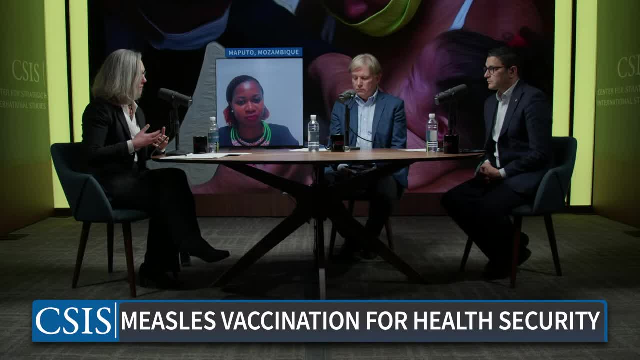 So could you say you know a little bit about. you know some of the what you're seeing in terms of reaching those zero dose and under immunized children with measles vaccine and kind of where you see the trends at the current moment. 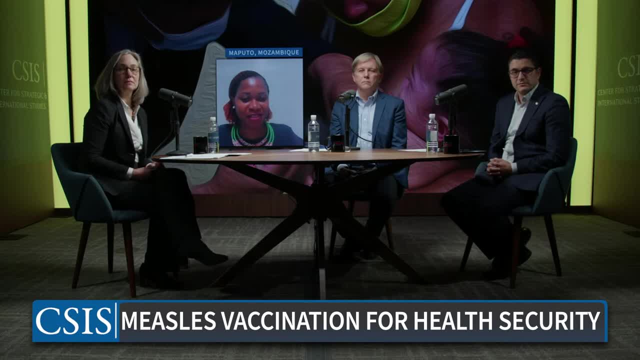 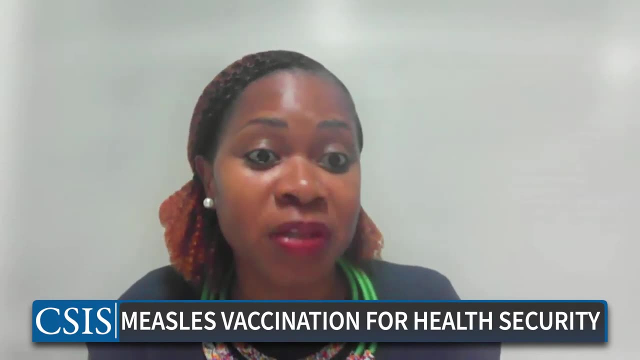 Thank you, Catherine. It's a pleasure being here and discussing this very important topic. Let me put you a bit in context of what is happening in general in the African region. You all know that measles is one of the leading causes of infant mortality, and this is still real in our context. 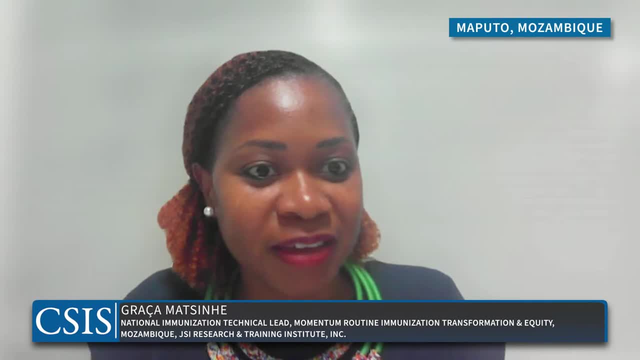 And different from the America, where the and other countries where the elimination goal was met. we had a very ambitious 2020 goal for eliminating measles, which was not met, And we see a scenario in which the coverage of measles has been decreasing from 2017. 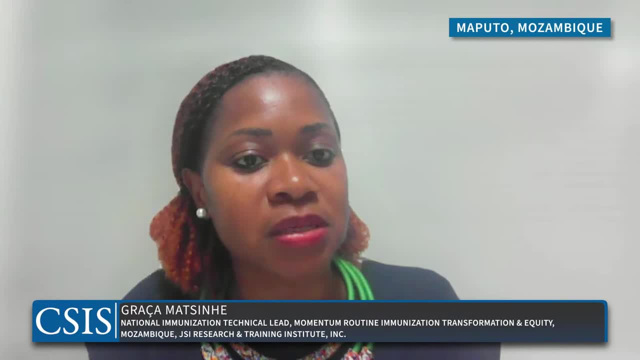 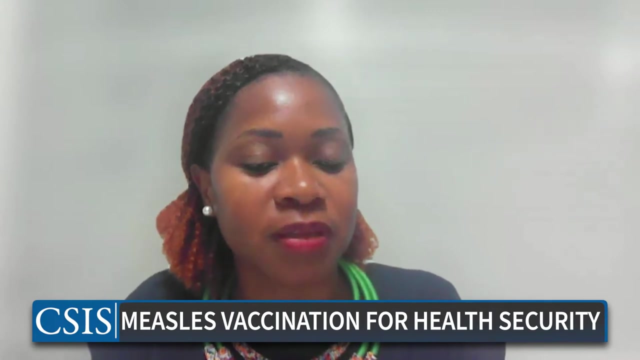 to 2021, there's a very big difference, not only in coverage- vaccination coverage- but also in surveillance. The indicators of surveillance have not been met by several countries in Africa, So definitely we have here a very fertile situation to have these outbreaks arising in different countries. 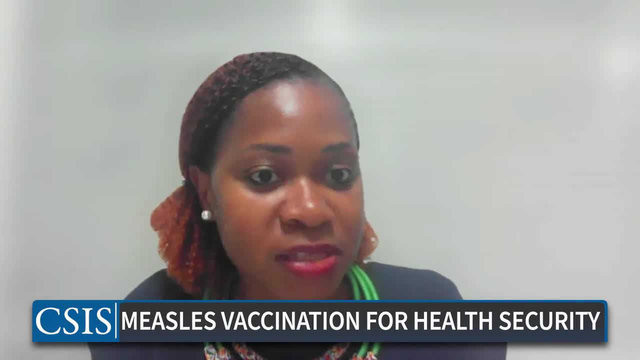 And we have seen an unprecedented outbreak in South Africa, for example, Which has been a country with very high coverages of immunization, and many, many other countries in Africa. So this is really, really challenging, especially when we look at the coverages that have been stagnating. 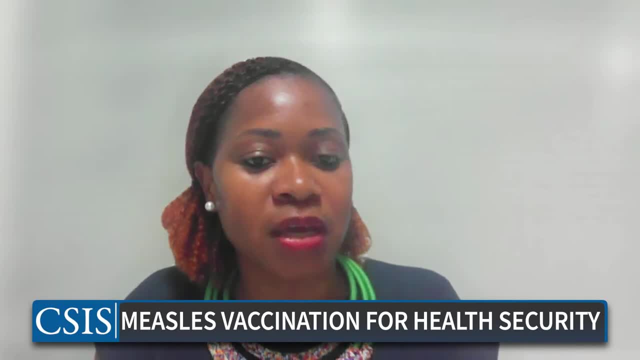 As Bill mentioned also, we see this situation here. The coverages have been stagnating for many years, Not only the MCV coverage but other vaccination antigens. But we also have one additional challenge is that, although many countries have been implementing- 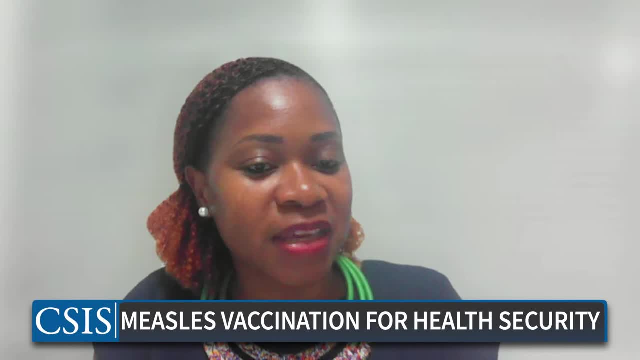 I think supplemental vaccination activities. the implementation is still suboptimal, So this obviously will create a lot of susceptibles And we know that this is the perfect condition for us to have outbreaks. In the African context, there are some particularities. 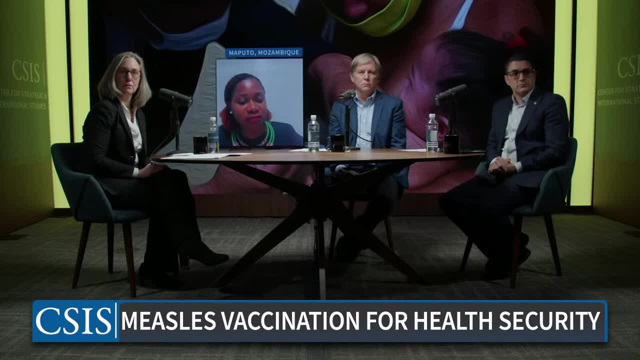 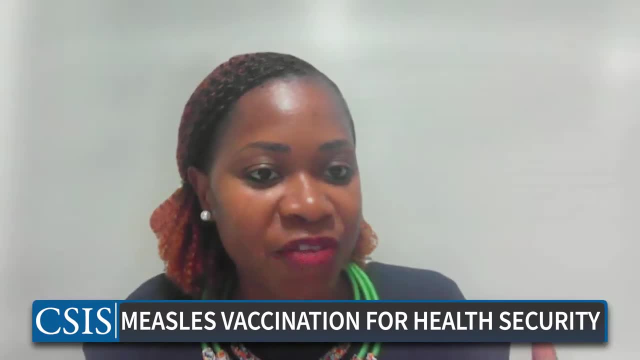 that I would like to mention, because I believe that this is very different in other regions And this particularities will affect directly the functioning of the immunization programs, the immunization programs and also the campaigns. I'm talking here about inequality of access of health services. 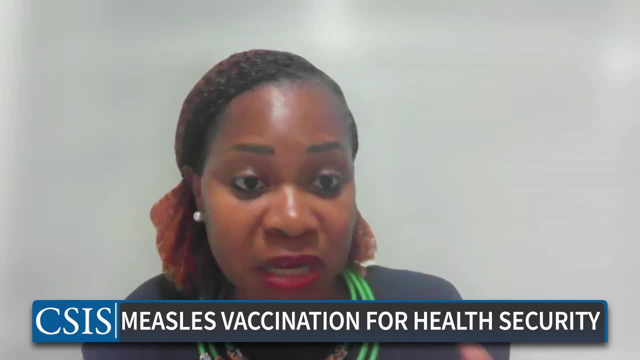 because the health facilities network is very poor in many, many settings. I'm talking about the low confidence of vaccines among the population. I'm also talking about the health system barriers which have been affecting a lot: The, the, the you know the you know the, the, the, the you know. 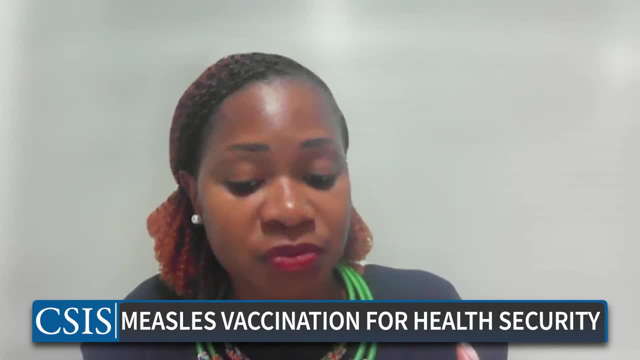 the uptake of immunization services in different settings. But also we have other particularities like the wars, conflicts in different parts of Africa, And we know that with conflicts the health systems will have a rupture in service provision. So here we also have a big issue with achieving coverages. 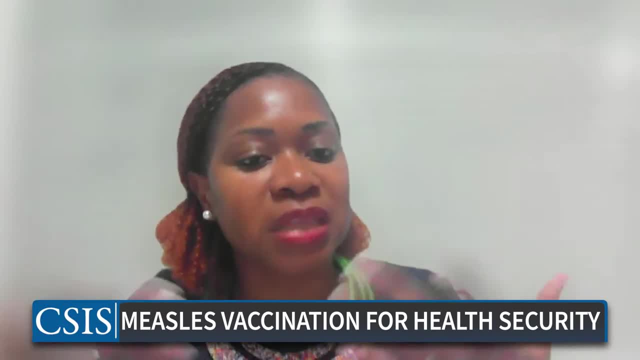 and making sure that children are getting vaccinated. So those are some of the things that come to my mind when we're talking about reaching children with measles vaccination. The context is very, very complex And we need to work together in order to make sure. 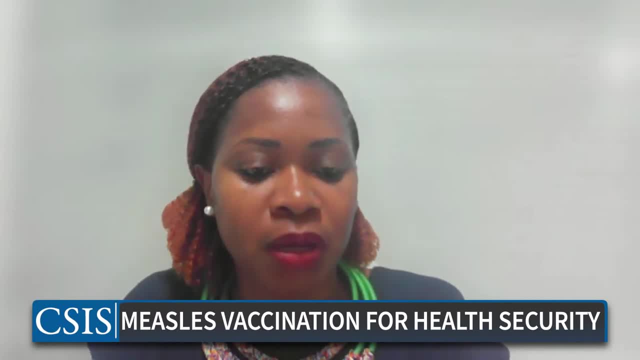 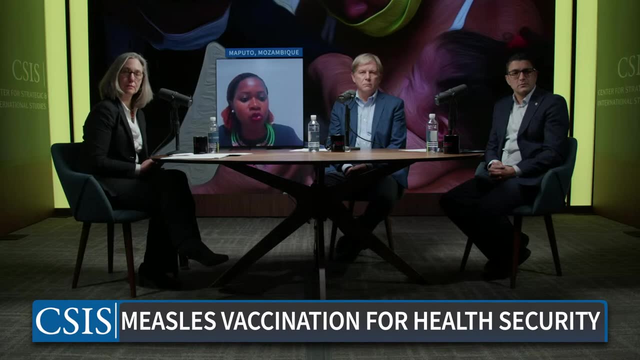 that these situations are overcome, Looking at how to better reach children. in this context, obviously good micro-planning is necessary And all efforts, be it by government and private sector partners operating immunization, are towards improving the micro-planning processes, starting from the bases. 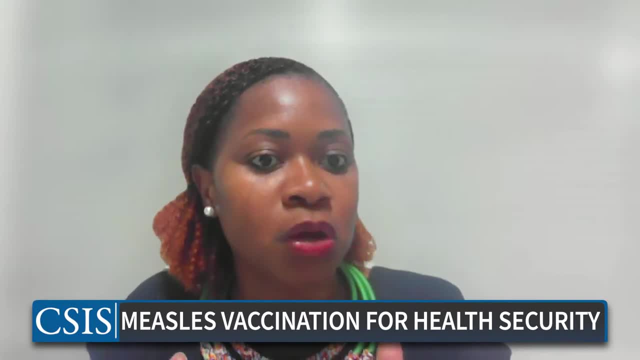 I mean the health facilities, and then the districts, and then the provinces. So having plans that develop bottom-up is crucial, And this is the efforts that we have been making associated with mapping and identifying children in the communities. We're now bringing on innovative strategies. 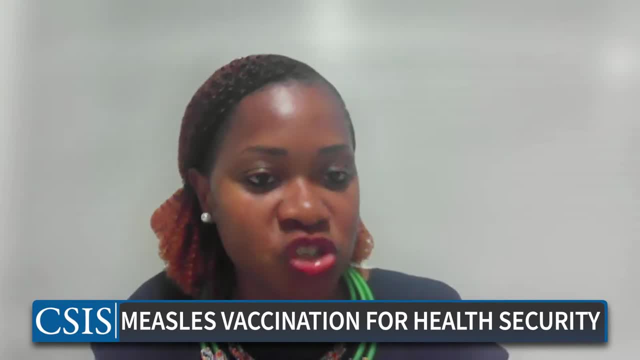 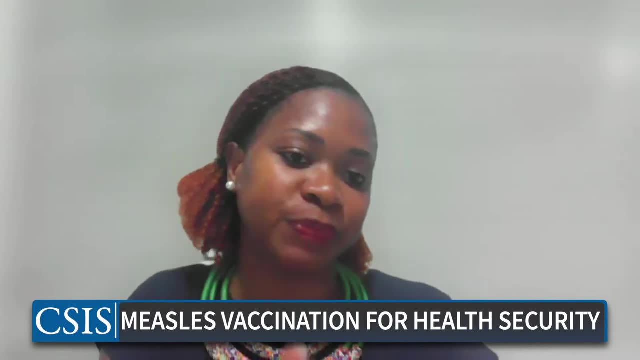 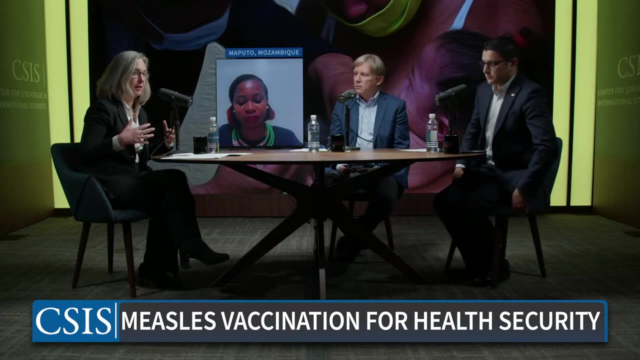 like using the GPS to map and identify those children so that we can know exactly where these children are And then it's much easier to reach those children when we go to the community. So several of you have mentioned the importance of really undertaking training for health workers. 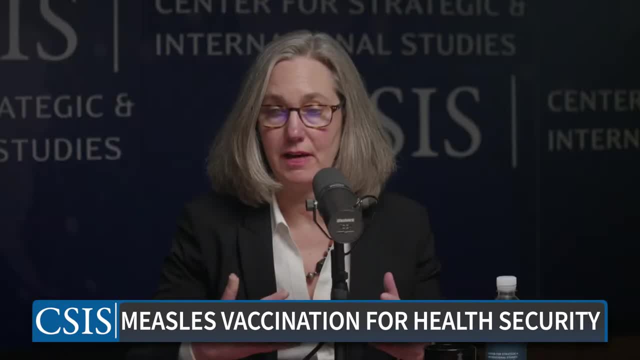 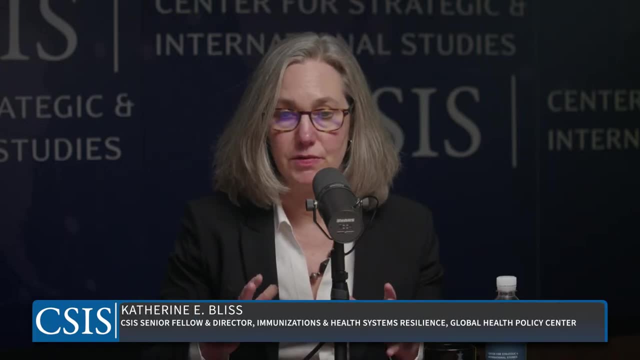 and improving surveillance and detection, as well as really employing GPS and other kinds of things, And we're also working on a lot of new technologies in order to really identify where children who are missing vaccines can be located. But one of the challenges, certainly, that we heard- 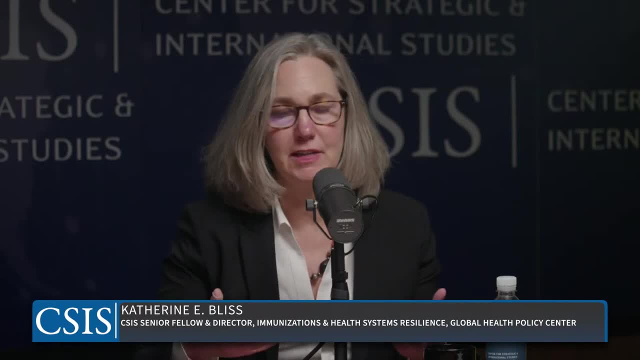 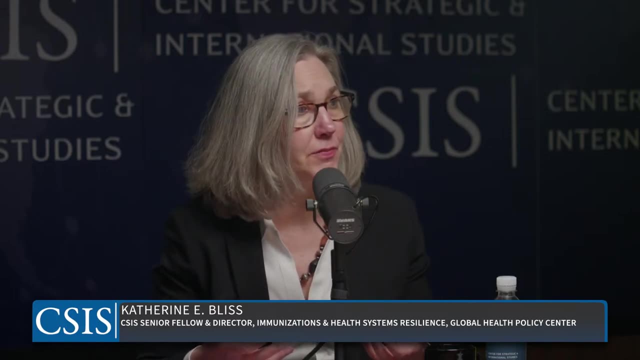 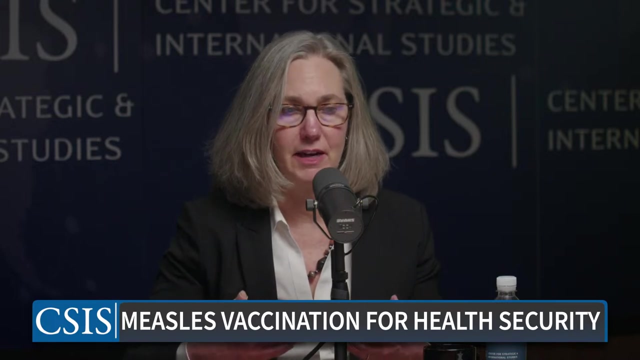 talked about a lot during the pandemic with respect to COVID-19 vaccines was that the health system was in areas where the health system itself was fairly fragile. It was difficult to reach out to communities to really establish those connections, to find ways to build that dialogue. 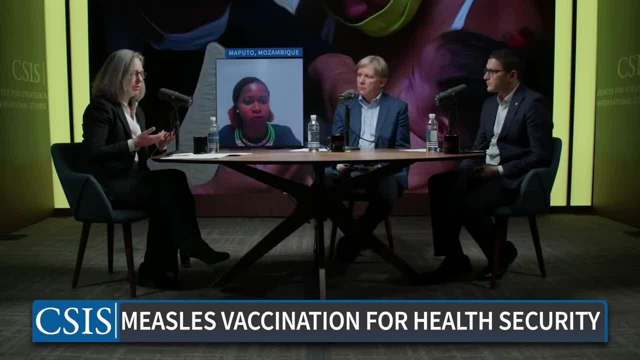 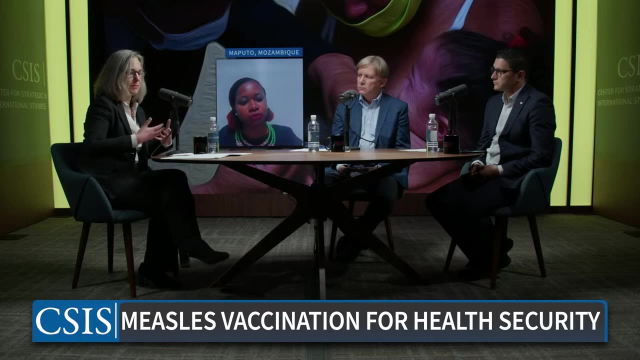 and reach the families in need. So maybe I would go back and start with you just to ask you to say a little bit more about the steps that you see need to be taken to really ensure that the health system as a whole is able to more effectively deliver vaccines. 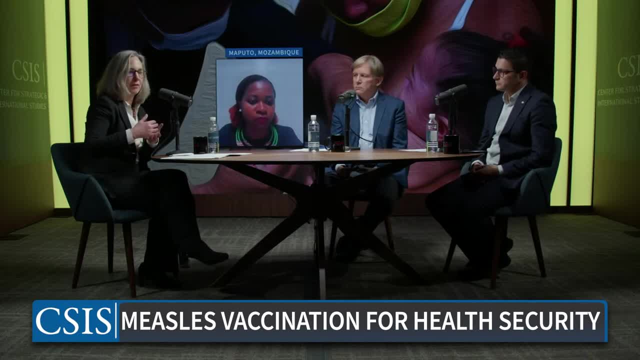 Is it better training for health workers or is it- I mean, you mentioned some of the issues around building confidence at the community level- What steps can really be taken to prepare the health system to deliver vaccines through routine programs before we even get to kind of needing? 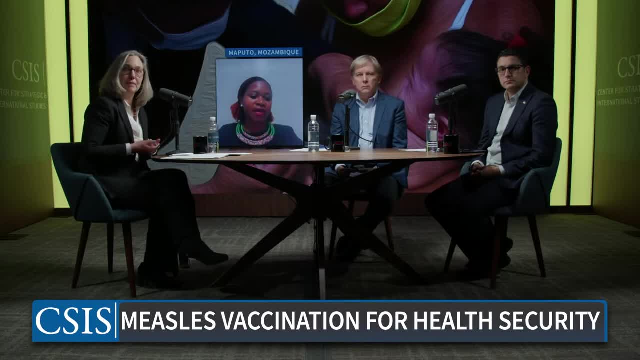 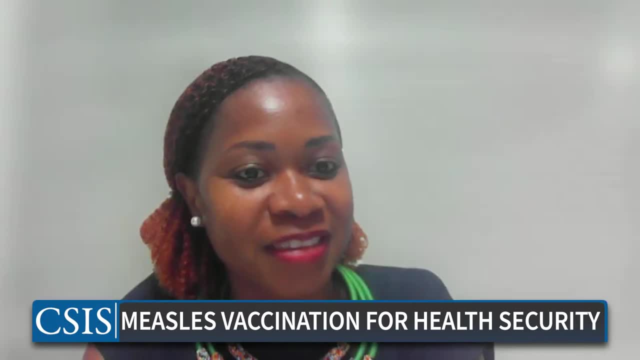 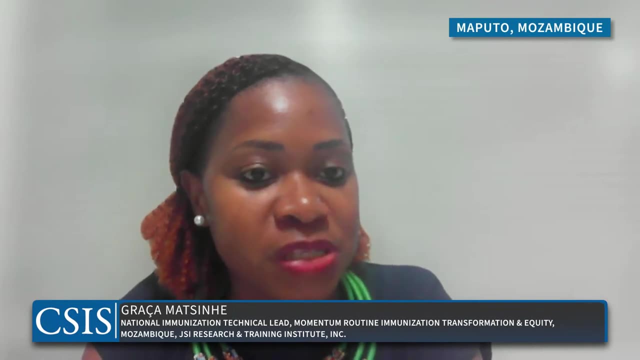 to deliver through campaigns? Yes, well, definitely. the COVID pandemic unveiled health system fragilities in the different contexts of the world, Be it in Africa, in America, everywhere the health systems were severely affected by the pandemic. But this also gives us an opportunity. 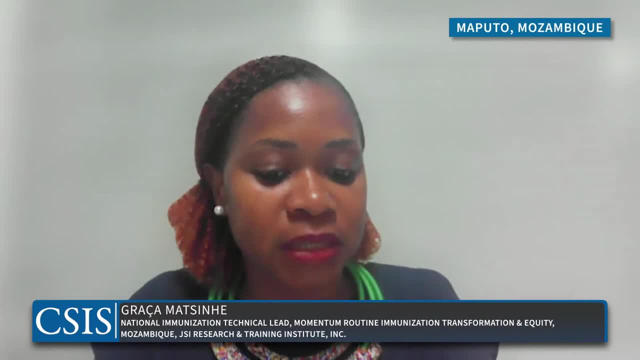 to build more resilient health systems, And we need health systems that will effectively respond to the need of the community. because we're working for the community, Everything that we do is for the good of the community, which is us, at the end of the day. 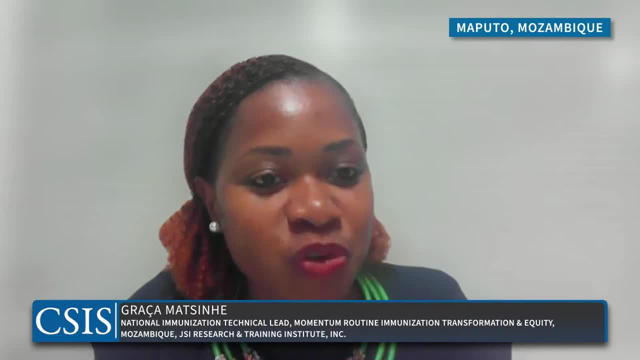 So, in my view, to have a very robust, robust routine immunizations that are able to deliver not only measles vaccination but all the routine immunization antigens, we need first to invest in human capital. Here I mean allocating the human resources. 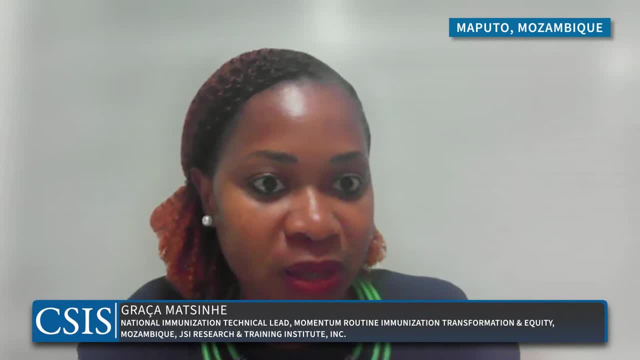 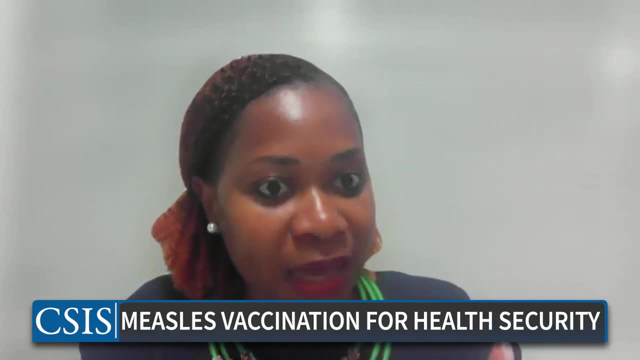 to the places where they're needed the most. I'm talking about the hard to reach areas, which usually tend to be the less served areas, So we need to make sure that we have the adequate a cadre of human resources to provide good quality immunization services. 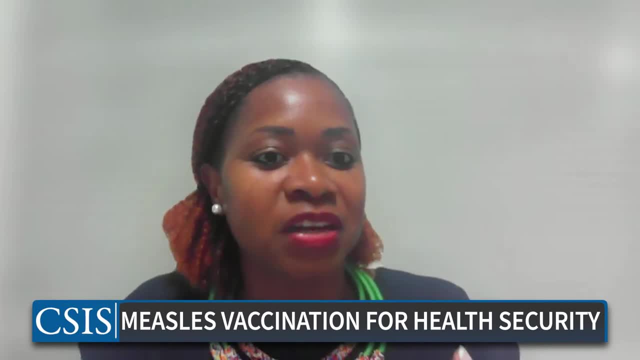 But also the ones that are already there. they need regular training, be it in the form of on the job training or mentorship programs, but we need to keep training the human resources to better provide immunization services. The other thing that comes to my mind: 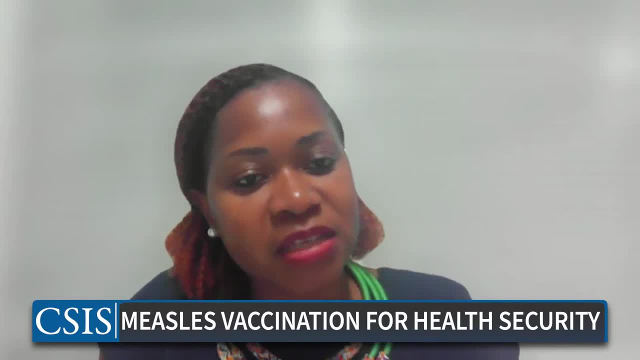 is the need of minimizing the health systems barriers, Because when we talk about barriers, most of the times we look at the distance, but there are so many barriers, many barriers inside the health facilities, which increases the missed opportunities of vaccination And most of the opportunities. 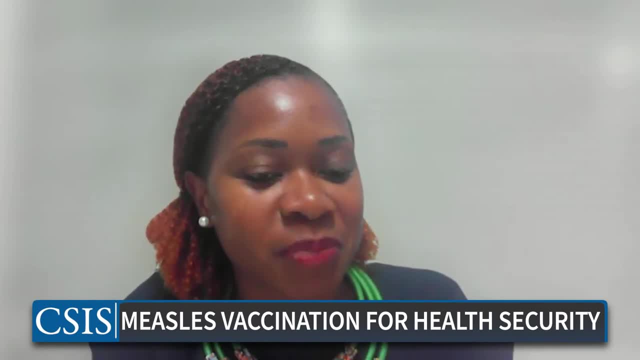 they are related to the health workers, the behaviors. So we need to minimize those barriers. We need to communicate better with the people who are seeking health services, the health facility, so that we can effectively provide good quality immunization services. The other thing that I think is fundamental: 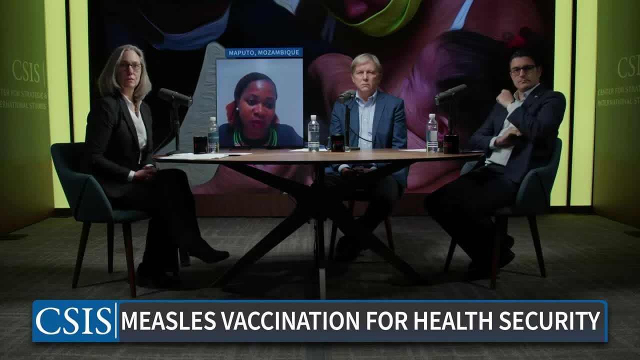 is to ensure the availability not only of vaccines but other consumables, including the cold chain. So those are the things that we need in order to have very strong routine immunization services and be able to deliver measles vaccination in good quality. Obviously, it's not limited for those ones. 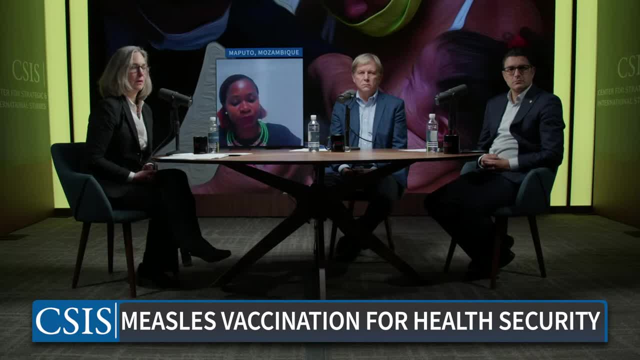 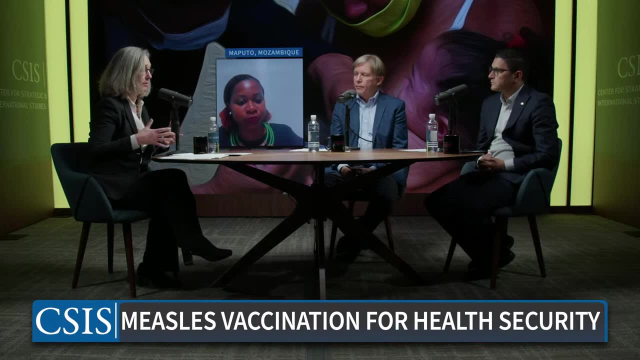 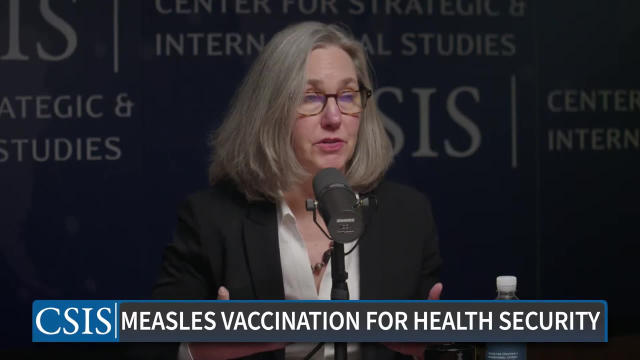 but I think those are the most important issues that we need to work on. Thank you, Daniela. I know that in the Americas PAHO has really placed an important priority on kind of rooting well building the capacity throughout the region. 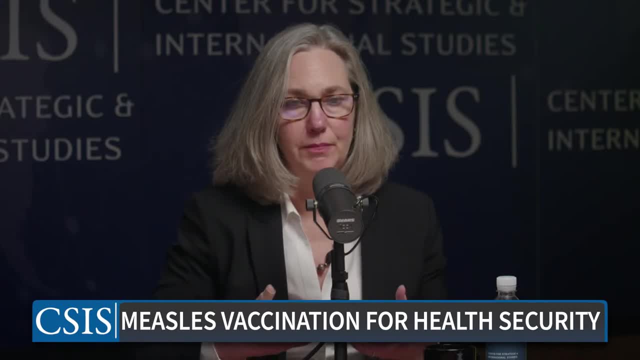 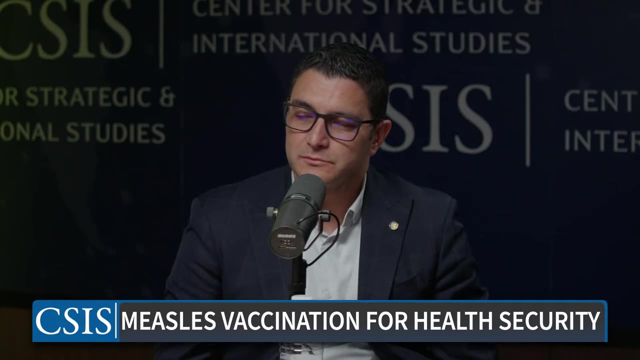 to deliver primary healthcare and really rooting services in that kind of model. I wonder if you could say a little bit about some of the efforts throughout the region. I know you have experience in Costa Rica with the ministry as well and with the primary healthcare model, but you know 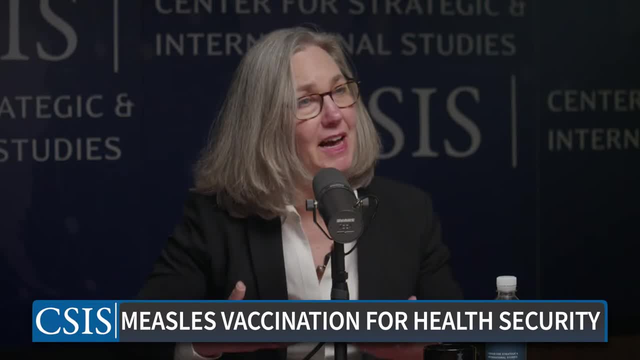 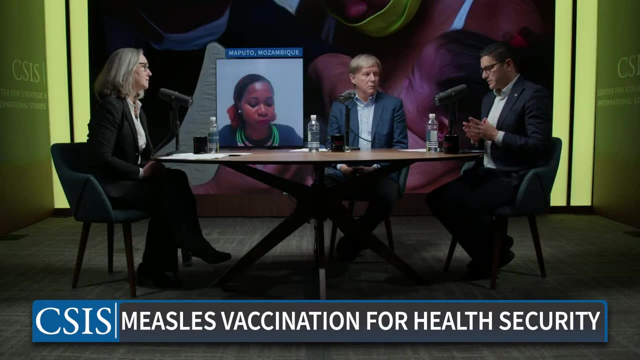 what is. how can strengthening the health system in that context really facilitate delivery of vaccines? Well, I think that it is very important to try to tighten up the relationship with the community and the primary healthcare, because, I mean, that's the essence of the primary healthcare. 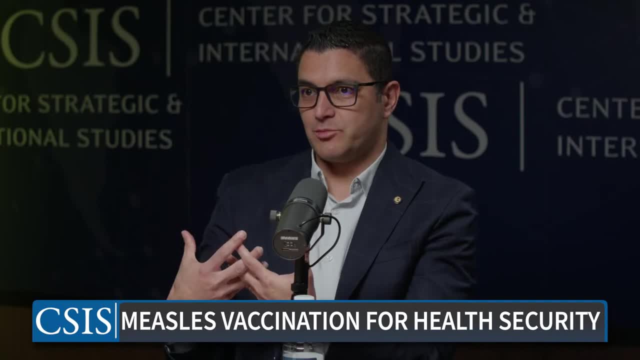 It's to build. you know, like that social participation, that promotion of health, that you can go wherever you go in a community and you can breathe wellness. you know the condition you choose has influenced me, like that social participation, that promotion of health. that you can go wherever you go in a community and you can breathe. you know wellness. you can breathe well this kind of time, or as well as a CAN, if you want to do painkillers, Of course, I mean this, 이 niqi she'n liδry in riders, naturals, which you can do this one as well, and you like to think? 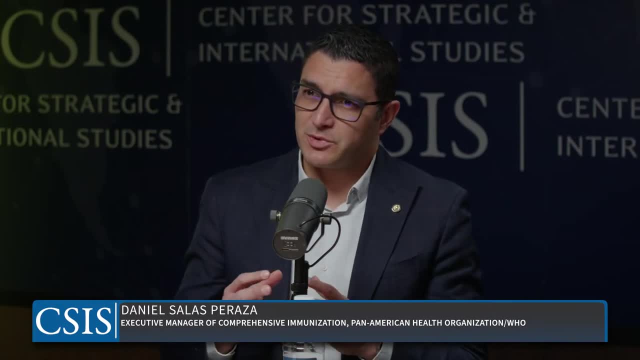 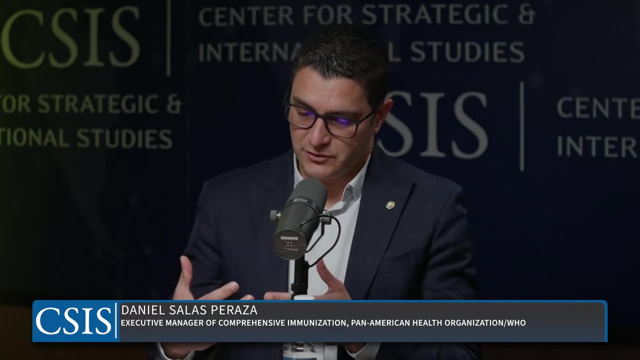 opportunities to improve your health, But that's something that probably is not happening at the level that we would like it to be, So it is very important to work on that, to really try to identify which are the social stakeholders, the partners, the non-governmental organizations. 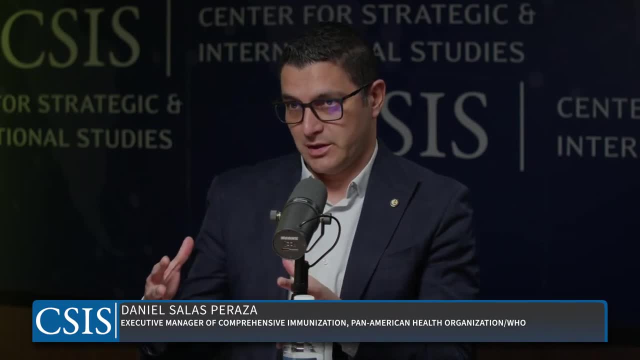 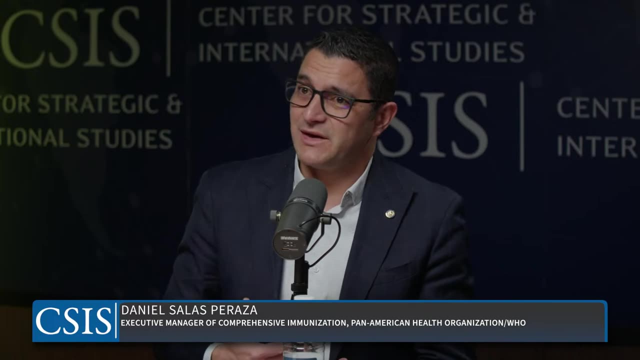 the private sectors that can really build that network to facilitate vaccination, to facilitate, for example, if you have doubts about to get a vaccine or not And if you are waiting to get to the health facility, to the health care facility. probably sometimes that represents a barrier. I 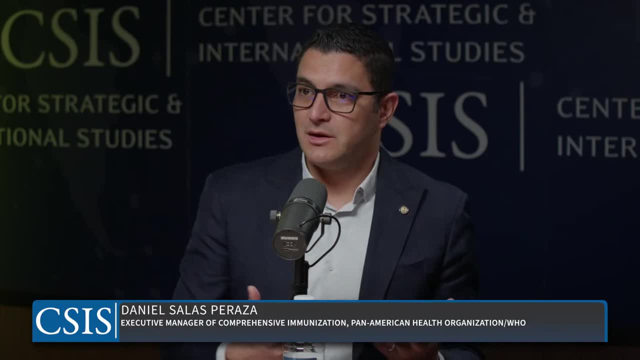 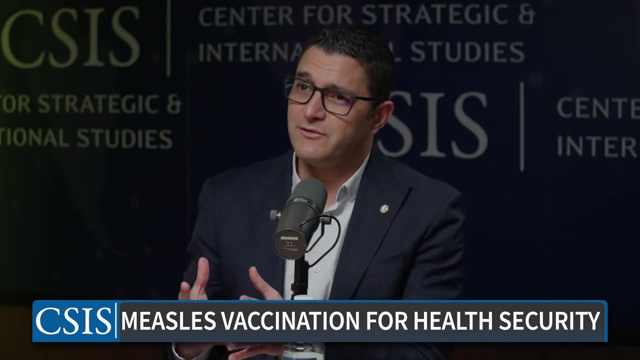 mean something that you have to defeat, But if you go to the local government office or if you go to whatever- I mean to pay a service or whatever- you can find that information easily accessible in words that you can understand. That would be a game changer, But that's something that we need to really continue working on. 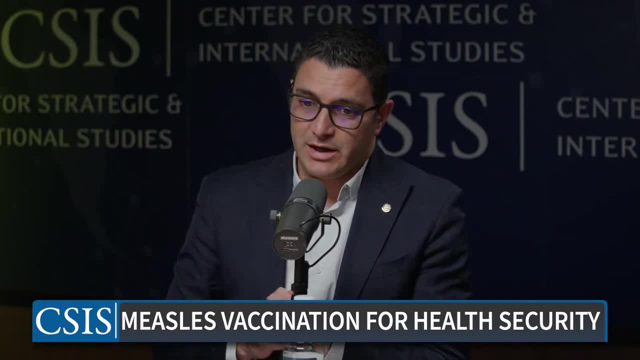 because something, for example, that we have found now is that families have migrated to a different composition And now, for example, both parents work during the daytime and they cannot take their children to the health care service if it is not after 4 pm, when usually the service is. 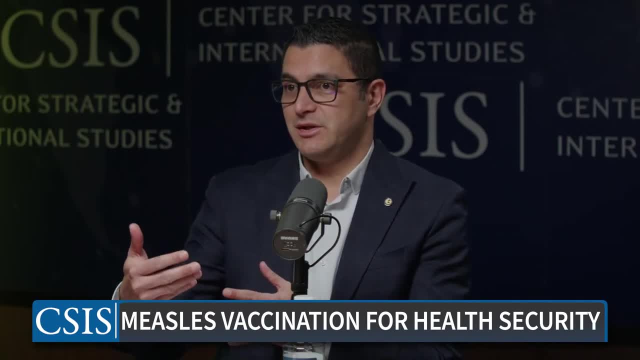 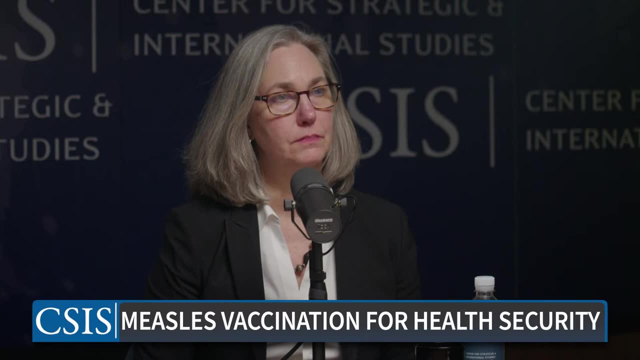 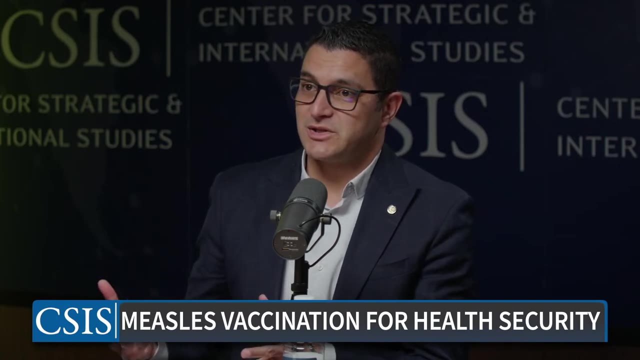 closed. So we have not adapted the possibility for those parents or the single mother or whatever, to really take that children to the you know to be vaccinated, For example with COVID-19,. what happened? We offered the vaccine in malls, in shopping centers, in, you know, in cars. It was a. 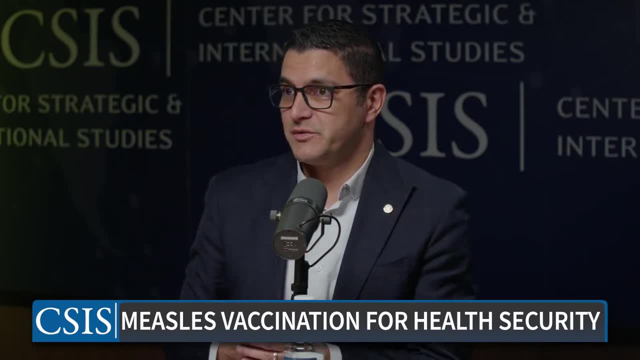 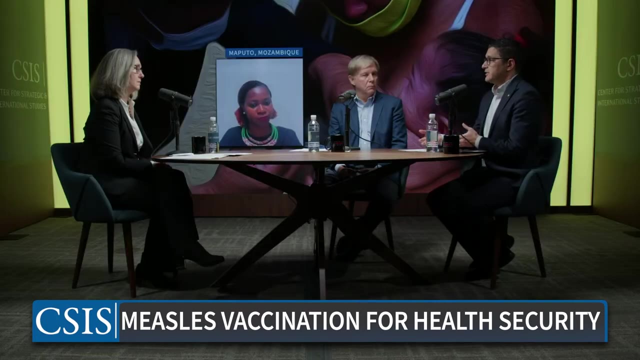 really different modality of vaccination. So we really I think that we really need to stratify the analysis to find out What is happening with that 50% of population that is not receiving their vaccine. It is because they go to the, you know, to the health service and the vaccine is not available. I mean because sometimes 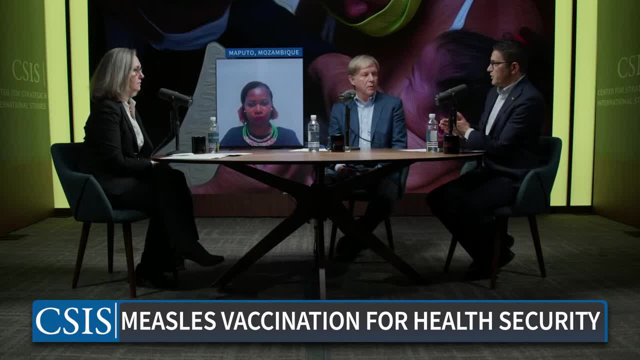 even the vaccination time of availability is just from 7 am to 10 am, And then you get there at noon and then the vaccine is not available anymore, Or simply you cannot go until you know evening or even later. 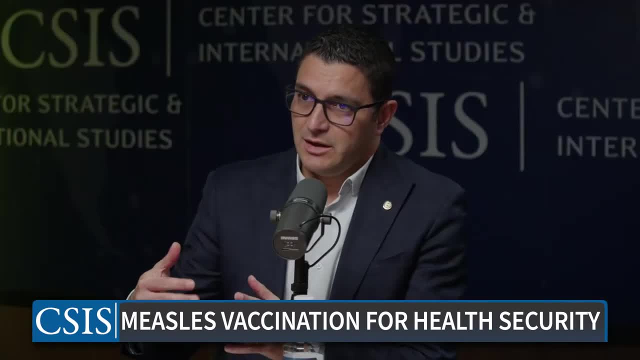 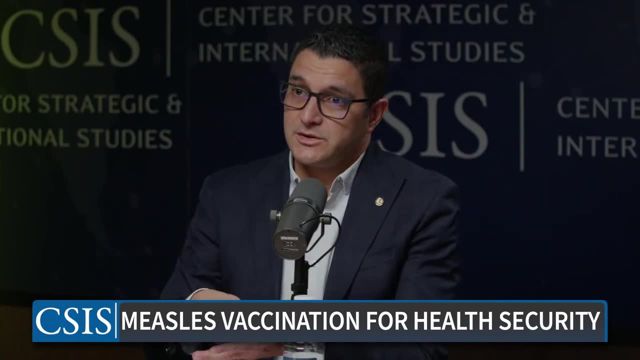 In some countries, for example, we have a lot of people who are not vaccinated. We have a lot of people who are not vaccinated. So, for example, in the Americas they have been experimenting with offering at night or evening, like visiting houses and checking. you know the schedules if. 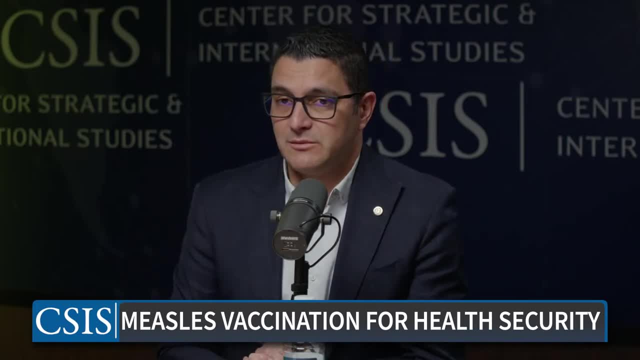 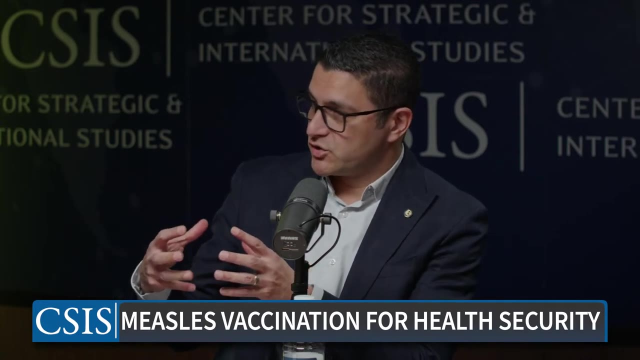 they are complete and vaccinating the ones that they find that are not vaccinated. But I really think that we need to adapt the offer of the primary healthcare and tighten up with older services as well, because it is not just to offer the vaccine alone. We need to really try to integrate. 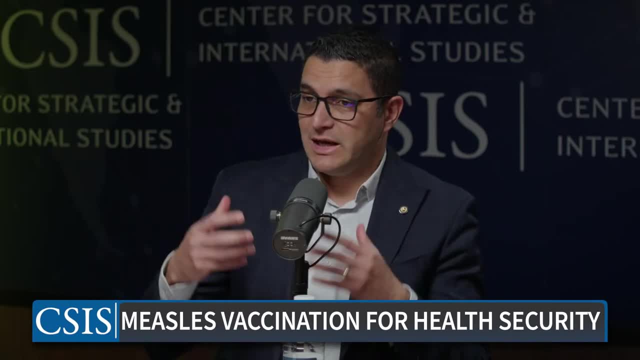 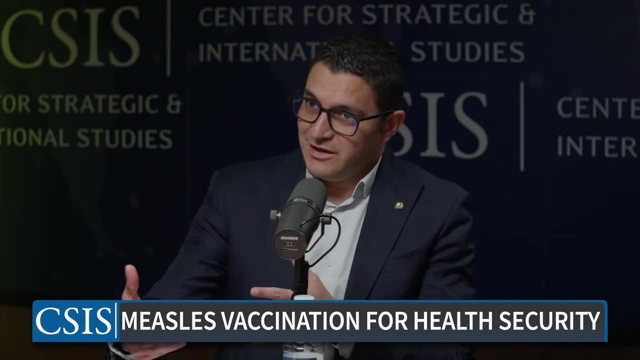 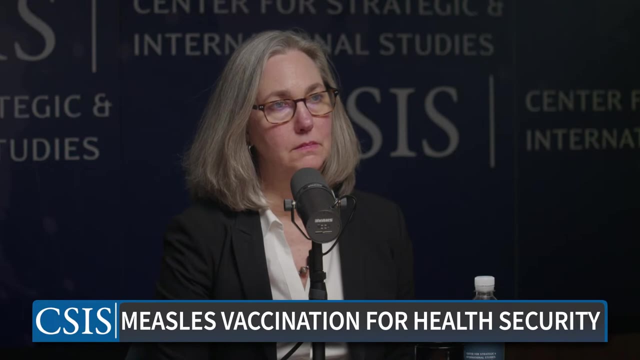 this vaccine alone, offering with other services, and have a course, you know, a life course approach where you can really, you know, get the family to go to the health service even on the weekends, because probably on the weekends we have just the emergency services you know working And 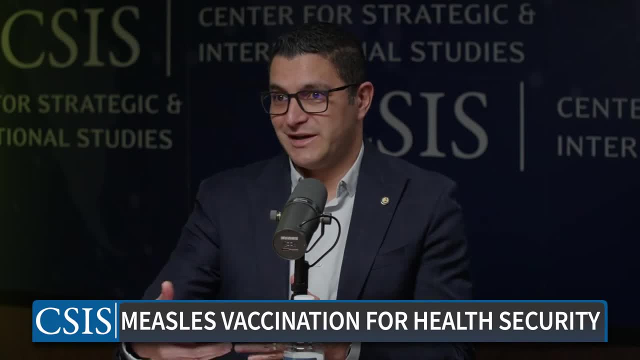 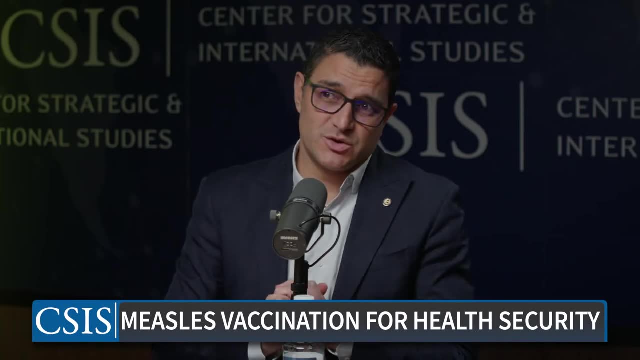 probably that's the time where the families can really go as a whole to, you know, to have like this package of checking their health. So that's something that we need to work on And I know that, of course, primary health care has been like the cornerstone of our services here in the region. 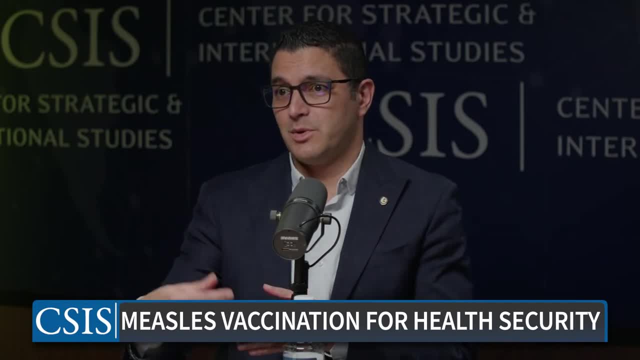 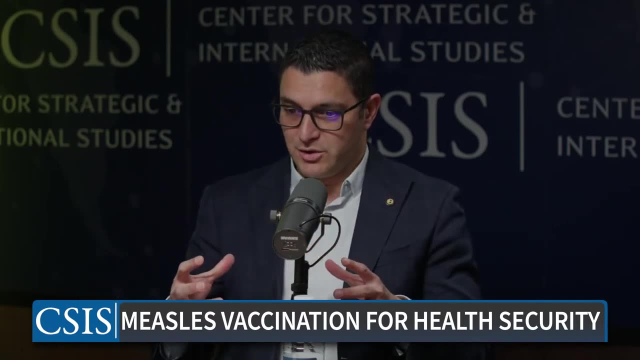 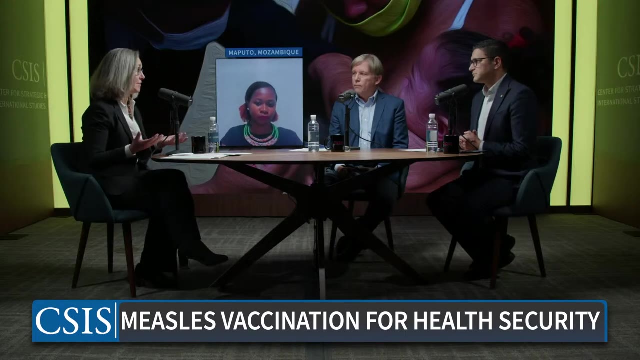 but it is not enough. We really need to go to the next step and to reach this next plateau of bigger integration, of bigger- you know- vision of building the social participation of health in the community. So some of it, you know, really is adapting to the way people live and meeting. 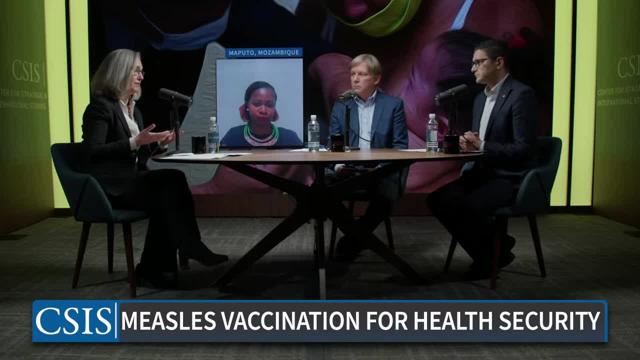 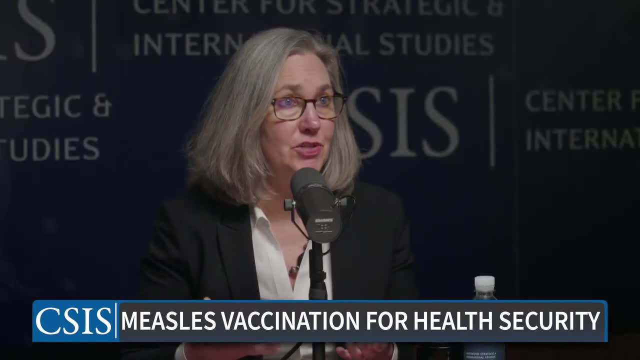 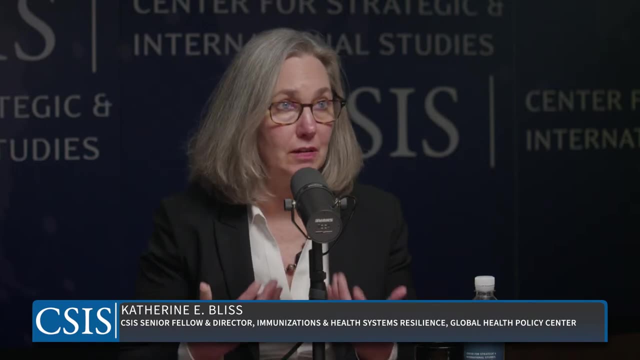 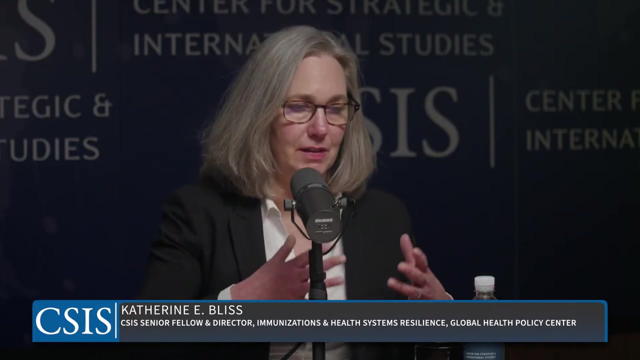 people where they're spending their time and finding them at work Or shopping or wherever they might be. Some of it also is relatively kind of traditional outreach right, Going to people's houses and talking and really just engaging in the social environment. But, Bill, I want to turn to you. I mean at the same time that it's important to really 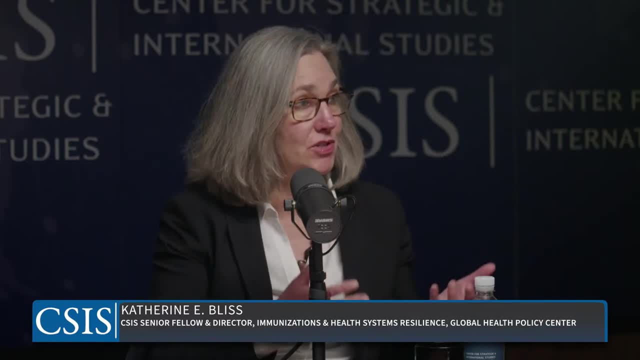 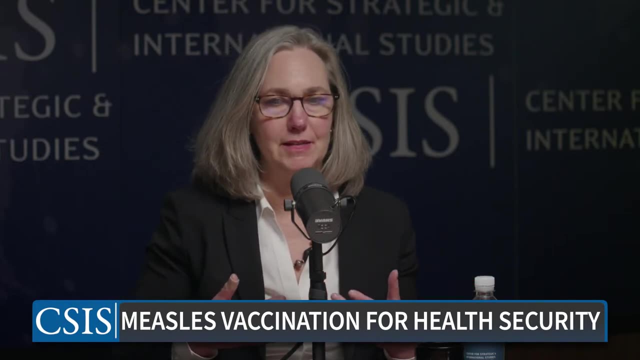 undertake maybe some of these more traditional methods. there are kind of new innovations in terms of delivering vaccines that may also even be used in the future. So I think that's a good example of how we can either make it easier to reach people or require different kinds of training. 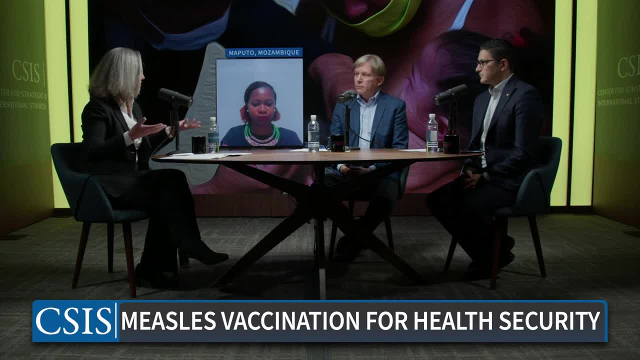 Could you talk about how some of these new innovations may change the measles vaccine landscape? Yes, certainly, And I you know the points that Graca and Daniel made about. you know, really trying to reach the communities is critical And there's, as you said, there's not just a technological solution. 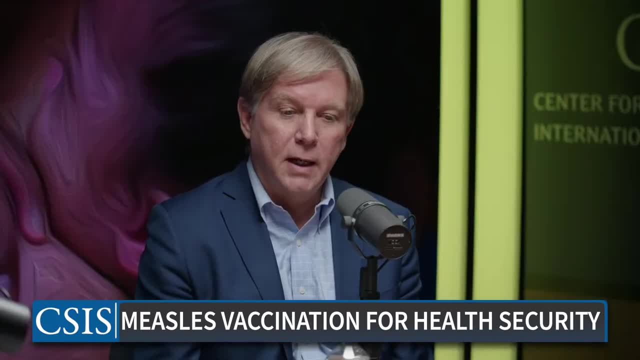 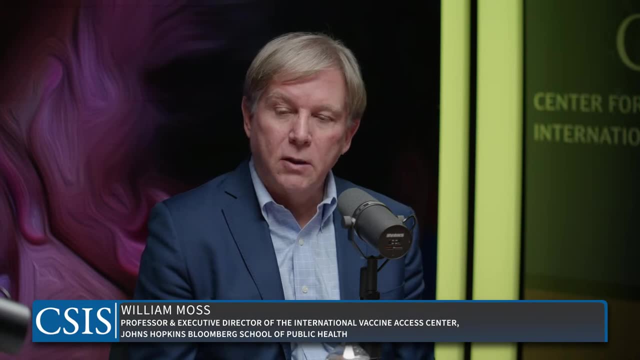 but in the measles world and in the vaccine world we're very excited about the potential for what are called microarray patches. And what microarray patches are they're? the devices are kind of like the size of a Band-Aid. They have very tiny needles on them that are coated with the vaccine. It's the same vaccine. 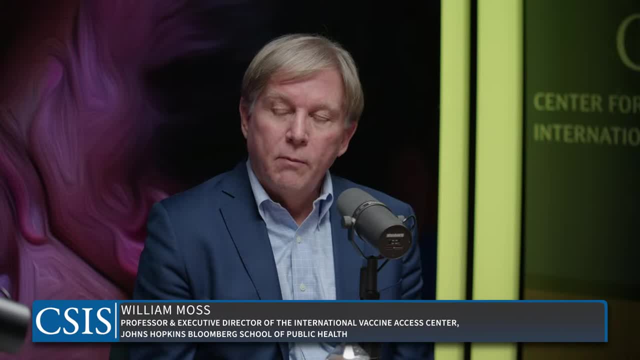 that we deliver by needle and syringe, But instead of kind of injecting it under the skin or into the muscle, they deliver the vaccine right into the dermis of the skin, where there are a lot of immune cells. So this is a technology that's been around for a long time, And it's been around for a long time. 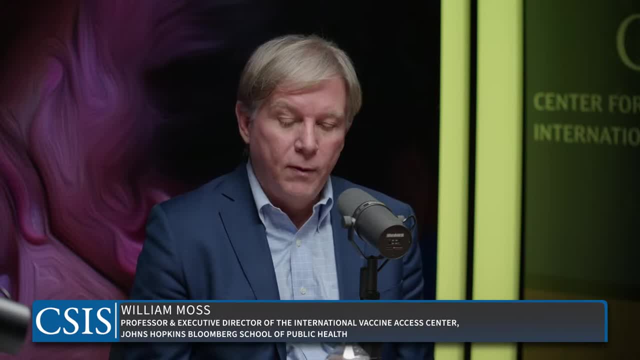 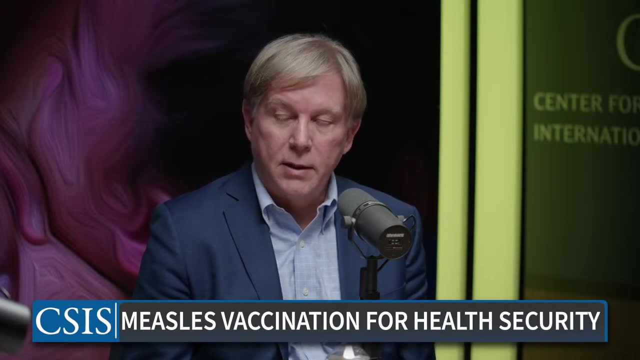 But it's slowly kind of moving moving forward And there have been some early studies that suggest that these are as immunogenic as a standard measles vaccine given by needles and syringe, meaning that they induce good antibody responses. But there are a number of advantages of this type of vaccine delivery. 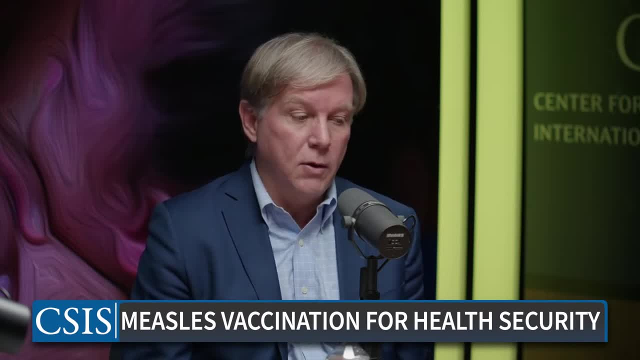 platform. They obviously don't require needle and syringe, So you don't have to need a needle or a syringe, the medical waste problems and the costs related to that. They don't require reconstitution. where measles vaccines are currently stored in a dried form, what we call a lyophilized form, They have. 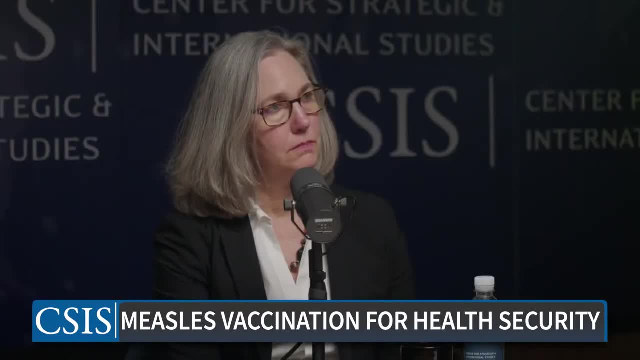 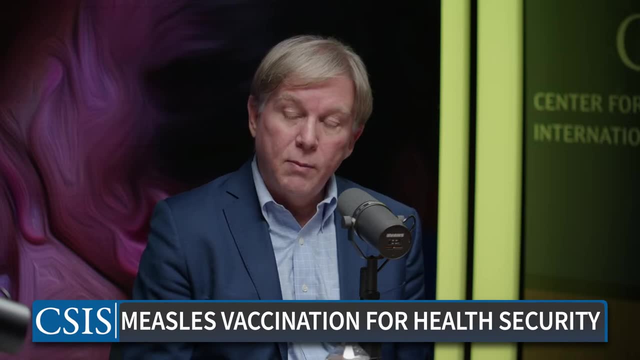 to be immune reconstituted with a diluent. There have been rare but sometimes mistakes made with the reconstitution. They're very thermostable, meaning that they can stand warmer temperatures, So you don't need that kind of rigorous cold chain. They could be administered by 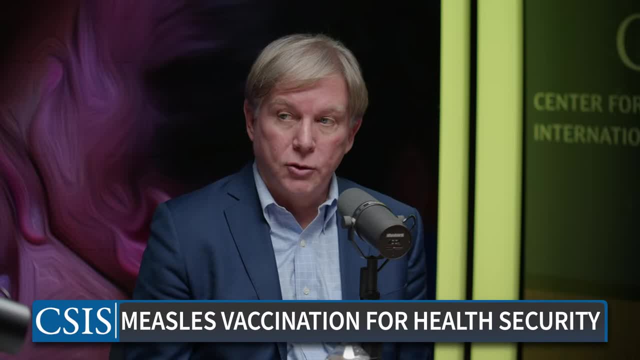 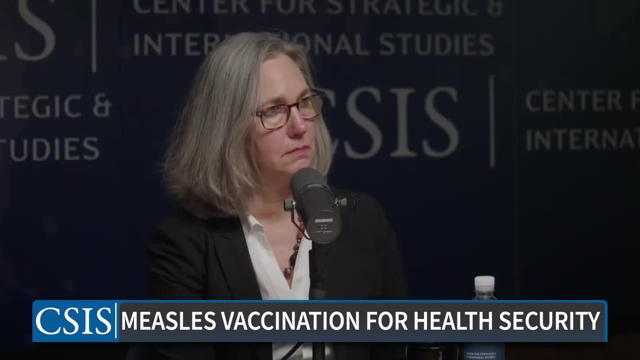 people other than trained healthcare workers- community health workers, for example- could administer them. They could even be self-administered And they're single use, so you don't have the problem with multi-dose vials where a healthcare worker may decide not. 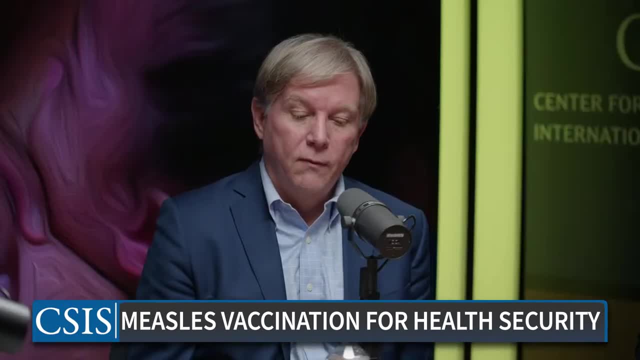 to open a 10-dose vial of measles vaccine for a child. We are kind of moving through the normal process of evaluating vaccines. There have been now in phase two trials in humans. There was an early study from Ghana that was reported about the. 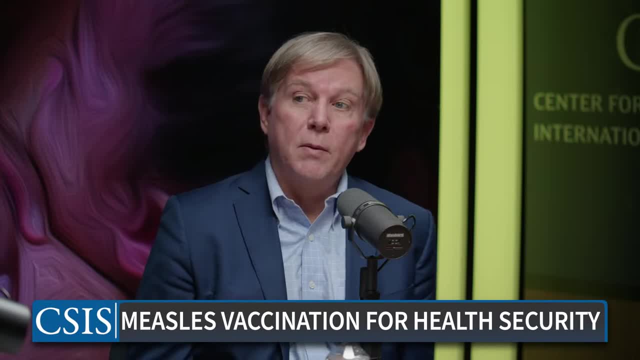 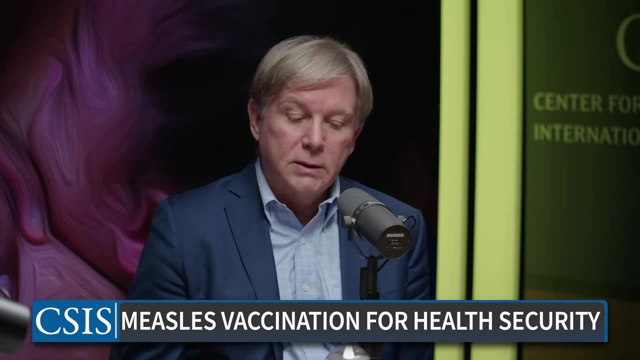 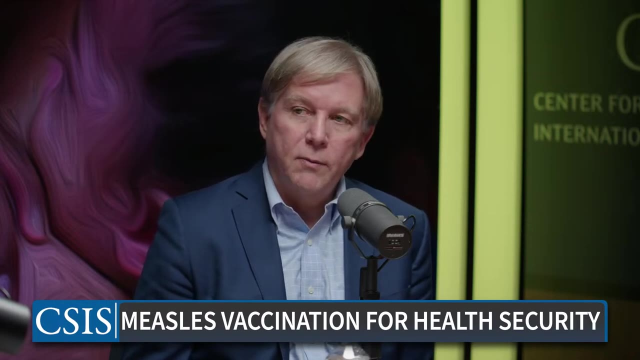 safety and immunogenicity And I'll also say the acceptability: parents, caretakers, much preferred that vaccine delivery platform And so it's going to take a while to kind of get this through the process, get manufacturing scaled up. It requires different manufacturing requirements. 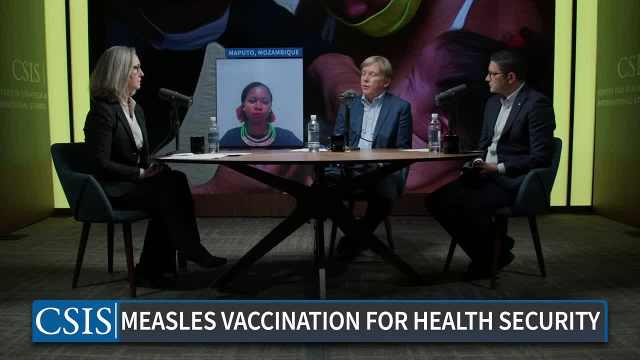 People are projecting maybe around 2030. I hope it's earlier than that- when these become available, But many of us in the measles world feel that these could be. this technology could really be a game changer for measles control, elimination and then, hopefully, eradication, Because of the 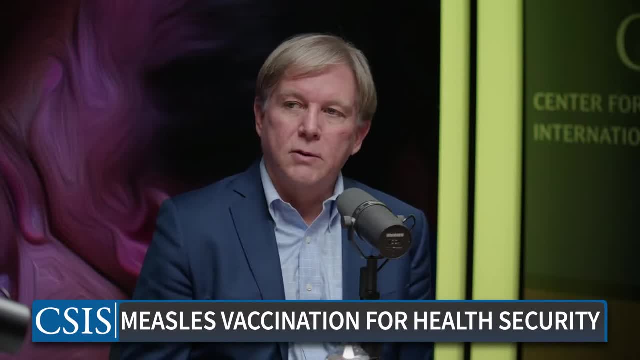 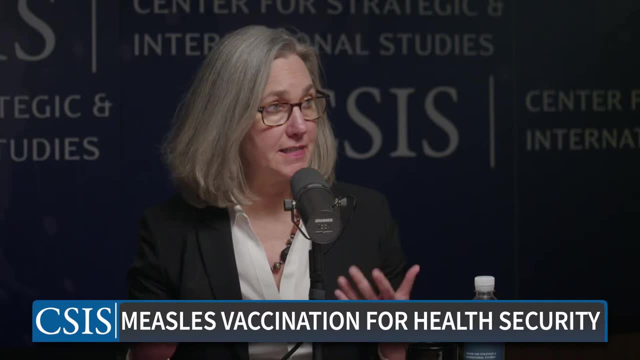 ease of administration. you can really take these out to those hard-to-reach children and that we've been talking about. So these could potentially address some of the challenges that Grasa raised, you know, around remoteness of the population or not enough healthcare workers or not enough trained. 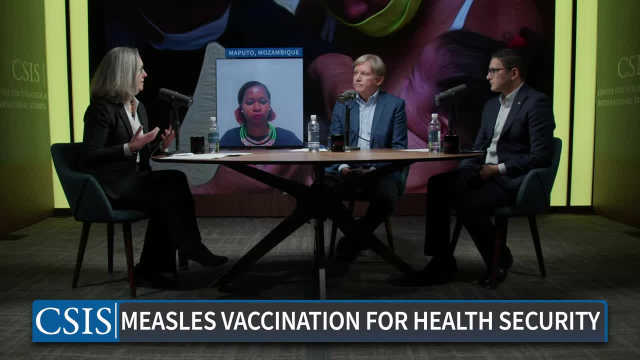 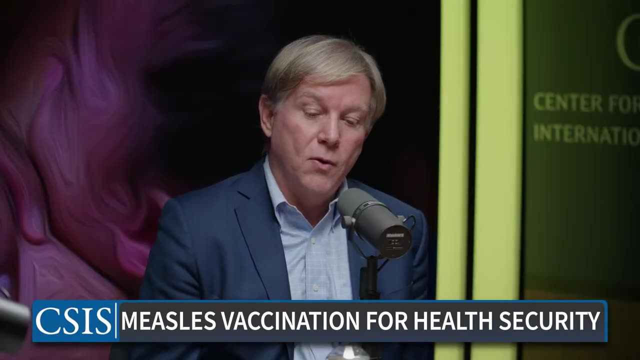 workers. How expensive are they likely to be? Yeah, we don't know yet. That's a key question. There's no doubt they're going to be more expensive than the current measles vaccine, which is quite inexpensive, And you know this is one of the challenges for the vaccine. 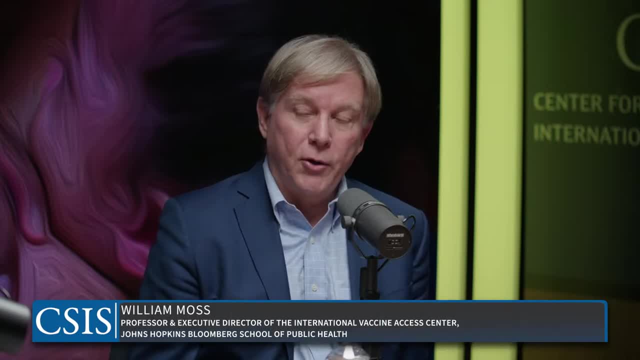 manufacturers. They're going to be more expensive than the current measles vaccine, which is quite inexpensive. And you know this is one of the challenges for the vaccine manufacturers is ensuring that there's actually a market for this. You could think of this, you know. 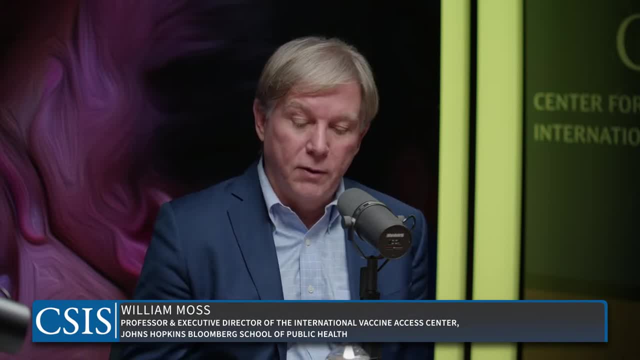 wouldn't this be great for kind of- I'll call it- the niche market for those 15% children you know who are very hard to reach. But that may not be enough financial incentive for the vaccine manufacturer. So there's a lot of discussion about how to have, for example, 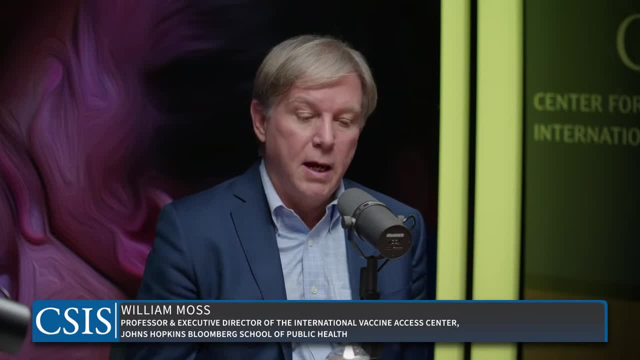 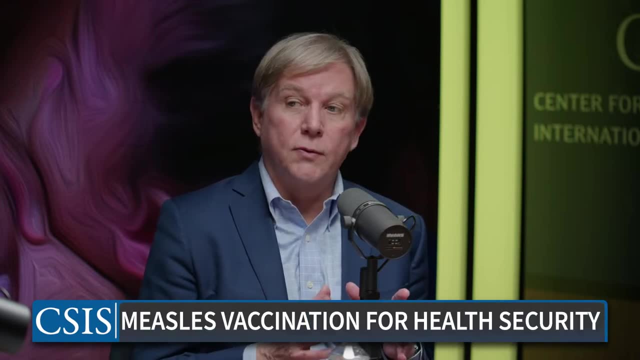 an advanced market commitment to help support, you know, finance these. There are these micro. this technology can be used for other vaccines and have been developed for other vaccines- influenza, rabies, polio. So you could imagine kind of a vaccine manufacturer, you know, using their manufacturing facilities to make multiple vaccines. 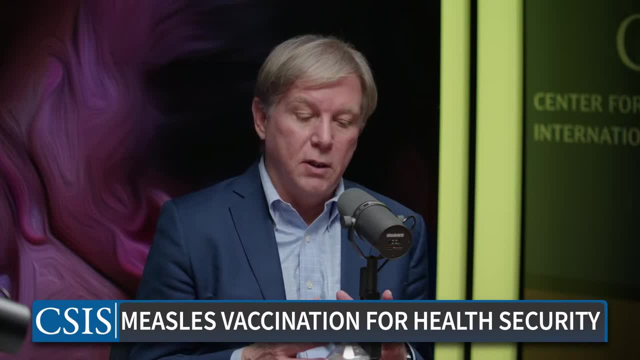 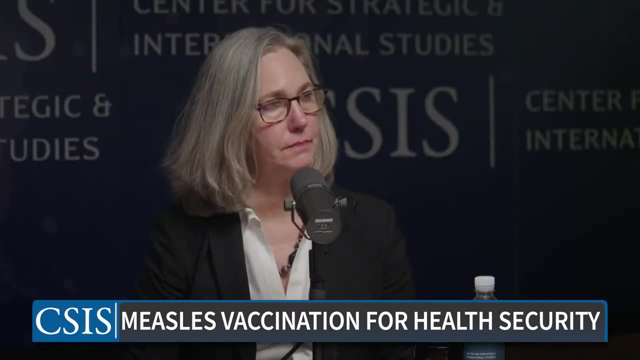 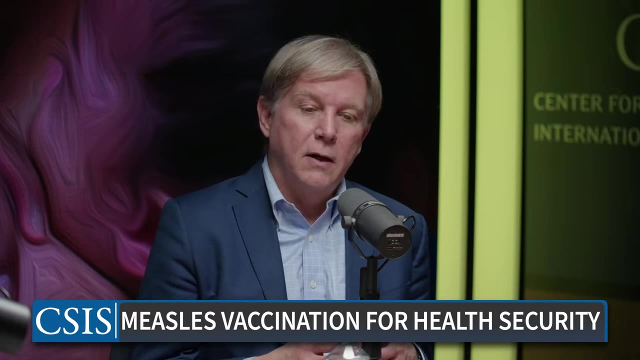 But that is one of the challenge that is that this field faces is that there's no doubt it's going to be more expensive than the current vaccine. And how much are willing, are governments, bilateral organizations willing, to pay for the advantages of that vaccine delivery platform? 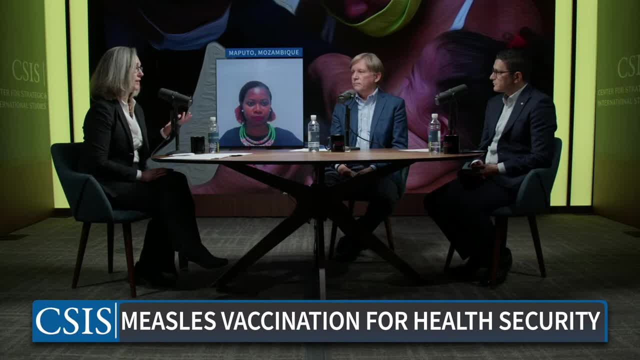 So cost and really financing immunization programs is kind of a perennial question. right, We talked a little bit earlier about the importance of really integrating measles into- I mean it is integrated into- routine immunization, but it's not integrated into routine immunization. 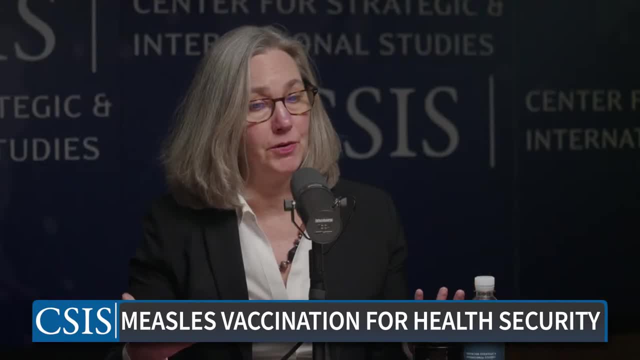 We're going to be talking about it a little bit later on, but I think the question of making sure these vaccines are delivered in the routine programs- because if not, then you, if there's an outbreak, you have to undertake a campaign which all of you have said is much more expensive- involves different levels of planning and workforce and the like. 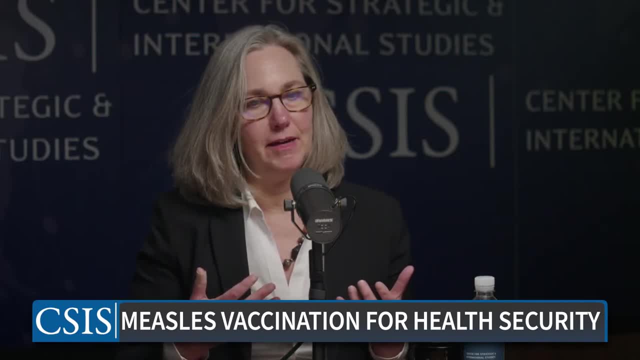 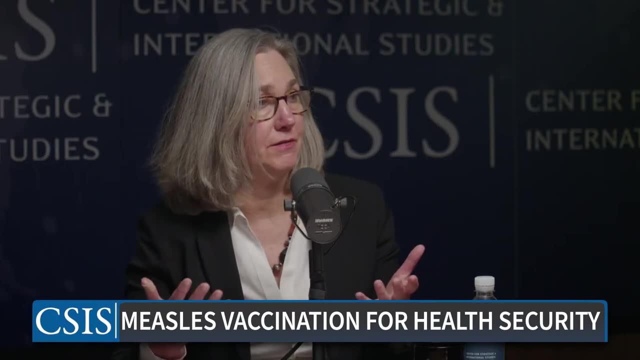 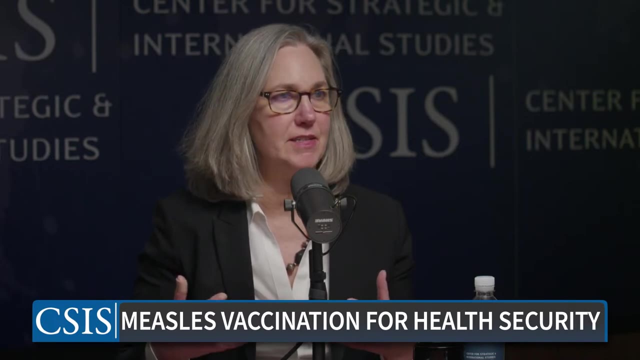 I wanted to just ask each of you to reflect a little bit on the importance of increasing financing for immunization programs and kind of what the needs are in the current context. You know we've come out of the pandemic where clearly lots of money was generated for immunizations. 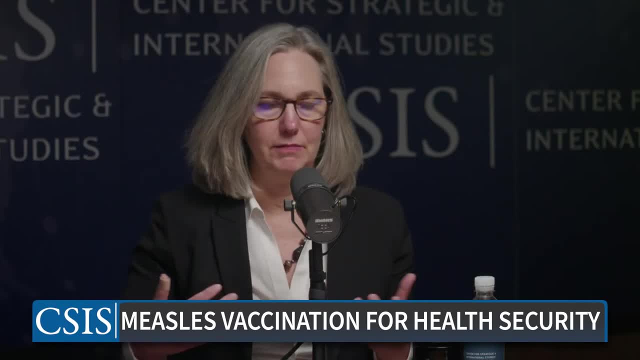 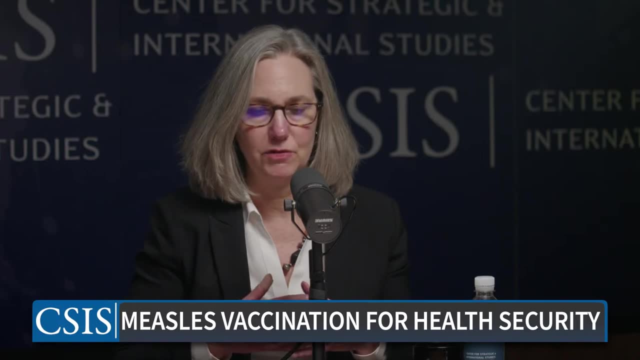 We saw COVAX and you know now there are, you know, plans for new manufacturing facilities in different parts of the world and you know real efforts to kind of drive, kind of shape the market, as you were saying. 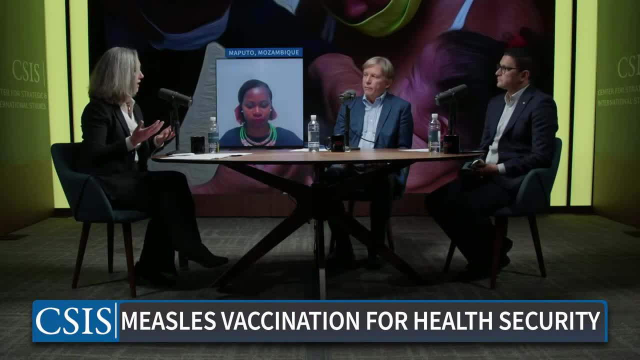 This is, you know, for countries that are eligible for GAVI. this is an important year. The replenishment and the start of a new strategic period will be starting in the next. I guess GAVI 6.0 will be starting in the next couple of years. 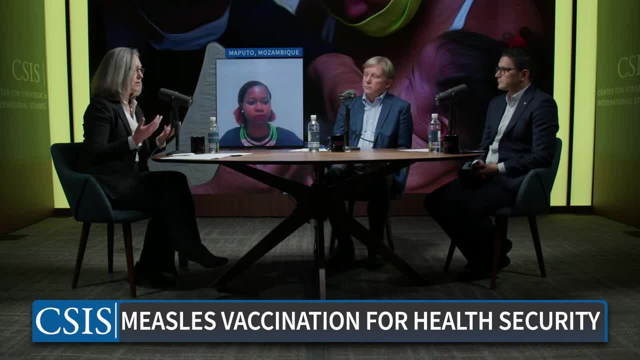 Obviously for countries that are regions that you know where countries are not eligible for GAVI. there are other concerns. A lot of the middle-income countries still face considerable challenges when it comes to ensuring equitable access to vaccines but are not eligible for those kinds of support. 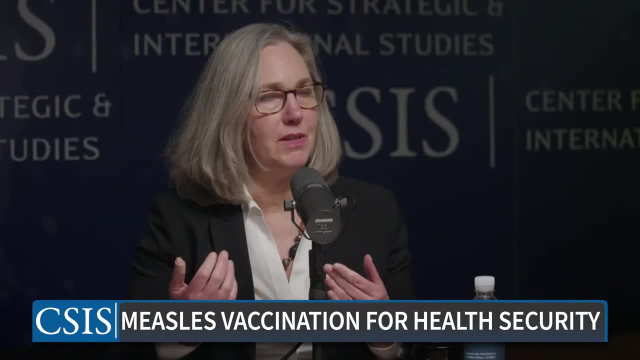 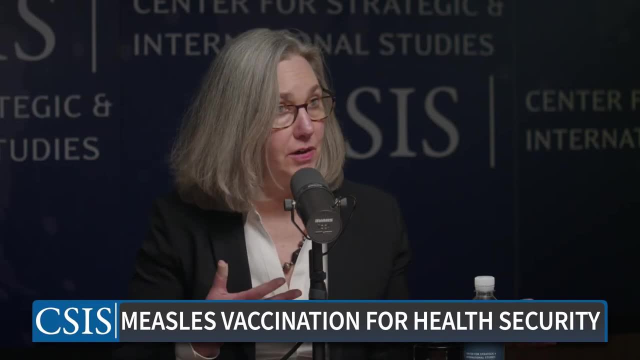 So, Danielle, maybe you know, let me start with you. I mean, most of the countries in the PAHO region are not eligible for GAVI support. Obviously there are donor countries you know to GAVI that are in the Americas, a few eligible countries. 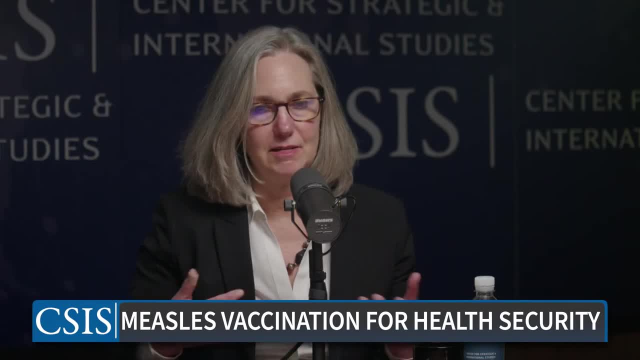 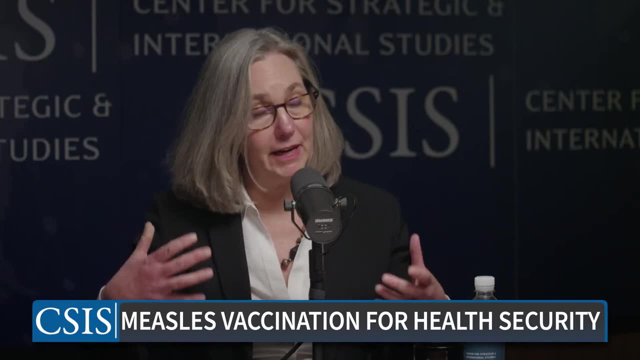 But you also have the revolving fund that has really shaped a lot of the market. Could you just say a bit about the importance of kind of ensuring financing- financing for immunizations in the next phase? Well, I think that the most important thing about this- 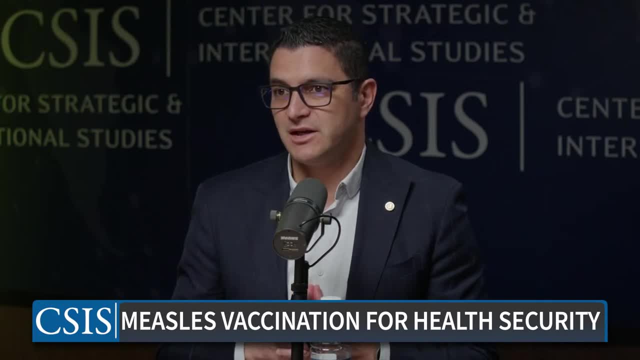 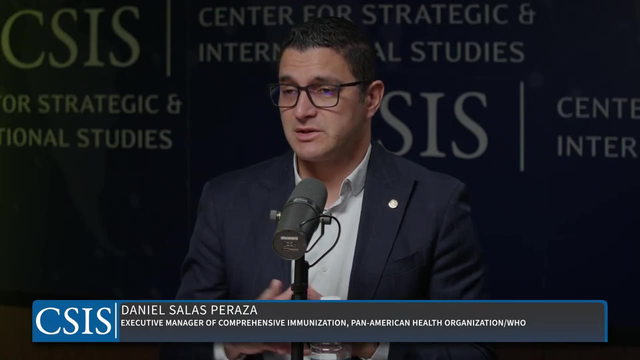 is to position the importance of vaccination on the policymakers, you know, the leaders, the president- because we need to look into co-responsibility. We should not, like, rely totally on an external donor And countries should be responsible. I mean, we're talking about the cost. 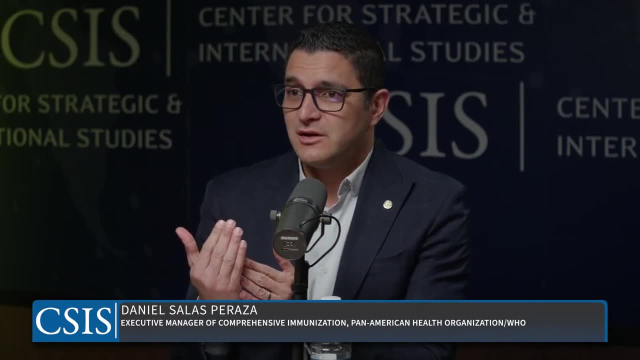 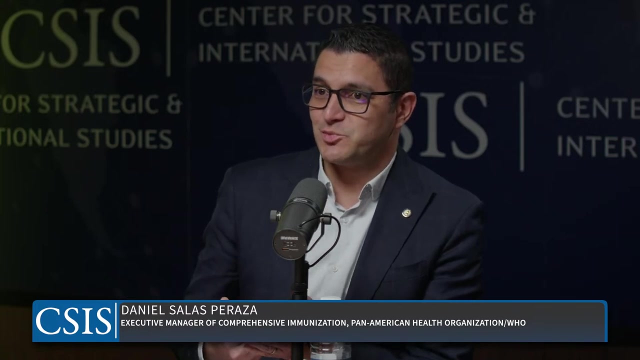 high cost-effective intervention vaccination And you're getting a return For each dollar that you are investing. you're getting several dollars per that investment, But the thing is that usually those dollars go to other programs, not to the immunization program. 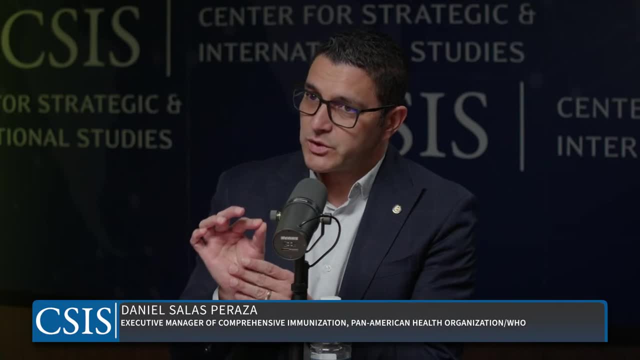 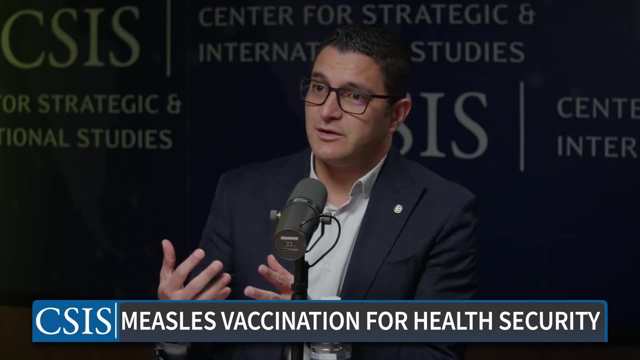 But the first thing that I think that we need to work on is to have this co-responsibility. We shouldn't let the countries to be totally dependable on external support. But of course we're going to need support. I mean the countries, and we're talking about India. 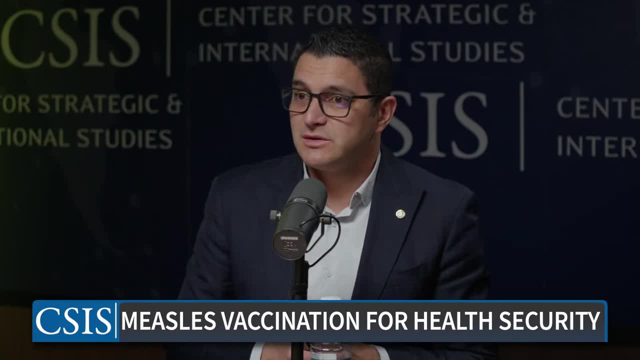 America and mostly in middle-income countries, they do not have the budget, the funding to really, you know, cope with all the challenges in health. And we know that non-communicable diseases, you know the burden of disease has been really getting, you know. 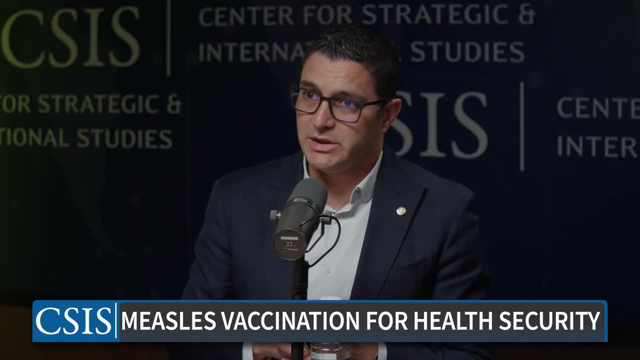 higher in the last decades And of course we need to prioritize, But what we have, for example, for the follow-up campaigns that the governments take responsibility about the measures you know that are being taken And that's the majority of the you know. 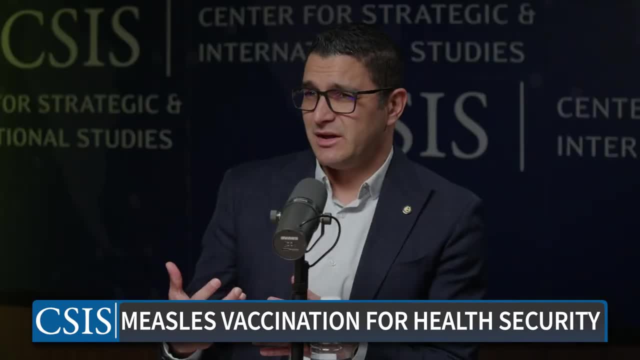 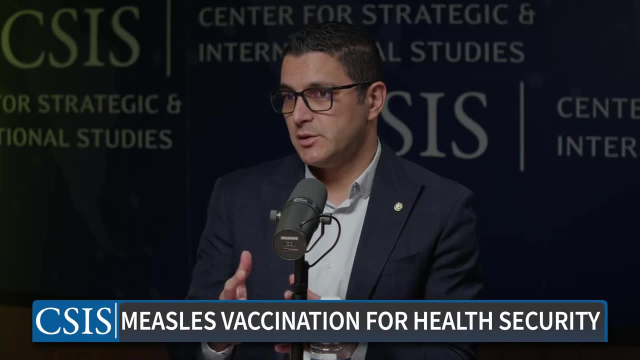 the funding for those follow-up campaigns. So it's not something that, oh, if, for example, an external donor is not going to help that, that follow-up campaign is not going to take place. No, it's not that way. 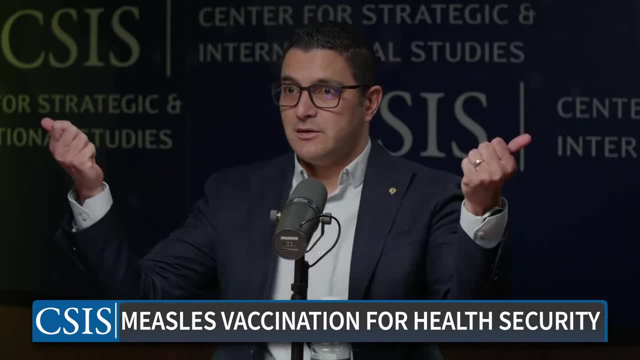 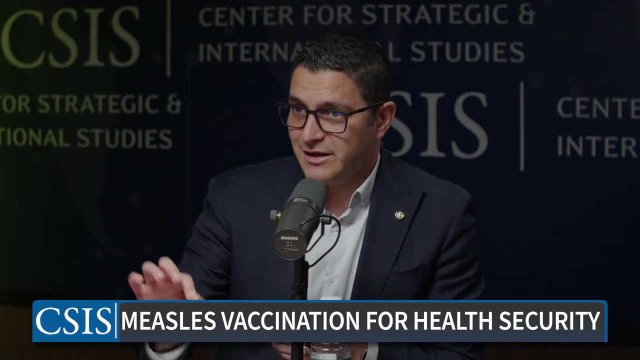 But, for example, we are always trying to, you know, canalize, to channel all those funding that we can get to really give that extra, you know- support for countries Because they need- I mean, we're talking about middle-income countries- 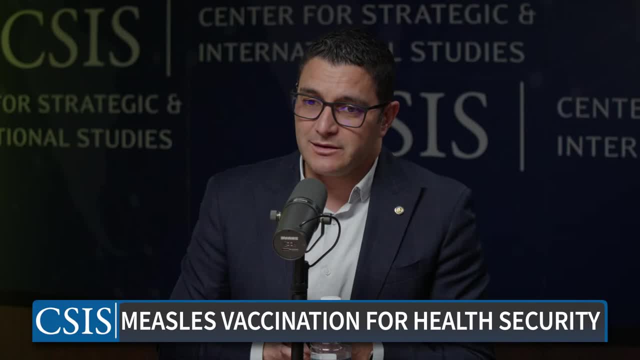 They need that support, But of course we're not. I mean we're expecting what is going to happen with the mixed strategy and Gavi 6.0. We're really hoping to get more support from Gavi. We don't know what is going to happen. 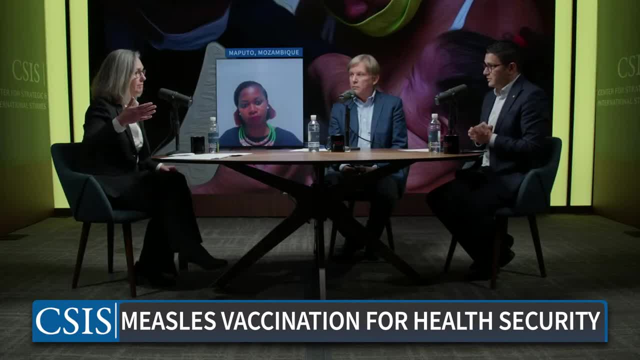 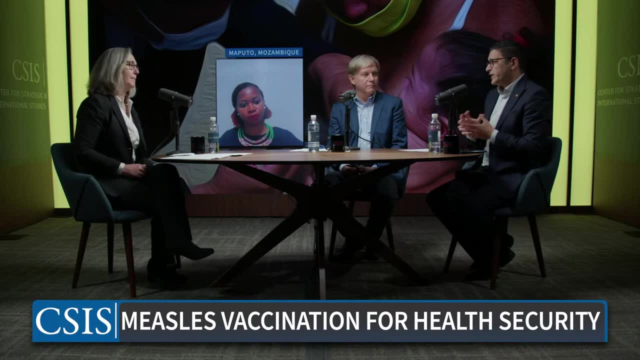 Sorry to interrupt, but when you say the mixed strategy, that's the middle-income country strategy where there's been some technical assistance, But it's an ongoing discussion. Yeah, The criteria that they have, you know, chosen for this strategy is very like strict. 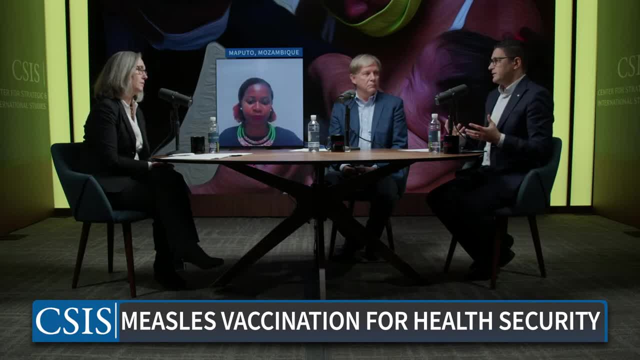 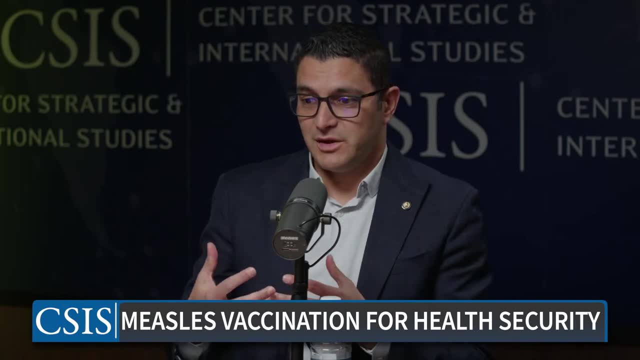 So many of the countries that, for example, we have a lot of polarization, We have we are the most unequal region in the world, you know. And so it doesn't mean that because you have, like, a threshold of being above a percentage of income, 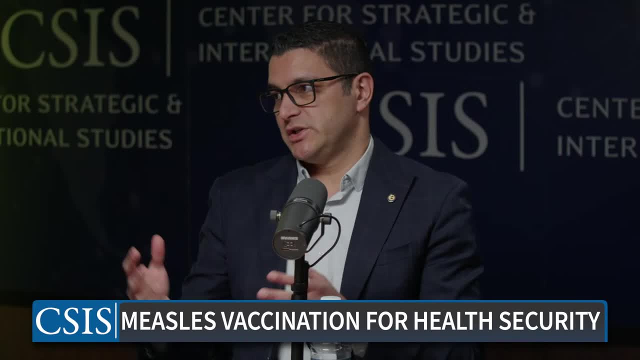 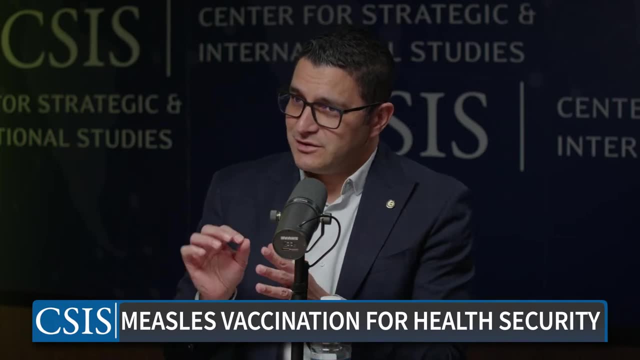 of general GPD or whatever. it means that that country is totally sustainable and can really face all the challenges in vaccination or other topics. So that's something that I think that there should be like a more comprehensive approach, you know. 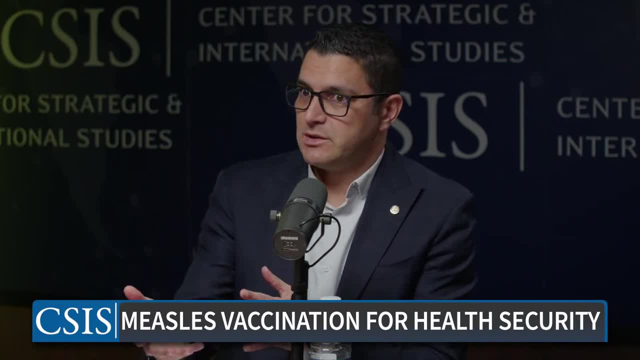 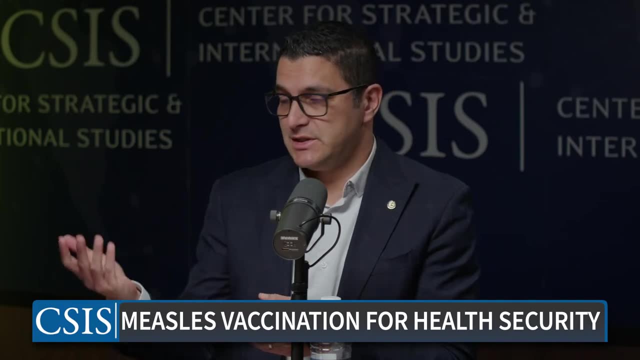 on defining which are the criteria for a country to be eligible to have extra funding. But of course we're always looking with our partners. We have a longstanding partner, for example, the CDC, the GID, the Global Immunization Division. 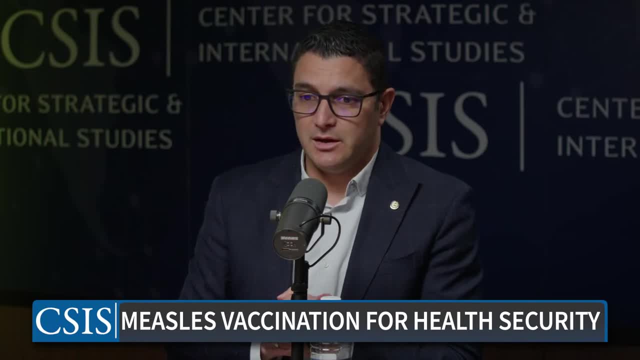 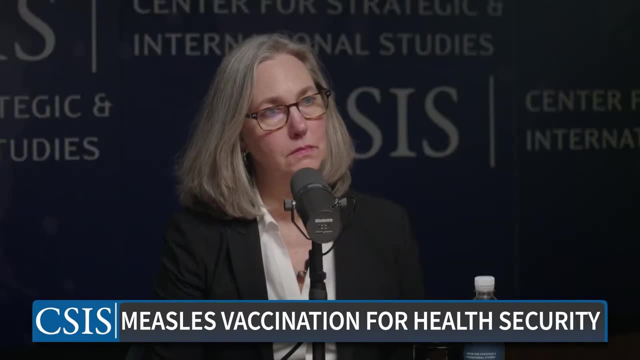 and they have helped a lot our countries And we're always, for example, for measles, Red Cross has been a great ally in the past And we're always looking, for example, for polio. we have the Rotary Foundation. 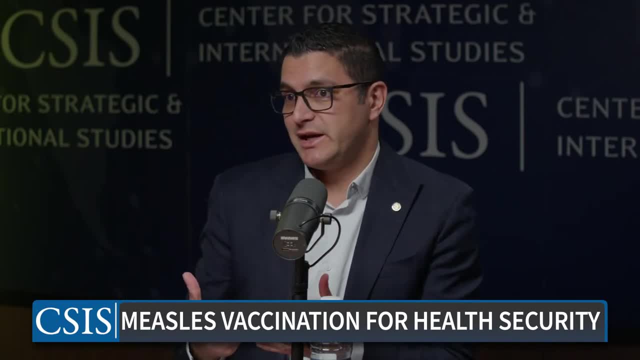 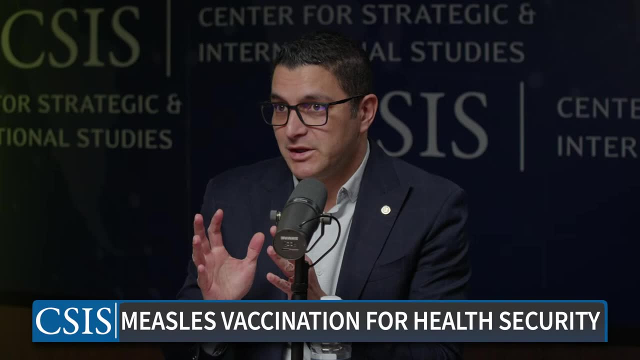 But we're always looking. We're always looking to get, of course, extra aid, because countries are not self-sustainable. But one message important here is that we should not like make them believe that if they do not get the funding, 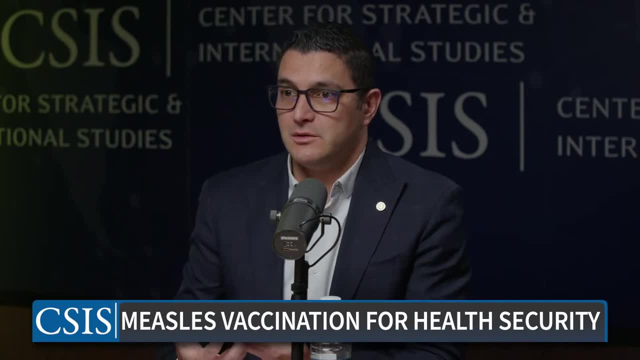 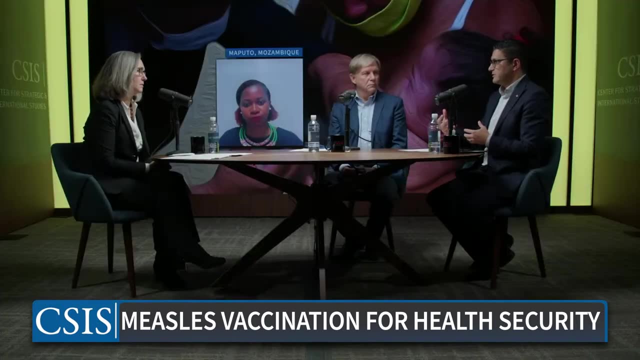 I mean nothing is going to happen to strengthen the EPI, the Expanded Program of Immunization, because countries should take responsibility and should take that accountability of what is happening in their countries. But of course I mean, and that's something. 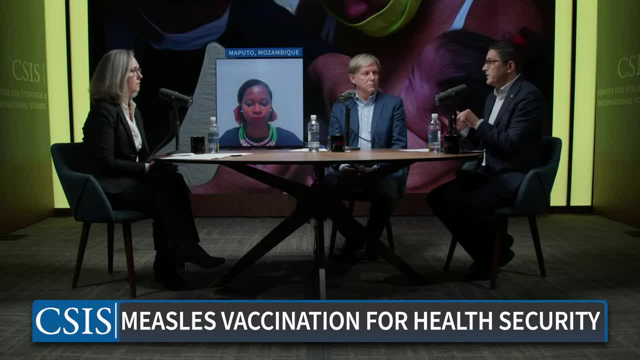 that we really need to continue working and we're now working on a methodology to develop a methodology to estimate the impact of the overall vaccination program, because sometimes we really proceed with this just for the introduction of new vaccines but not for the- I mean for the regular program. 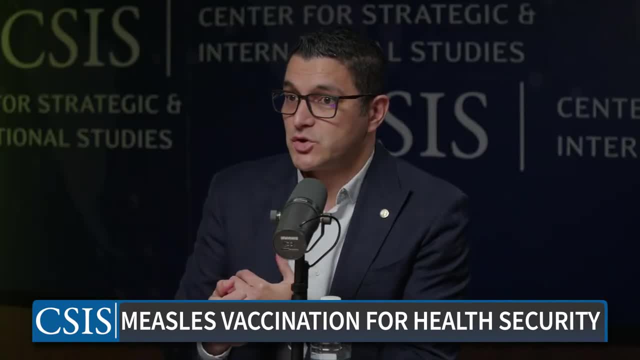 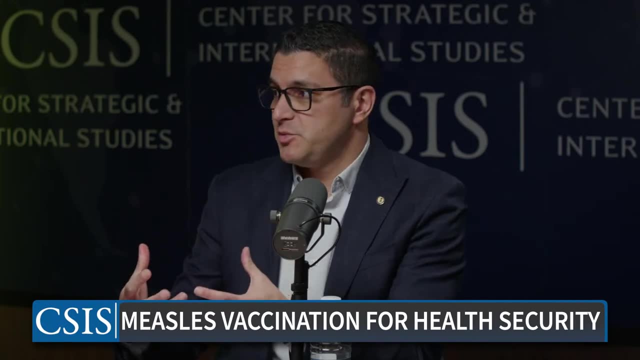 What has happened with education? What has happened with- you know- tourism? What has happened with production? What has happened to the workforce? Because we have been having strong programs on immunization. so we're working on these to really get to. 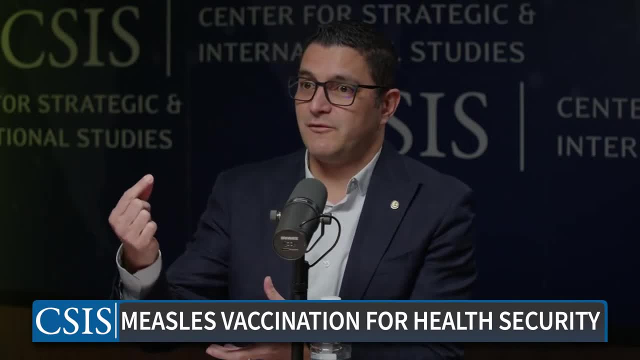 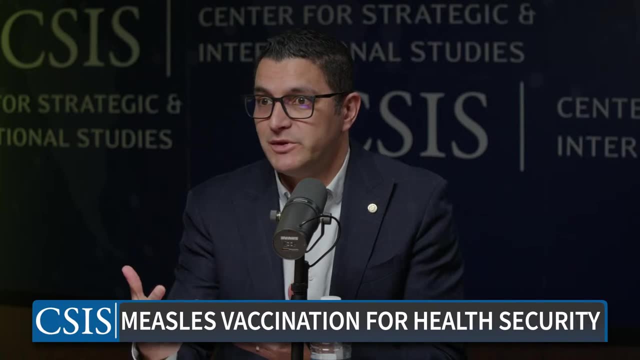 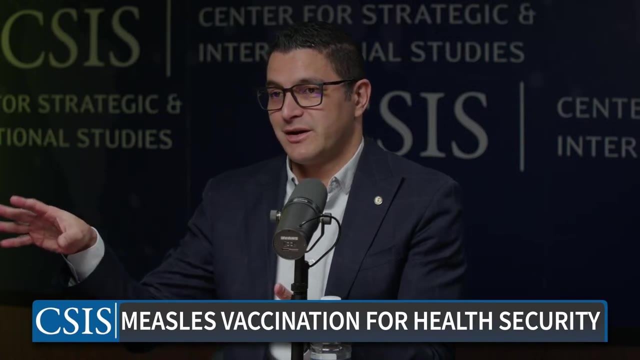 you know, to the ears of the president, of the minister of finance, of the minister of education, because they need to hear. what does it mean to have strong immunization programs for them? not, we always are counting deaths and disease or and the people that got sick. 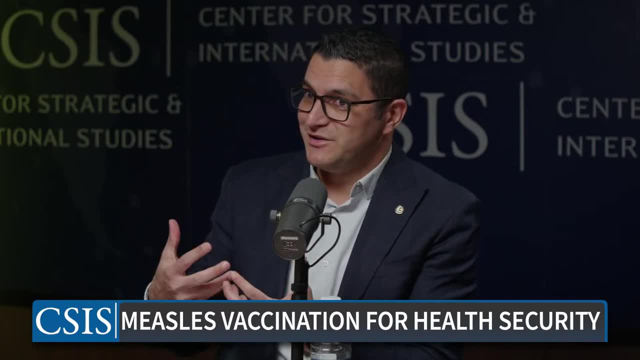 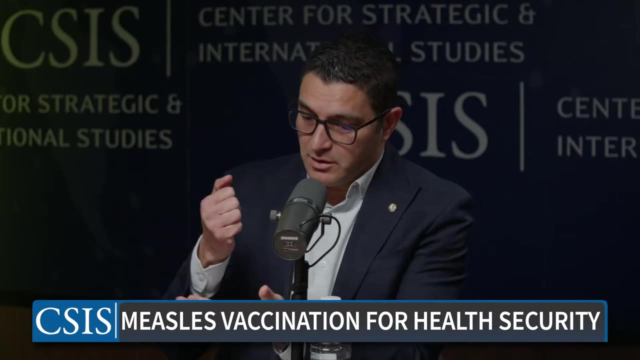 but not are talking in their terms. you know, We need to apply some kind of social marketing tools to really convince them, to get them engaged and they see the need To the Congress, to everybody that could take a decision. we really need to get those people with, you know. 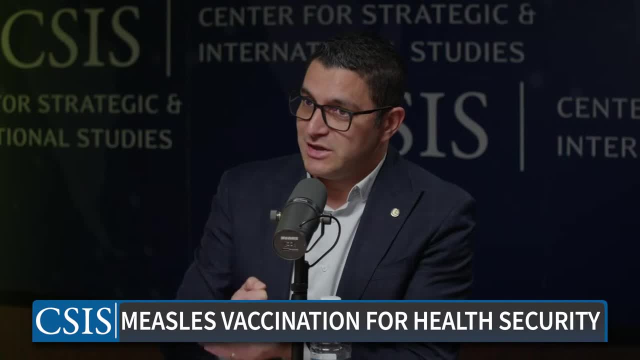 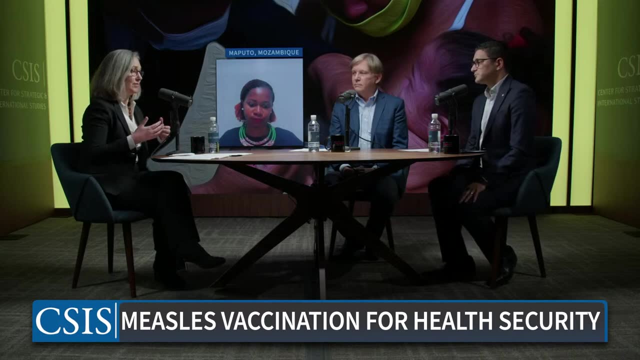 very clear messages about why it is important to have strong immunization programs. So it sounds like it's really needed to have that- just a frank dialogue around policy and the importance of investments for the overall economy, not just kind of the specific health aspects of it. 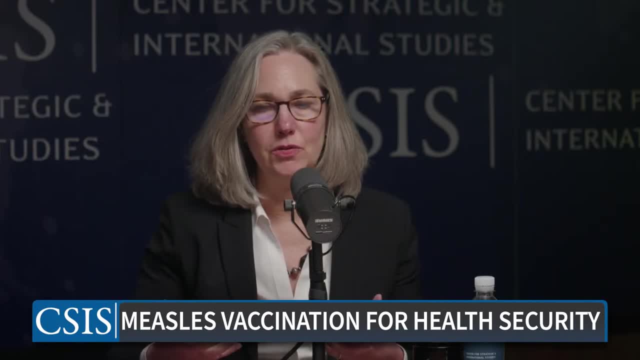 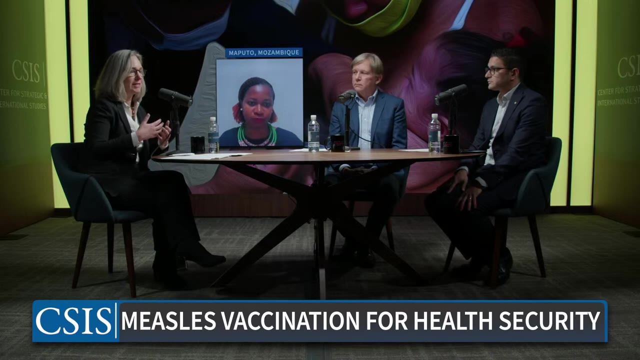 Well, let me turn to you. I mean, what are you hearing in your conversations in Mozambique around the? you know thinking in terms of co-financing and the? you know some of what is likely to come forward in the next round of, you know, the Gavi discussions. 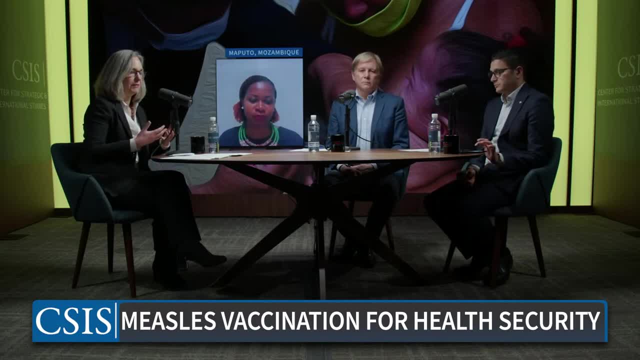 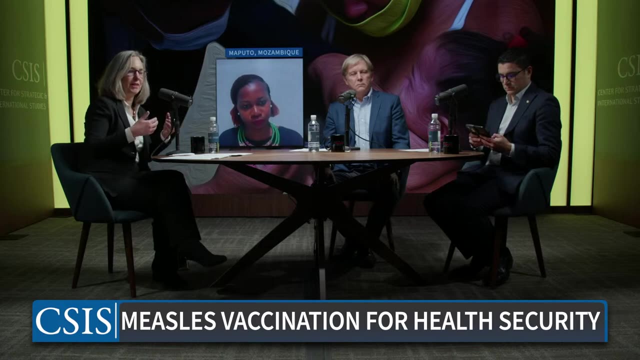 and the formulation of the next series. is the discussion around financing something that Amrite is involved in, or is this you know? are these you know, bringing together the you know, the discussion around the investments and the importance to the larger 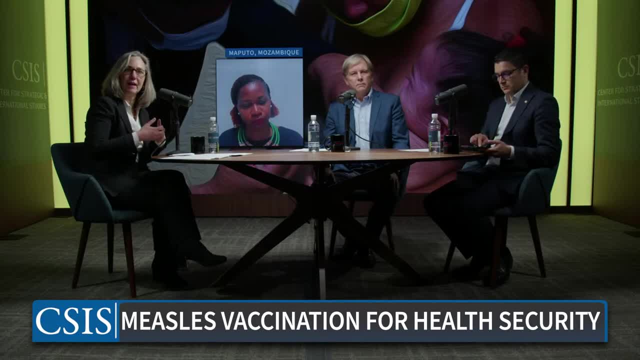 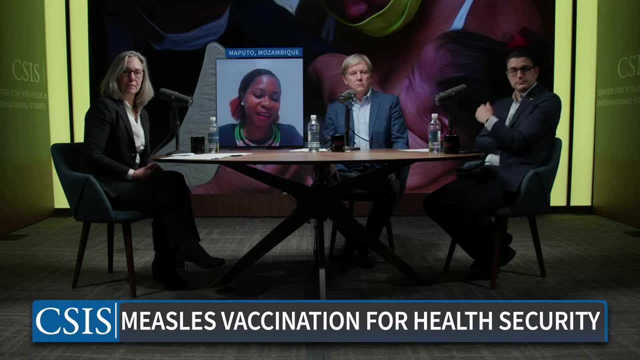 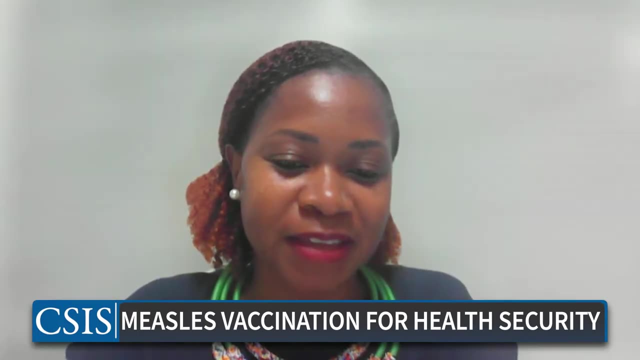 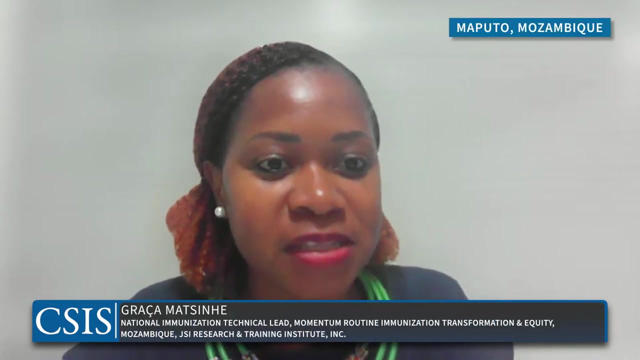 economy. You know, where do you see that conversation taking shape? Well, Catherine, one of the gains we had from the COVID pandemic it was that the very first time we had different presidents or heads of state talking about vaccines and vaccination. So COVID was not, definitely it was not- a good situation, but from that we could have 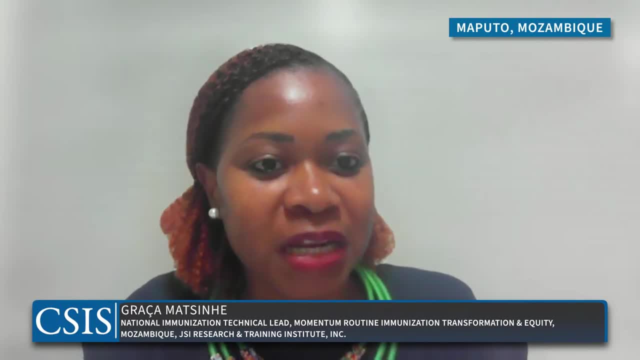 this understanding from the political leaders on the importance of vaccines, which we had been battling for years and decades to make them understand that vaccination is really key for the prevention of diseases. So in at that level I think we now know it's much easier to be heard when speaking. 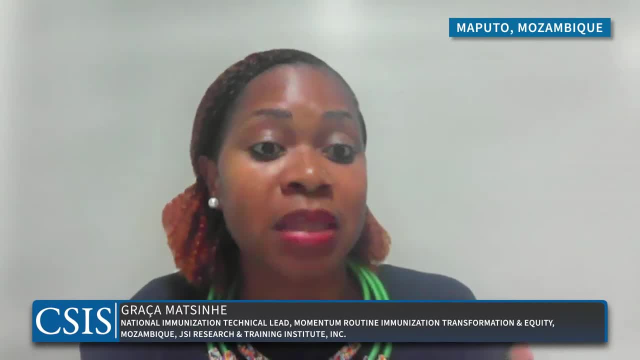 about vaccines, the importance of having children vaccinated and the importance of having investments to make sure that the vaccines are there. Well, one thing is what they know, but the other thing is what they don't know. So you know, I think you know, I think you know. 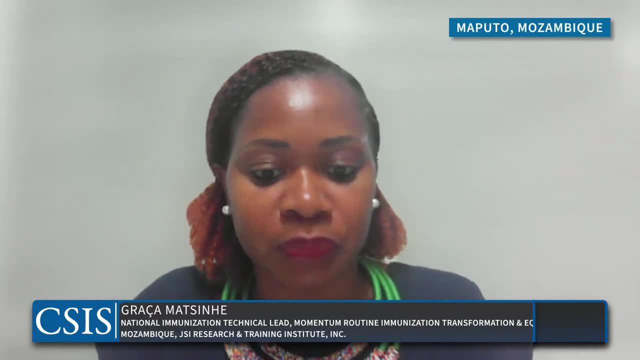 it's not difficult. It's not difficult to have these kind of decisions with the government. It's not difficult to have the voting power. We can have one or two prizes in a minute. We can have a little bit of time to think about the pandemic. 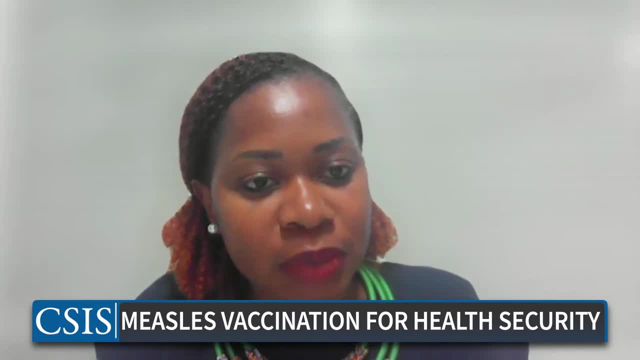 So it's not like you know one or two, but the main thing is what happens in reality. So definitely, like Daniel says, we need to continue working in terms of doing advocacy with the political leaders so that they can increase the domestic funding for immunization. 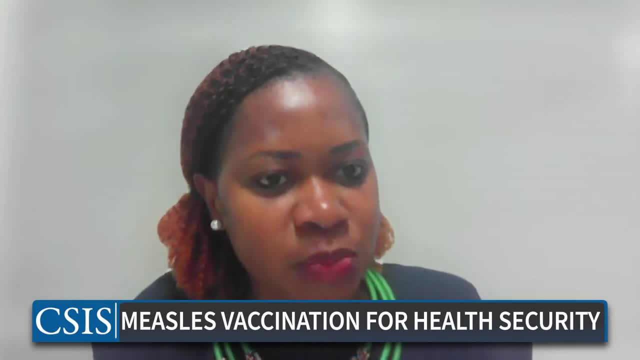 Of course, they say that there are a lot of priorities, But, yes, immunization is a priority. If you vaccinate children, we ensure that we have a human capital that is healthy in our society. So I think this is very important. 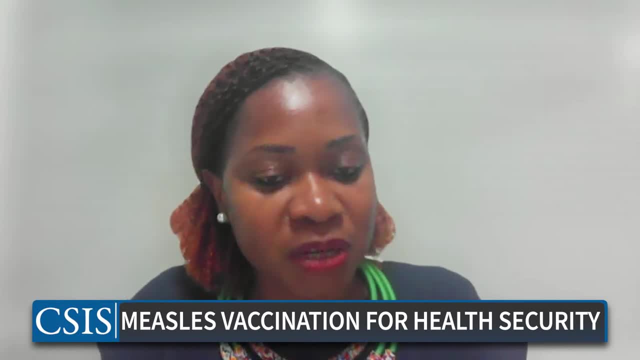 Thank you, is what we have been doing, um. we have been addressing um as a group of partners. we have been addressing uh the party, the parliament, so that they can understand the importance of um channeling more resources to the immunization program. so this is an ongoing work that we'll 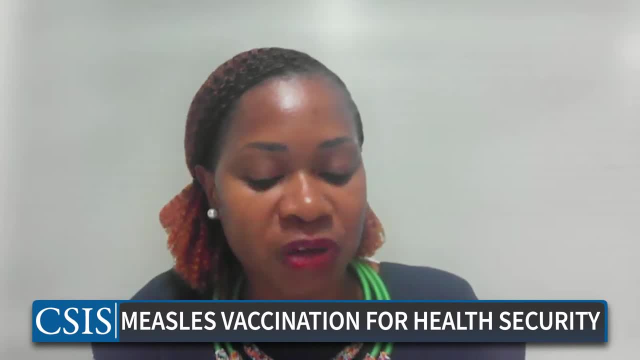 continue doing um as a group to make sure that the financing is is increasing, but also um i want to bring here the the idea of exploring non-traditional partnerships. we have a very good experience from covet vaccination, where we had we we involved the private sector um to 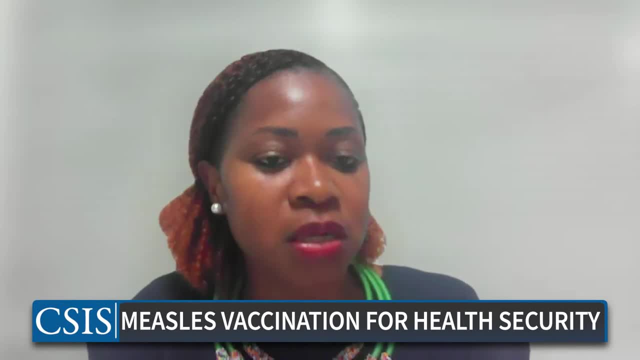 mobilize resources for to buy vaccines and also supporting us in the implementation of vaccination in the remote area. so i think those are things that we really need to explore and most of the time when you're thinking about financing, we only- i mean when we think about. 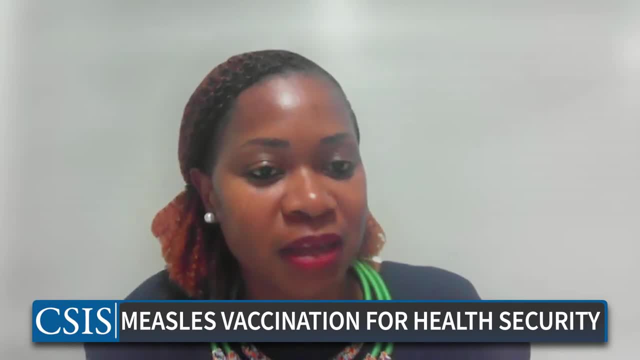 the vaccine. we only i mean when we think about financing. we only i mean when we think about support. we think about only the financial support. but they are, they are non-financial support that we can benefit from, especially um with the, with the economic um agents in the rural communities. 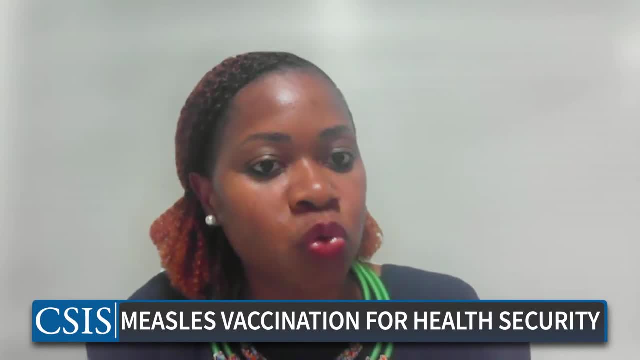 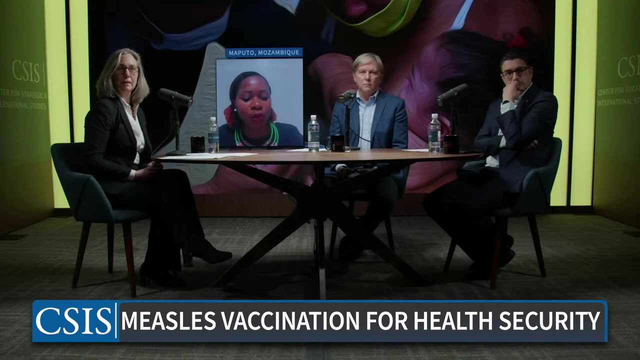 so those are things that have been discussing in the immunization working groups. uh, in order to find alternatives for financing the immunization program, um when we're talking about the co-financing, um in in my context, in in my country, the government has been consistent in in. 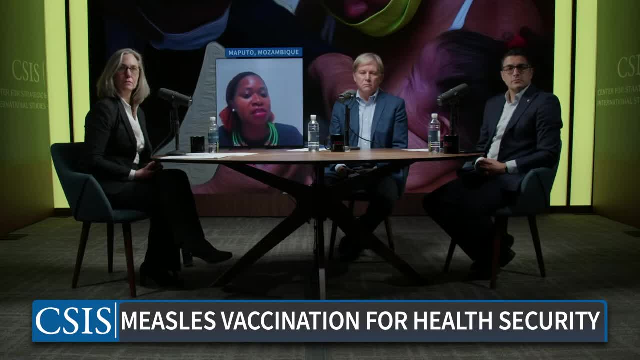 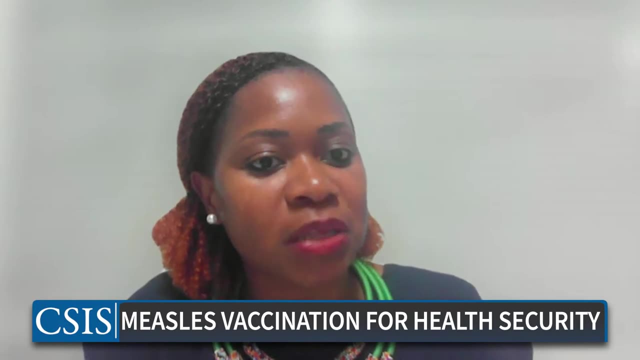 complying with the co-financing requirements. but as the vaccines increase in the calendar, obviously the obligation also becomes larger. so it's about time for the government to set priorities and um and make sure that more resources are channeled for the immunization program. um, talking about the government replenishments, yes, the funds are there, but we cannot only rely. 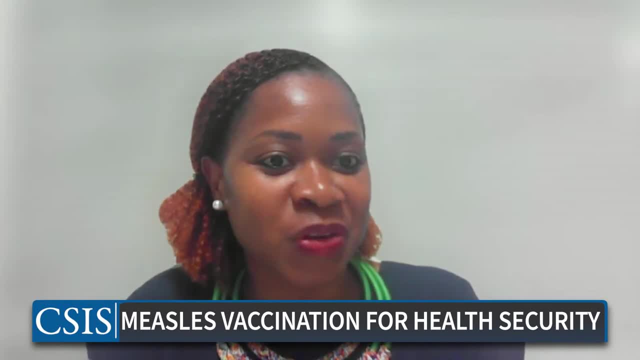 on government on gavi funds, because they're not. they're not not limited, less one of one day you can wake up and no funds to support the country. so i think i want to stress this importance of governments working together to raise funds to support the implementation of immunization programs, especially in low and middle income countries. 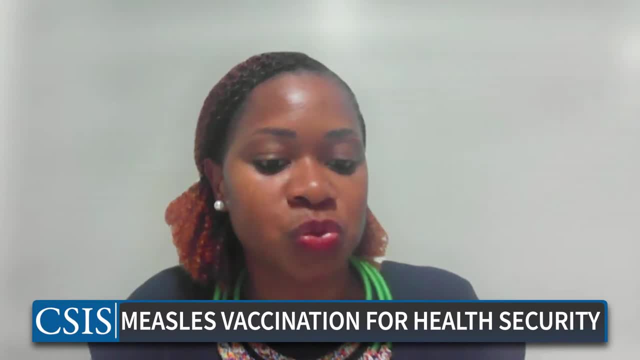 where they really need those, those resources. however, the replenishment is also an opportunity for countries to narrow down the priorities, because we want money for everything and it's not possible to cover everything at once. so, um, i see the replenishment as an opportunity for us to look exactly what we 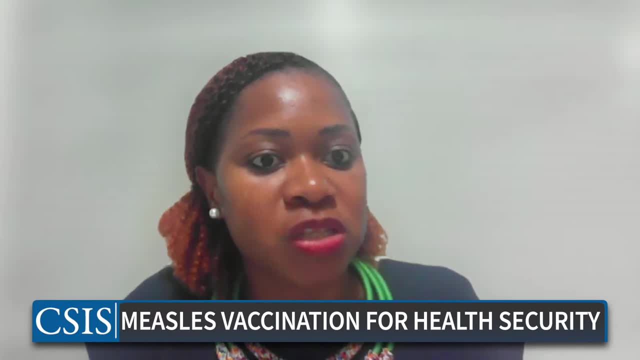 want to do that. we have a very good impact in the immunization services. i look, i, i see here the importance of scaling up the red and red strategy, which is crucial for reaching um the dreamed, improvingными our um a point in time to the future, after um, before we have to show. 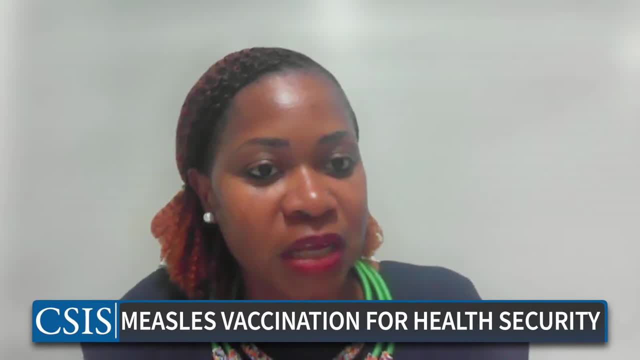 what we are um the goal of um MeerabuH's uh on, which is a very significant goal, um which would be actually to bring what's actually the most important- highest quality, effective medicine to exit uh zoonomics um to process this. on behalf of uh. 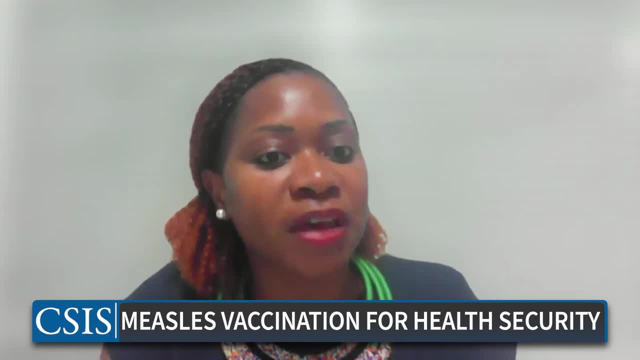 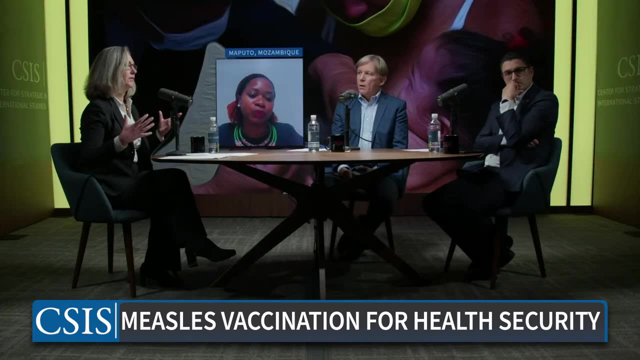 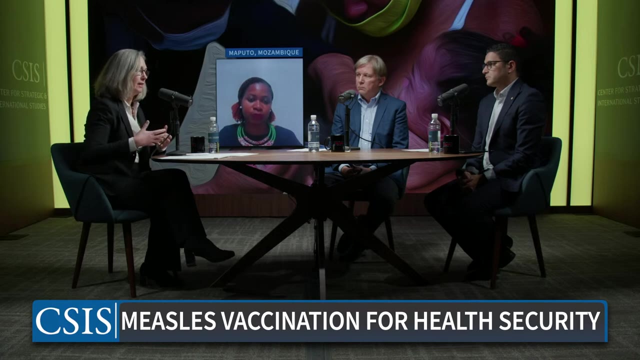 to improve the cold chain and the availability of vaccines through the resources that Gavi will be providing in the next cycle. So all of you have really emphasized the importance of multisectoral partnerships in not only financing but really thinking about some of the different technical challenges that 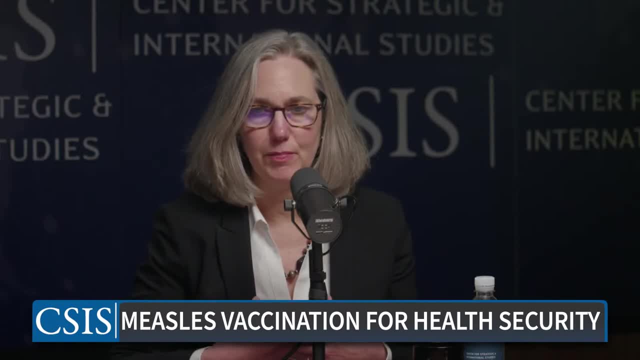 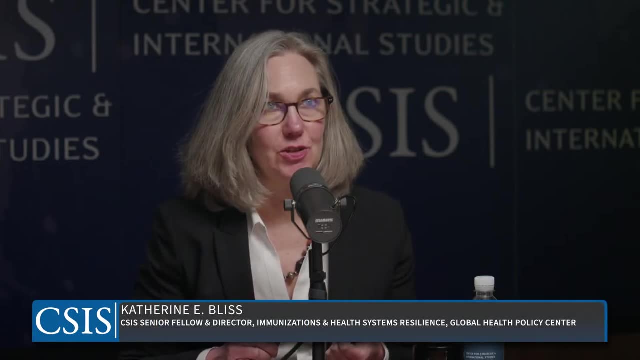 are currently faced and even some of the political challenges that you've talked about as well. I want to turn to the issue of vaccine confidence, that several of you have also raised, and, of course, the issue of partnerships there, both in terms of thinking about communication. 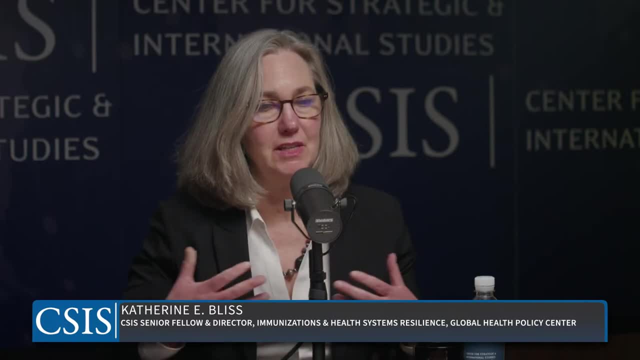 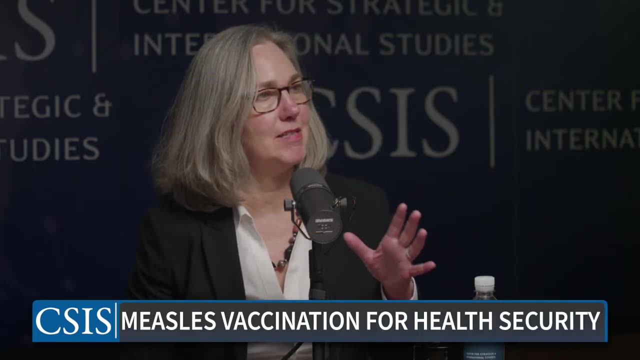 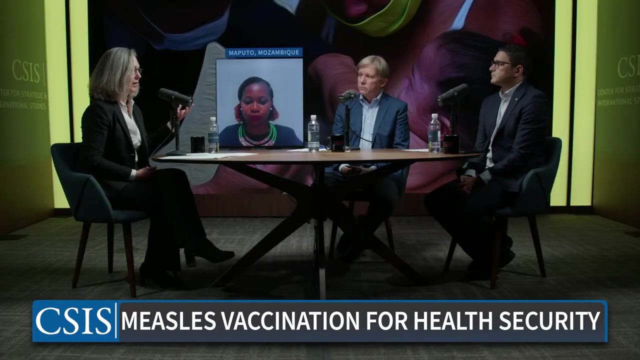 around vaccines, but also just some of the different media that are used for communicating about them as well. Bill, I want to start with you because before we came in here, we were talking a little bit about your work in Zambia. You started out working with a hospital that had a ward that had what 30 or 40 beds filled. 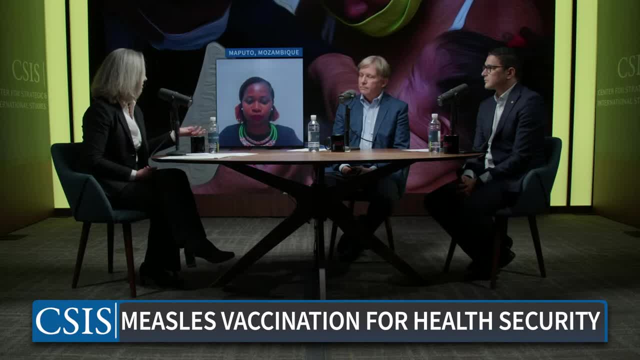 on any given day with children with complications from measles right, But then over some period of time that ward was once vaccines had been introduced- was really not in service as much anymore, And so over several decades certainly we've seen this here in the United States and elsewhere. 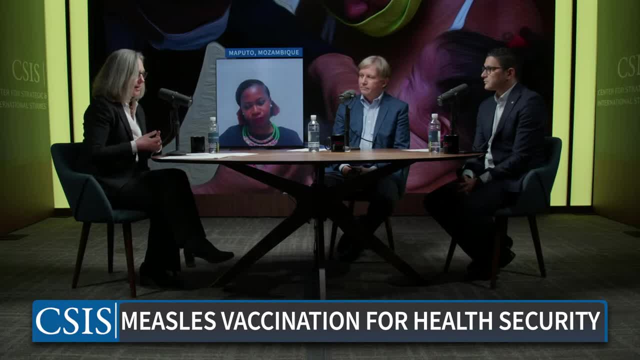 people have kind of forgotten, And so the challenge really is, maybe not in areas where the rates are lower, but could you say a little bit about you know, reflect on that experience but also the work that IVAC has done, you know, around vaccine confidence and what some of the current challenges with? 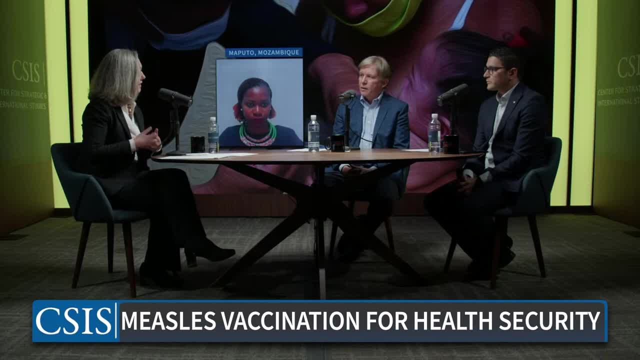 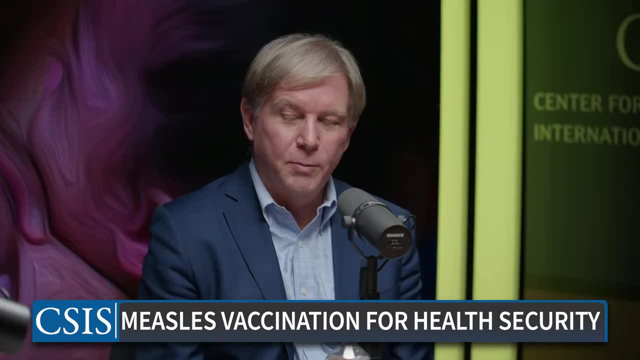 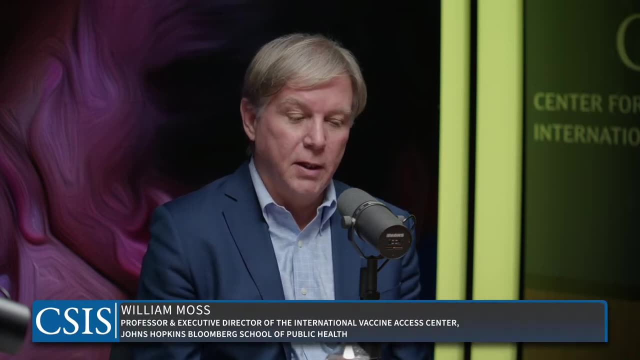 respect to measles vaccinations in particular, are that you're seeing? Yes, Well, Catherine, it was quite remarkable to see in Zambia, You know, a hospital ward filled with children with measles And then, after Zambia conducted their first mass measles vaccination campaign, to really 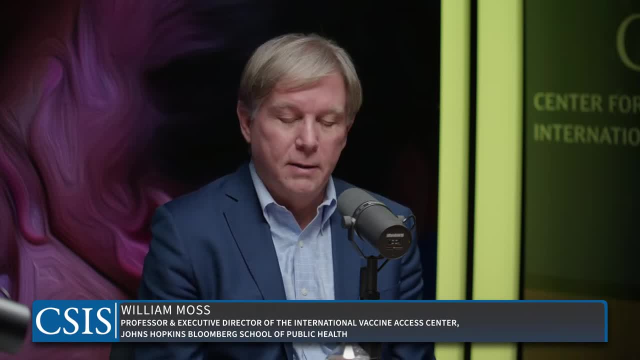 see that ward go away. measles hasn't gone away in Zambia, but that measles ward was eventually shut down. I think of you know just some higher level reflections. You know when I think about vaccine hesitancy and vaccine confidence first of all, I think 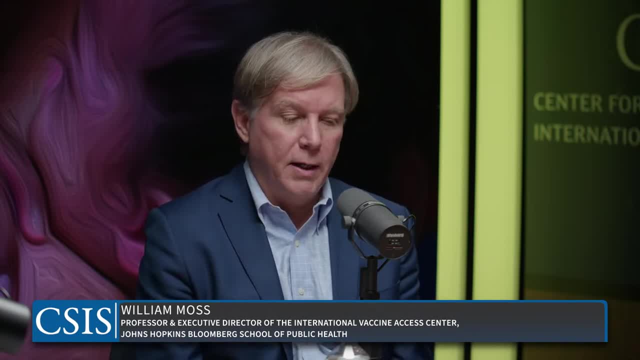 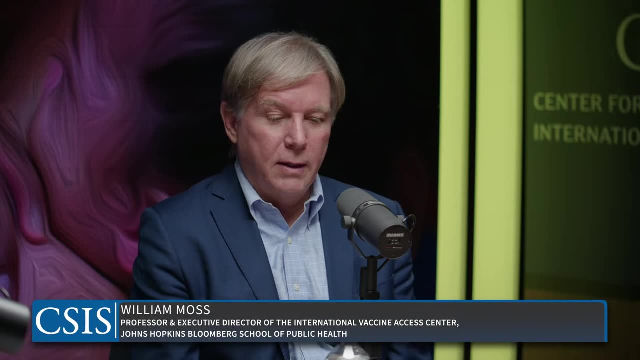 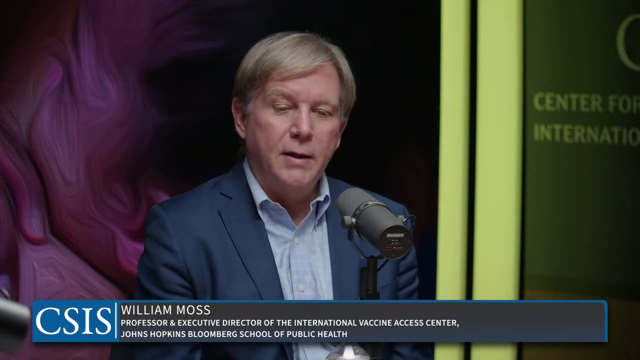 that it's really. it's a spectrum, It's not a, it's not a binary, and people and beliefs can move along that spectrum. And and the other kind of assumption I go into discussions about vaccine confidence- is that I think every caretaker, every parent, every mother, every father wants what's best. 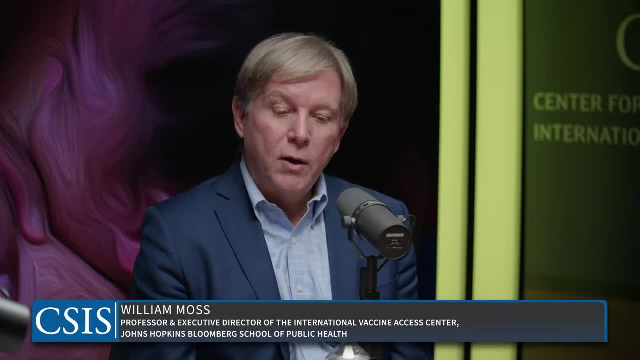 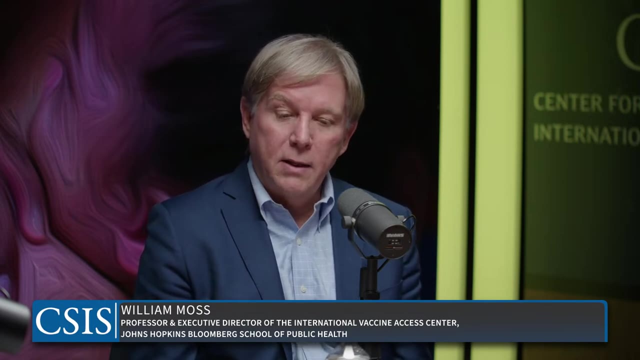 for their children, But they and so they're weighing risks and benefits And And That calculus is different than for others, And I think what we, as public health officials, need to do is make sure that people are making that calculus, that risk benefit calculus- for their own child or for themselves with. 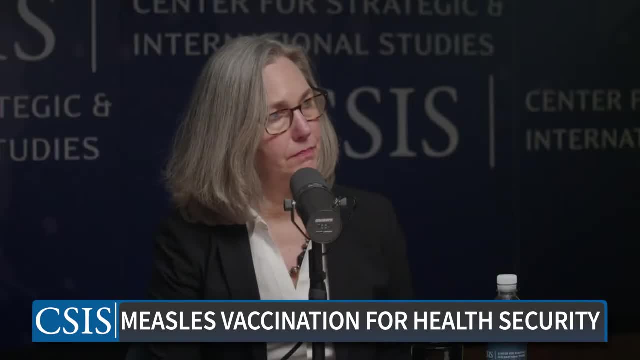 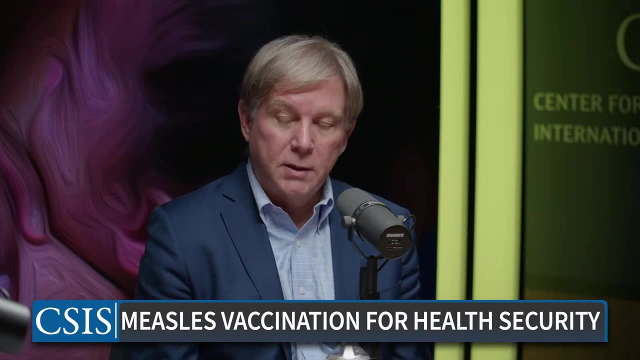 accurate information And there is a tremendous amount of disinformation and misinformation of vaccines, measles virus in particular, historically, But certainly, But certainly, extending to other vaccines. and what can be, I'll say, disconcerting for those of us in public health can be the fact that this is a, this is a long term war, a. 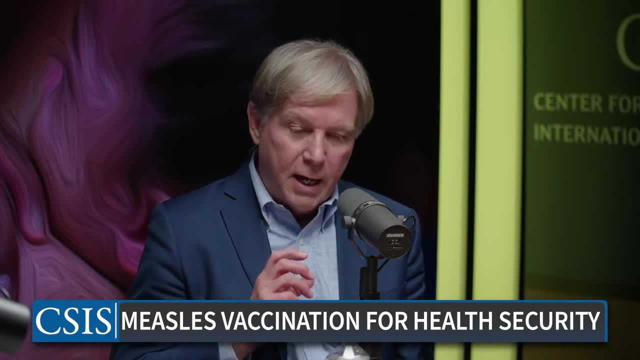 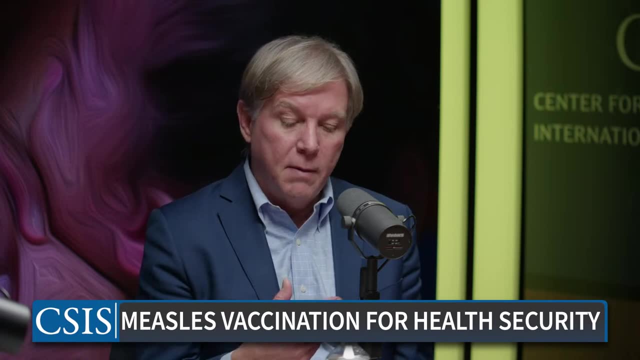 long term battle. This is not something we can kind of flip, you know, or you know, in one activity, you know, turn it around. And just to come back to points That, That's what Daniel made before about the community. 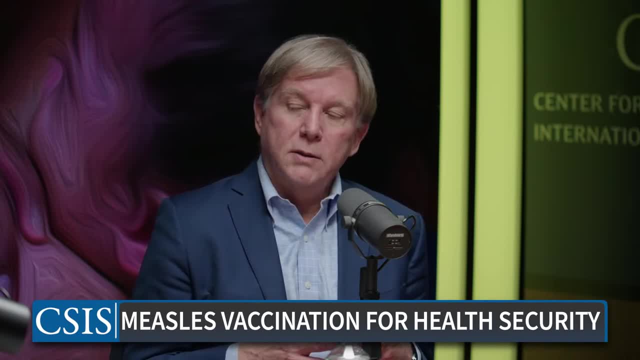 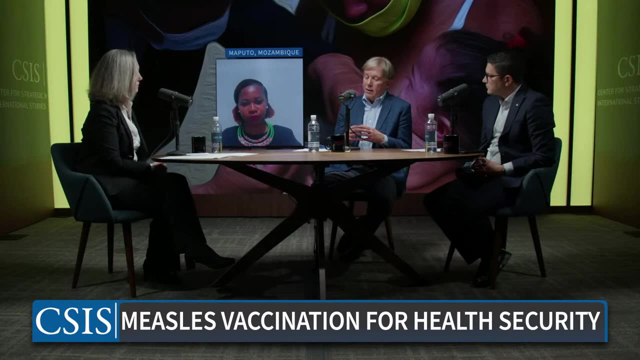 I think you know it's really identifying the trusted messengers within the community. That's so essential. And you know some of the work out of IVAC. I'll refer to the work by Lois Perverdum, our colleague around COVID-19 vaccines in the Baltimore, in the Baltimore community. 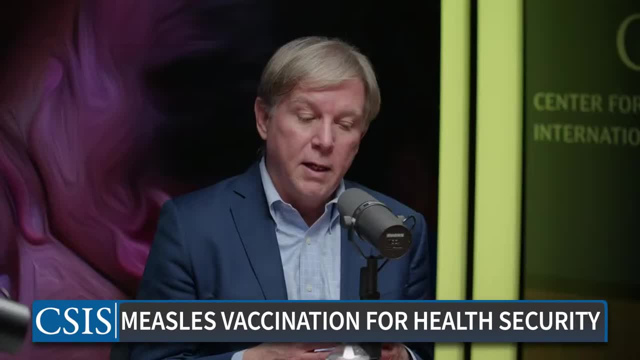 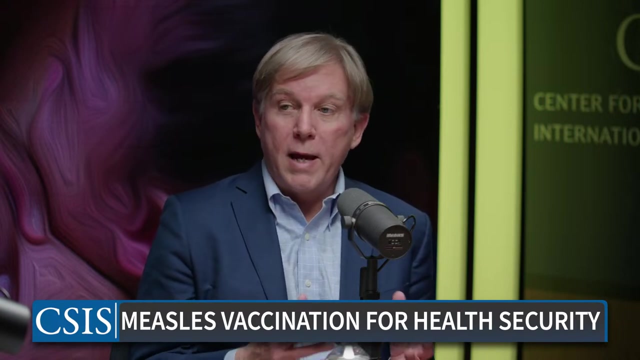 around where Johns Hopkins is and really engaging with the faith leaders, the faith based leaders and the religious leaders and the community leaders and have them be the ones you know, delivering the accurate information and delivering the messages to really try to best inform people as they weigh the risks and benefits of vaccination. 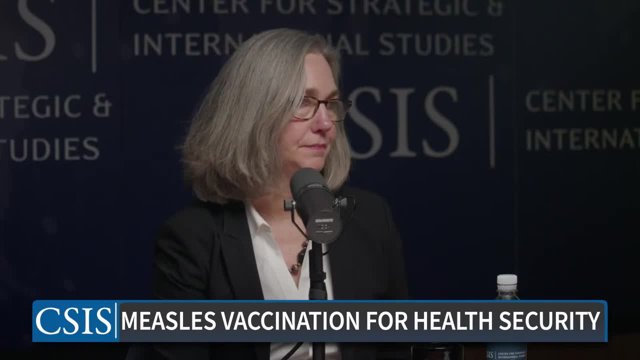 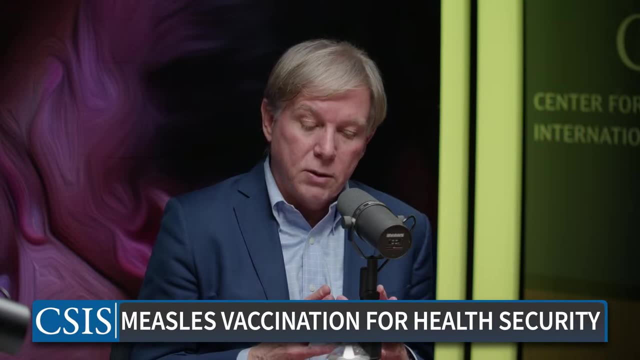 And I think public health officials need to be very honest about what- that there are risks associated with some vaccines And so we need But, But, we, But there's again. we're up against kind of a tidal wave of disinformation and misinformation. 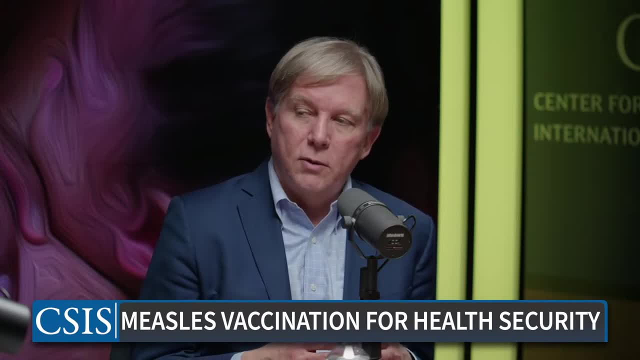 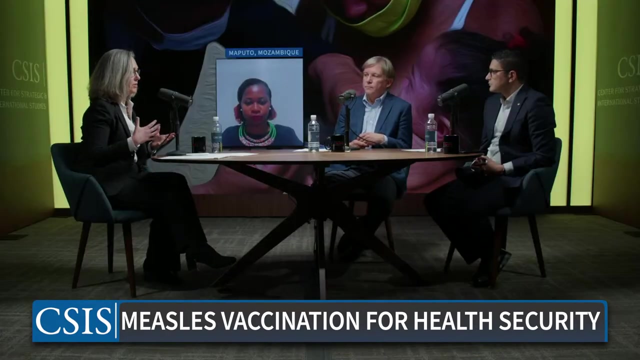 And so this is a, this is something we need to continue to do for the long term to be able to move people along that spectrum and best understand the benefits and risks of vaccination and that, that calculus. Thank you, Danielle, You know, thinking about the region of the Americas I think you mentioned, maybe it. 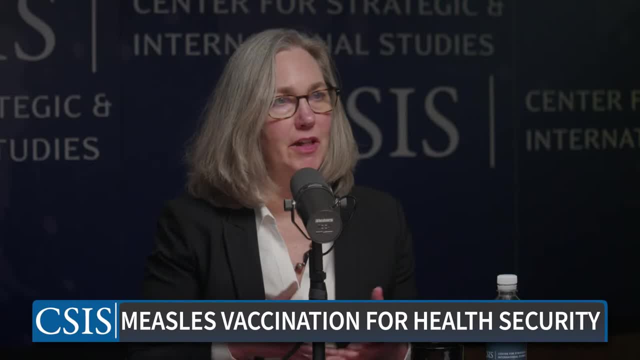 was earlier today or in an earlier conversation, just that health workers in the region had been exposed to so many different messages on social media and you know were different times, you know feeling bombarded by by all of these different messages. What are some of the approaches that you've seen that have been most effective in kind? 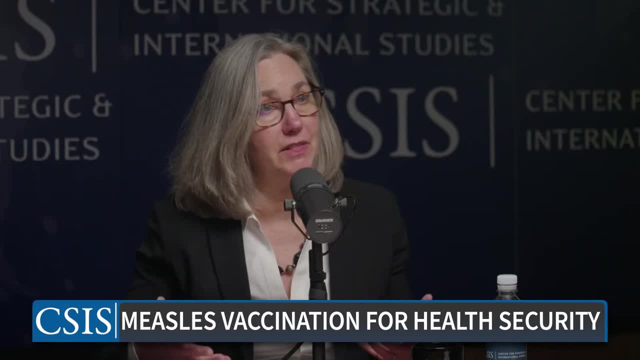 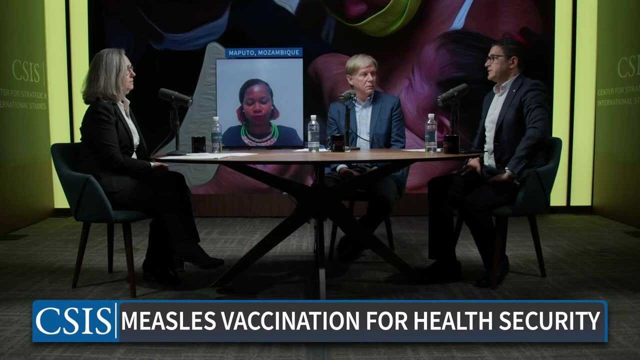 of Provide that community in particular with with the confidence they need to continue providing vaccines. Well, the most important thing is actually to train them to be advocates for vaccination, because usually you train them to know how to manage the vaccine, how to handle you. 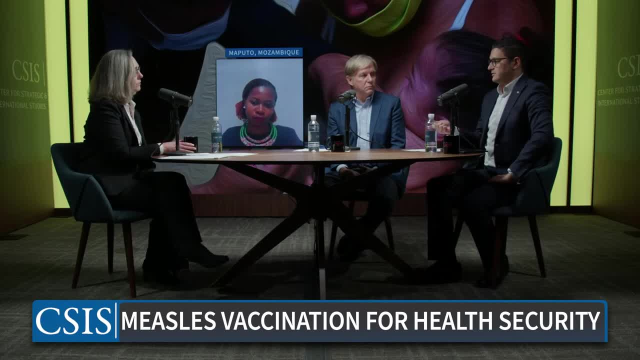 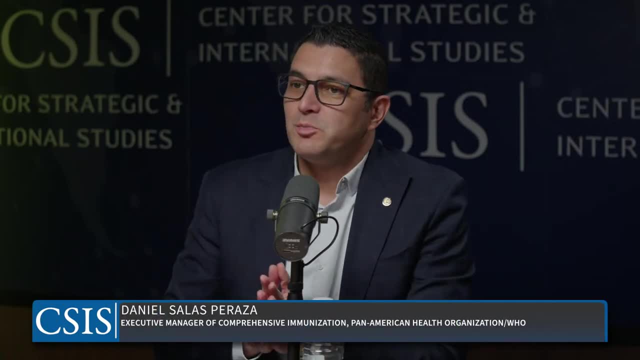 know the cold chain operations and probably you train them, of course, to know about the possible adverse events. the technique, the technique of application, But Usually you do not empower them to be a strong defendant of the importance of vaccination. So that's something that you first have to work with them. 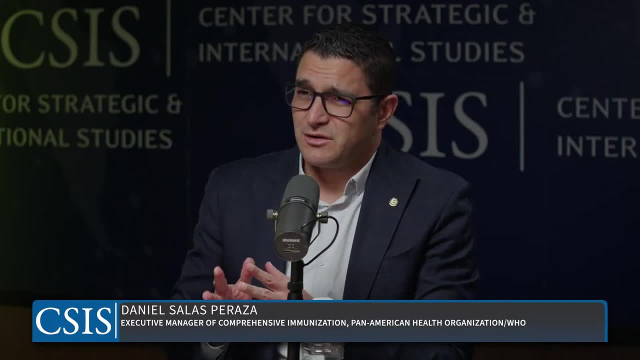 What I have mentioned before is that during COVID-19 vaccination- and I think that COVID-19 vaccination was a chapter, really a specific chapter in our history, especially in the Caribbean- we found that even 32 percent of the nurses were against the vaccination of 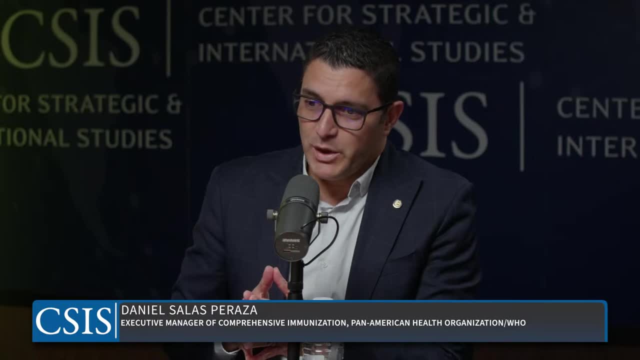 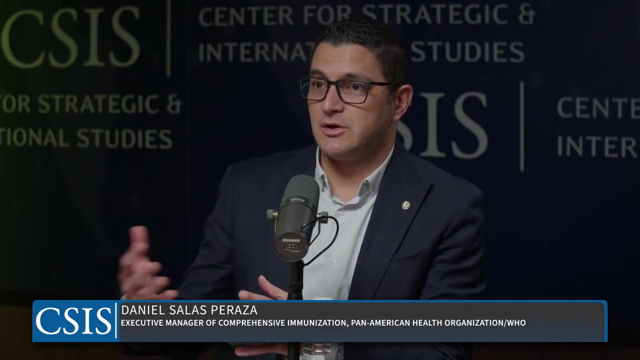 COVID-19. But We have not detected that this has spilled over to other vaccines in the regular program and probably we are facing here two problems, And one of those is the lack of risk perception, because we don't have these large outbreaks of measles or polio or diphtheria, I mean just in specific countries. 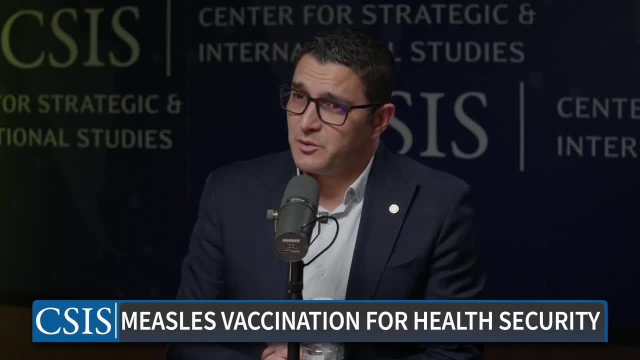 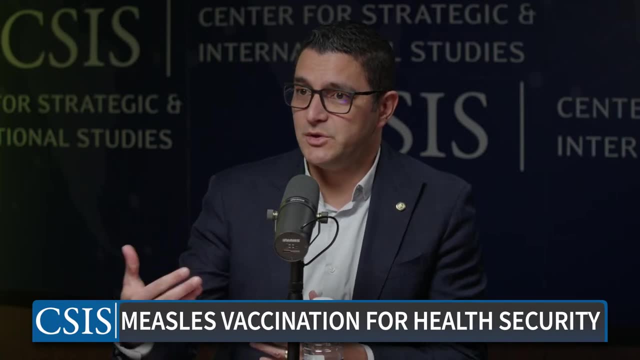 But it is not the case anymore, So I think that that's something that we need to work on and to increase the. why do we need to protect against measles? What are the consequences if you don't protect your, your child, against measles or rubella? 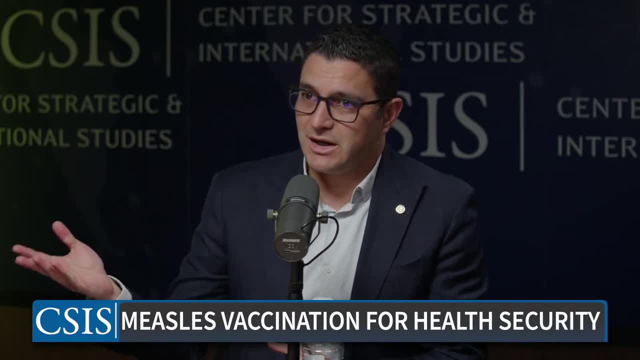 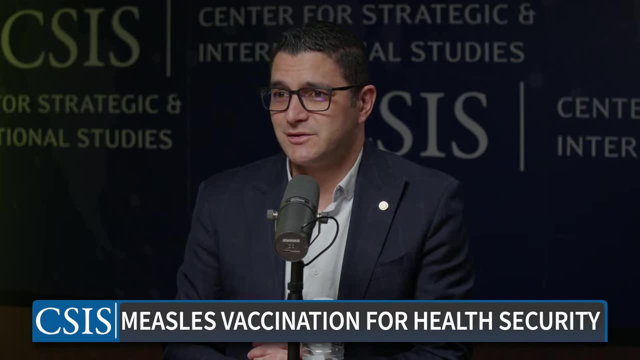 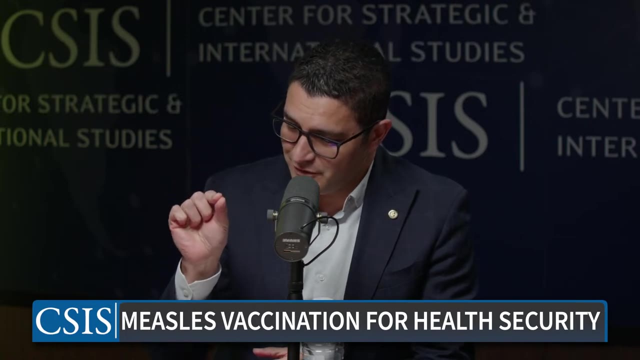 or But, and, of course, the other topic is how to deal with misinformation, with this information and the social media, you know phenomenon has been really hard to to to challenge and to to really, you know, tackle the problem of having just the easiness of, of, of, of tapping. 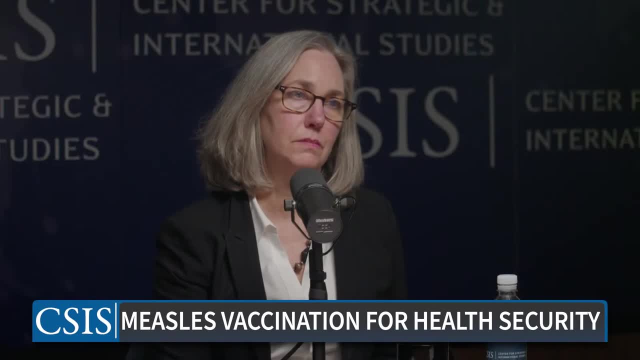 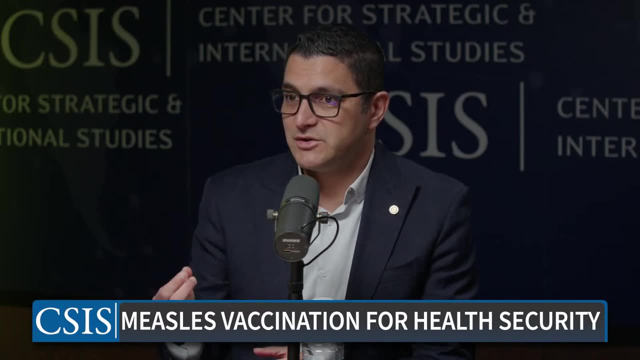 you know, a button in WhatsApp or whatever social media you're using, and and to spread the misinformation, And even I have received from professionals in health care. some of the messages trying to are asking me: is that true And it's something that is completely unfundamental. 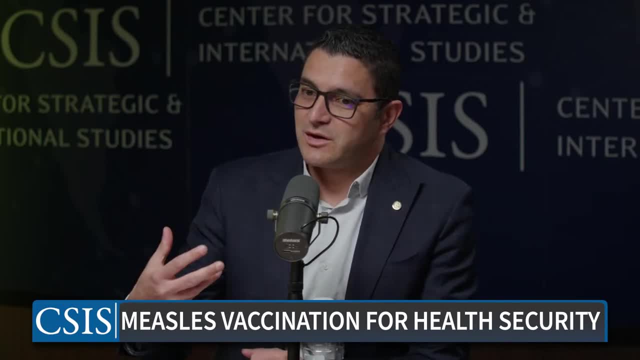 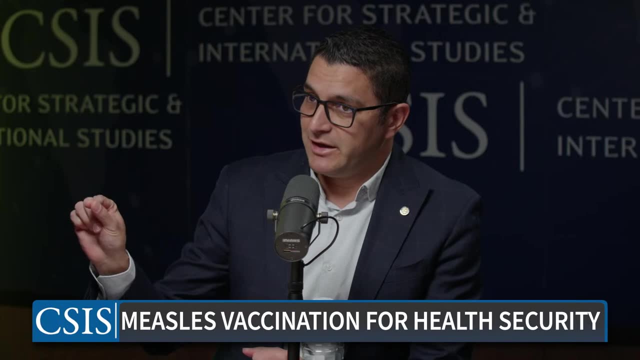 I mean it's, it's, but that that we need to work on how to timely tackle those fake news, for example, to identify the, the leaders and at the community level it is very important- But also, in the social media, how to identify the positive examples. 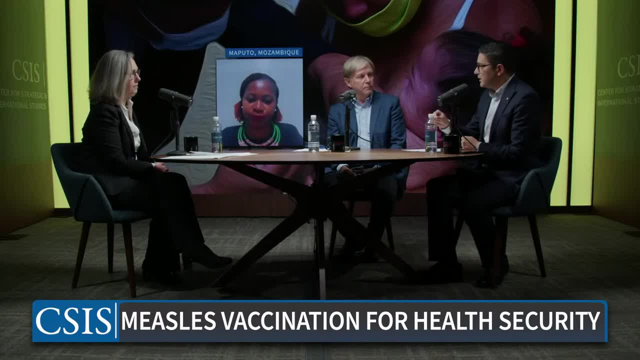 So I think it's really important. I think it's really important, I think it's really important to identify the positive examples of, of, of of you know, leaders that can really help us in the social media platform to you know, rapidly tell. 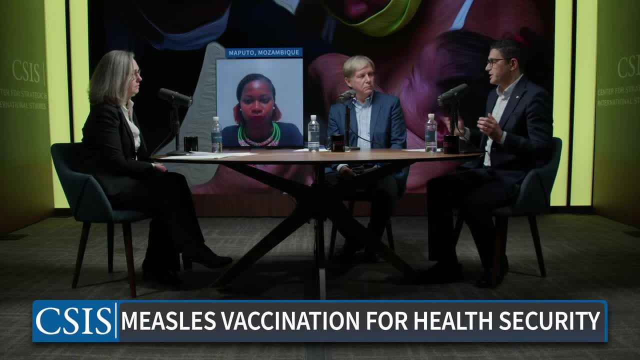 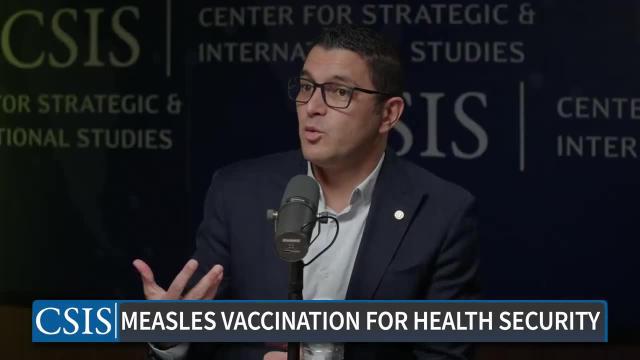 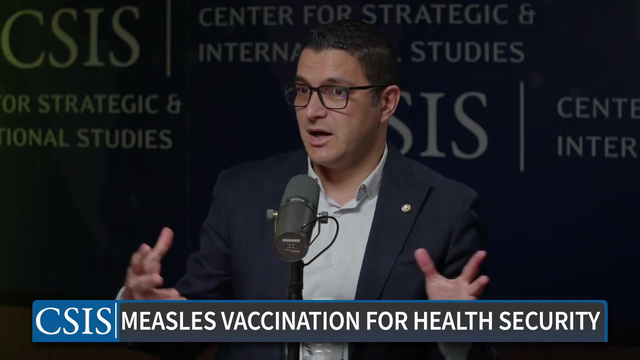 the truth about the fake news or whatever that is spreading out. So that's something that we really need. to continue working on the social listening, We now have social listening tools But, OK, what to do with those? Or are you detected on a timely manner if fake news is really spreading out and causing? 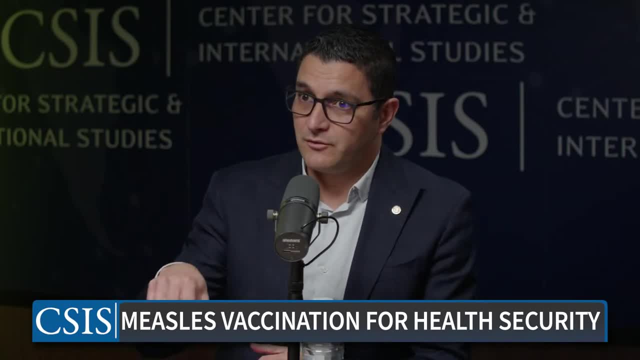 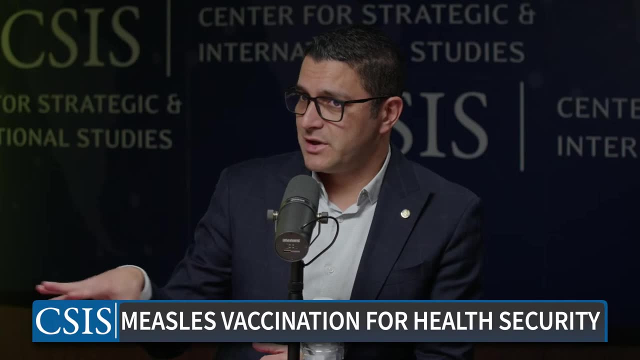 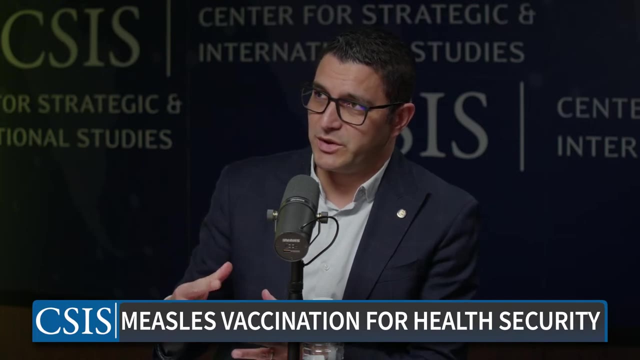 you know, like these kind of doubts or whatever, What we have found out during the follow up campaigns is that, for example, for MMR vaccine, that people are still very positive about receiving that vaccine, even when we had some kind of problems where there was a combination of using the COVID-19 vaccine at the same. 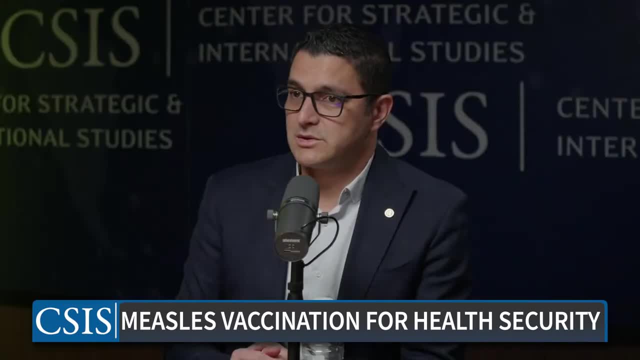 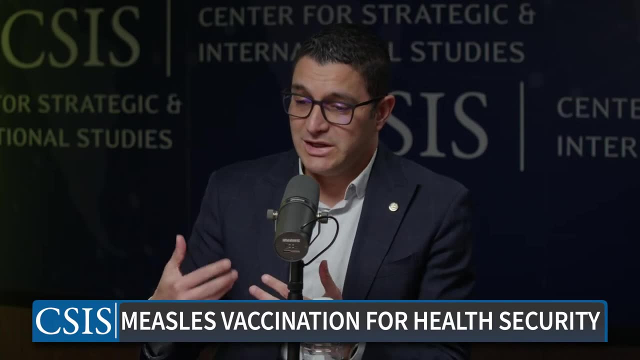 moment or applying the vaccine when the when the measles vaccine was was applied. But of course there are a lot of misinformation about the COVID-19 vaccine. But You know we need to really continue training our health care workers to be very dependent. 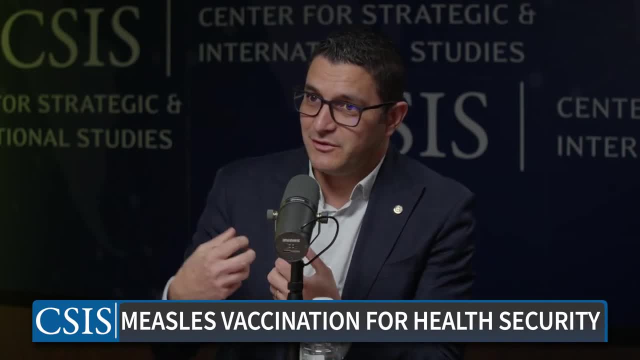 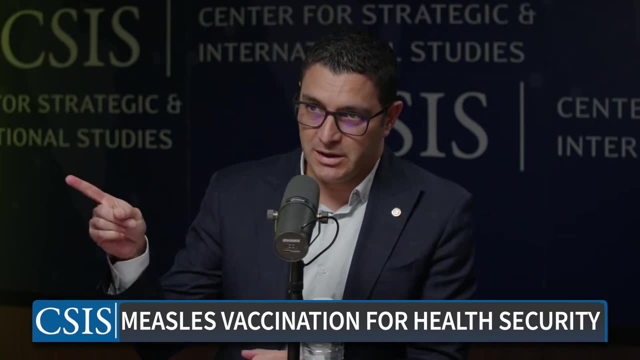 very you know, like leaders, to to to give the all the elements to the people of why it is important to vaccinate against X or Y vaccine but at the same time, try to identify those leaders at the community level, the religious one, the the ones that you know. 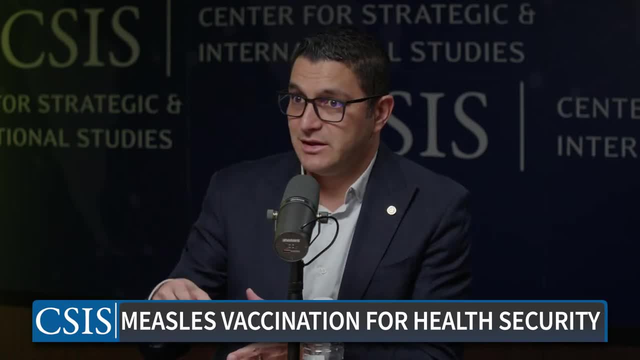 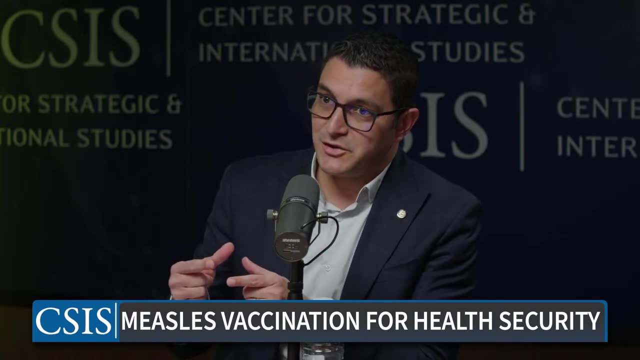 can really know where are the houses of the children that are not vaccinated and why do they think the way that? I mean it is more at the social Media, you know, level to identify the leaders, the, the, the, the influencers that can really 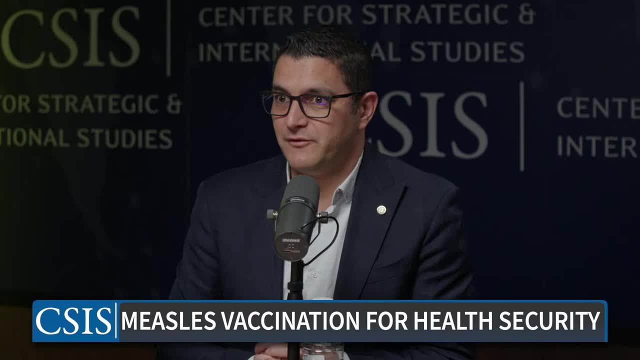 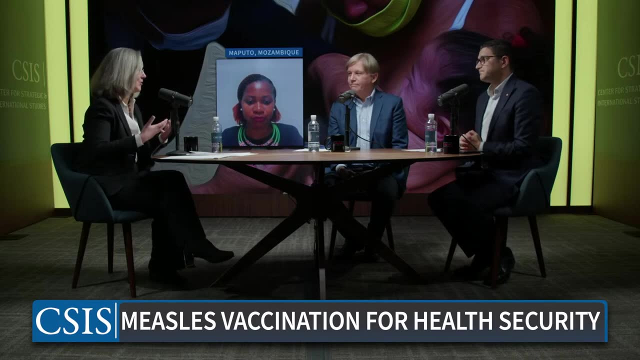 help us to, you know, to dismedify any kind of fake news. That's interesting. You said people are trained to deliver the vaccine, but not not the communication about why it might be positive to to take it. Graca, let me just ask you, you know, are you have you seen kind of an impact from the? 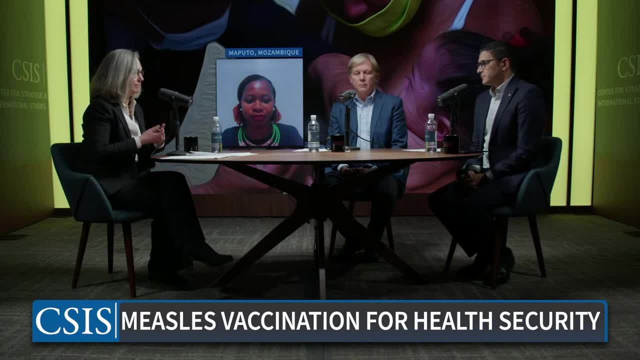 vaccine. Were there any tensions or, you know, hesitancies around the covid-19 vaccines You know did? did you see that spill into kind of some of the feeling about measles as well? Yes, definitely. Covid-19 vaccine had its own challenges and I won't repeat what Daniels has mentioned. 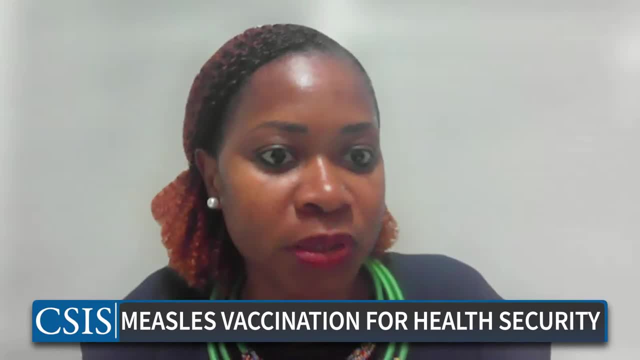 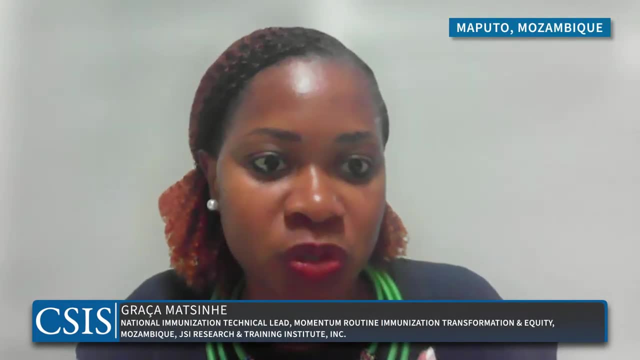 because the scenario was was pretty the same: health workers not wanting to vaccinate, communities not wanting to vaccinate, And we needed a very strong communication strategy to make sure that they do accept vaccination. And we saw that when the cases started to increase. that's when people really started. 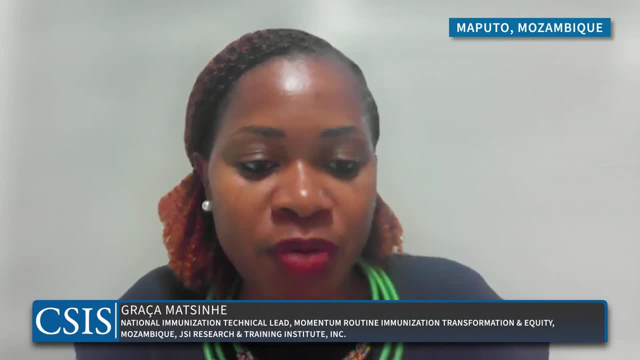 to to seek for for the vaccines. However, for under under five immunization, we don't experience the same challenges. I have the perception that these vaccines are much more accepted and communities tend to accept more easily, which is not happening, For instance, when there is cholera outbreaks, which we not vaccinating only children, but 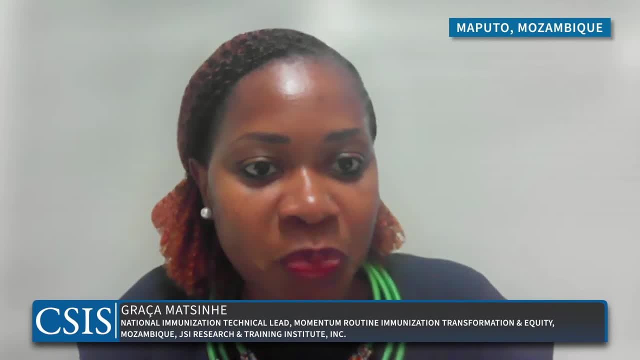 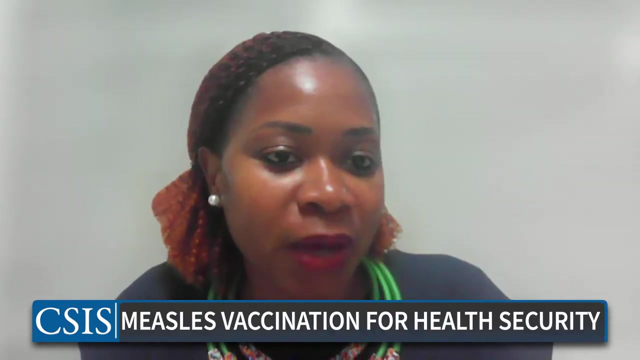 we're also vaccinating adults. There are lots of myths and misinformation around cholera vaccines, But we also see challenges and some hesitancy in HPV vaccines, where people believe that the vaccines will cause infertility In the case. so those are some of the issues that the vaccines bring, especially when 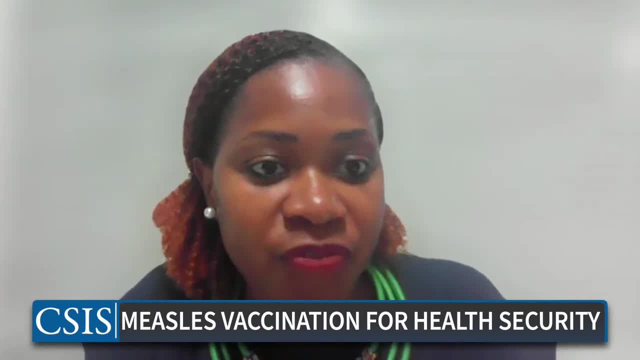 it's a new vaccine and not targeted to the under five. So community engagement, involvement of the community structures, the leader, be it religious community leaders, political leaders, at the at the more peripheral level, This has been very crucial to make sure that people will accept the vaccines. 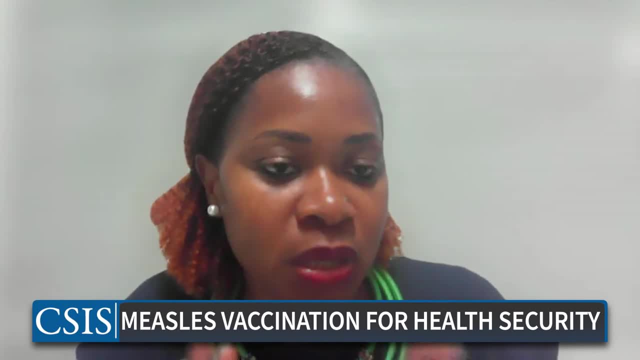 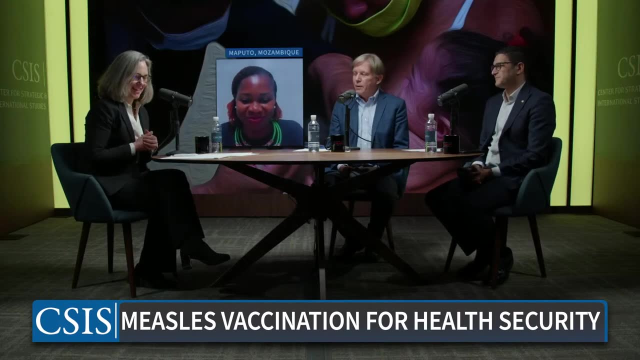 And also the myths and misinformation are dissolved. Well, thank you. So we've covered a lot of ground in the last hour or so. I want to you know, we we kind of started out looking back at, you know, the year 2000. 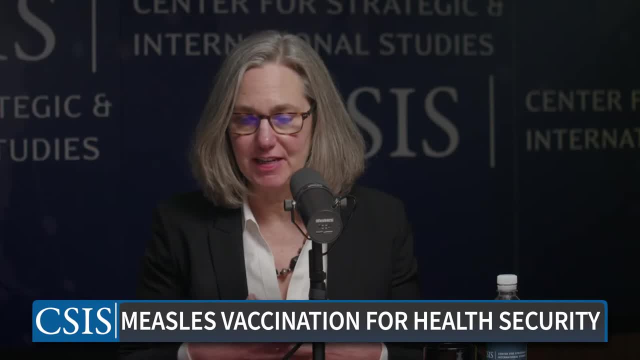 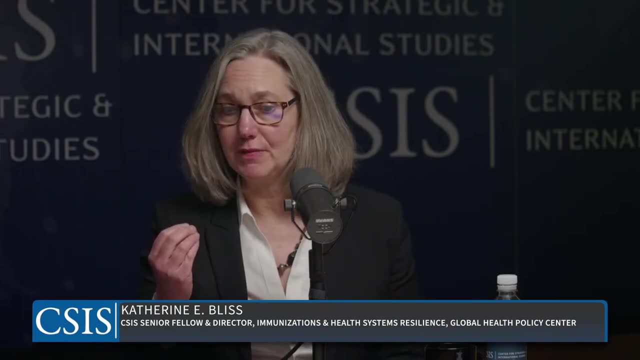 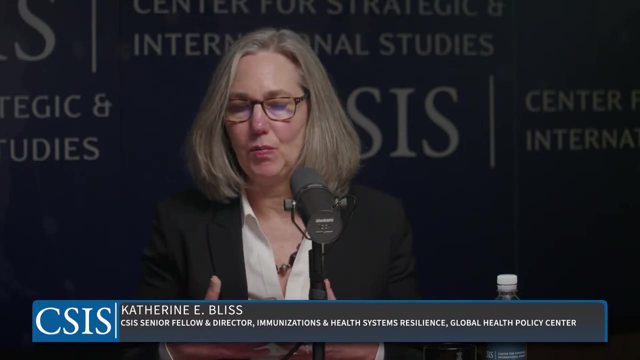 and even back to the 1960s with the introduction of of the vaccines. Let me ask you each just to maybe offer just one or two very brief, you know, kind of little predictions or looking ahead. But let me ask each of you to, you know, just say, you know, as you think about the effort. 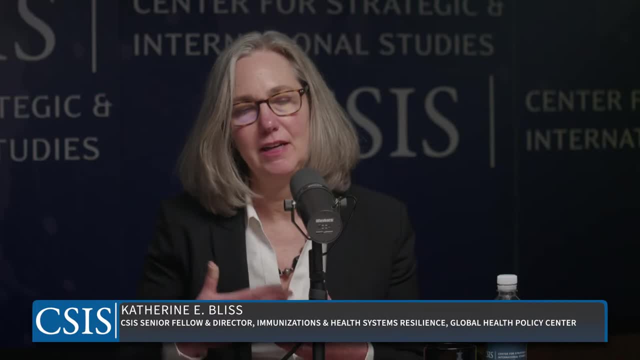 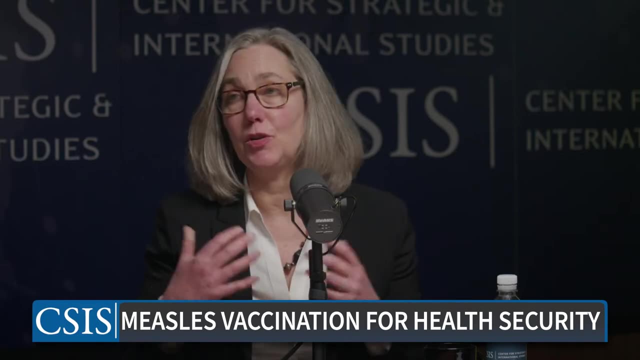 to eliminate measles and protect global health security, kind of looking ahead to 2030 or so, or beyond what, what is? what are one or two kind of developments on the horizon that you're most optimistic about or most excited about as you look ahead? 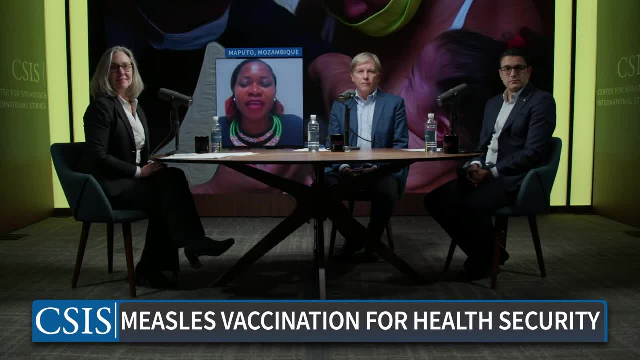 Graca, let's let's start with you. Well, Catherine, what comes to my mind is that we have come a long way. The the immunization programs were established around 45 years ago. in Africa especially, However, the threat of measles continues to be real. 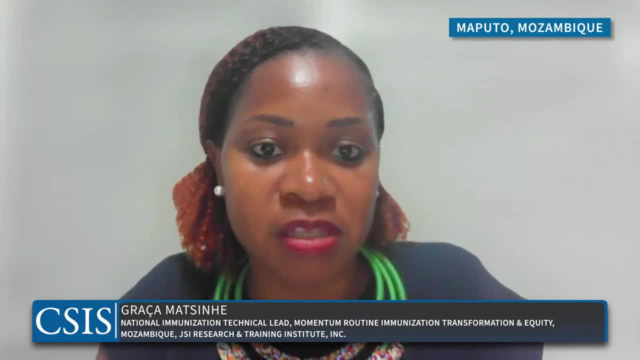 And we need to take collective measures in order to halt this, this threat. We need to strengthen community surveillance, We need to improve the visibility and funding of routine immunization and the health systems as broad, But we also need to make sure that the 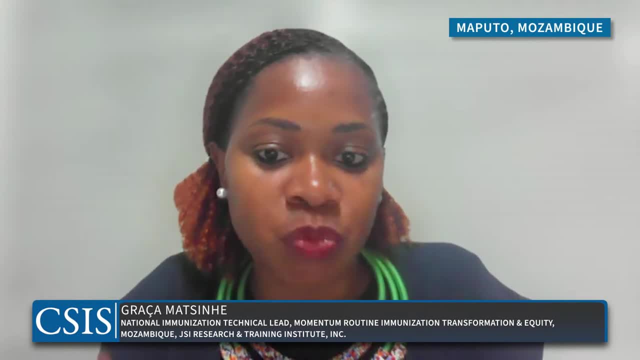 Measles efforts are very well aligned with routine immunization, the micro planning of the campaigns, the integration of intervention and the resource, the resource sharing. I think those are the key issues to make sure that we- we as a global community- will be defeating. 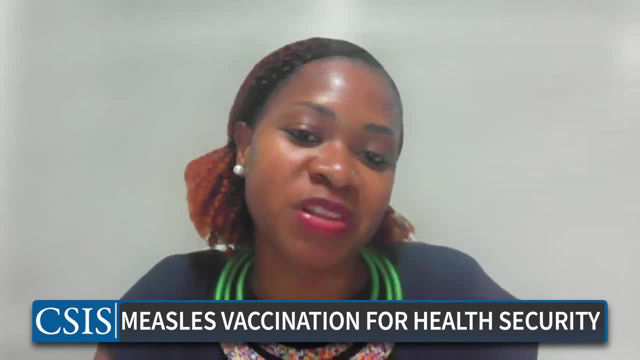 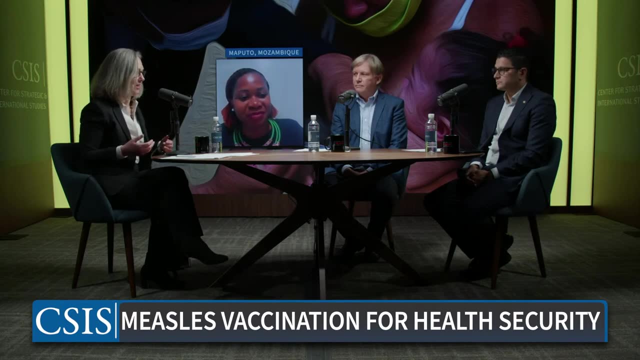 this enemy, which is the measles and other vaccine preventable diseases. Thank you, And that's right. This is the 50th anniversary of the expanded program on immunization, Right? So coming up, big celebrations, I think in April or so, Daniel. well, we have these global. 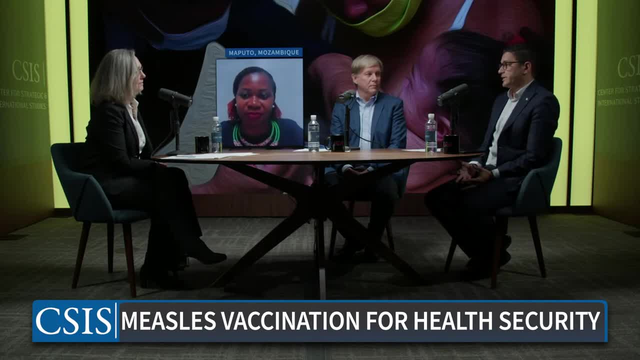 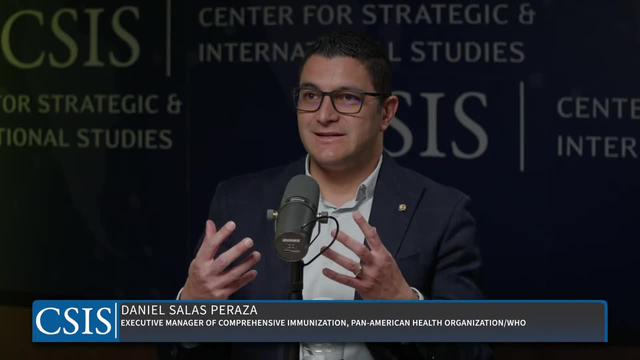 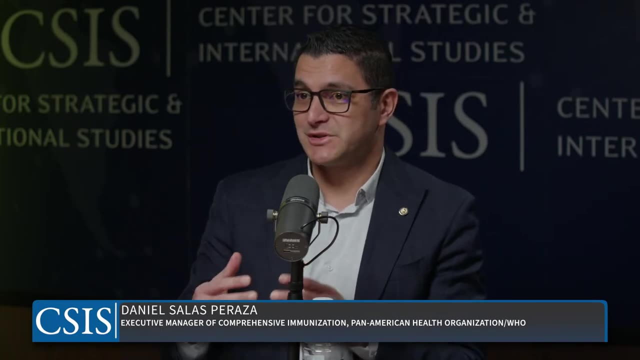 framework to work on immunization, which is immunization agenda 2030. And there is a lot of partners supporting that agenda. But I'm enthusiastic to see that you know that level of coordination at the global level can really translate into a synergistic approach at the country level, because I think that 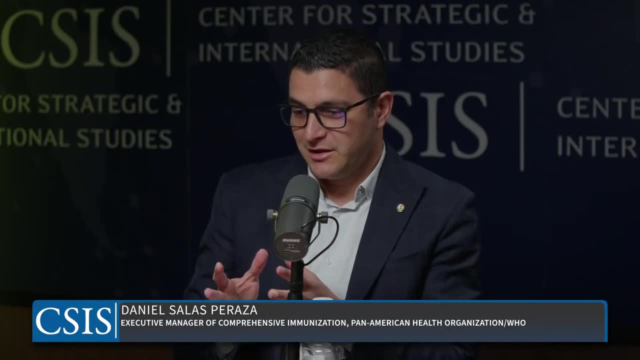 there is a lot of ground to move forward in terms of really integration. Thank you, Yeah, I mean again. I think we have to continue to be more inclusive, you know, in terms of integrating, you know our efforts, our possibilities, our capacities in different, you know, partnerships. 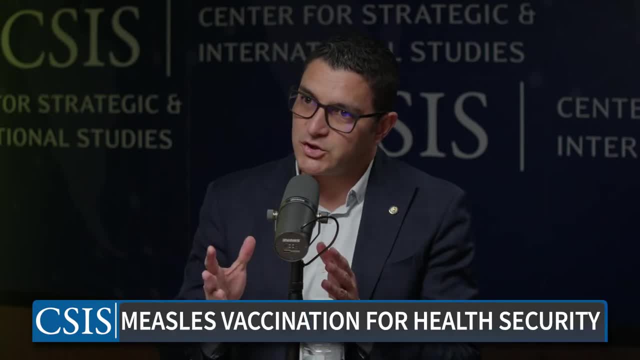 that we have the different partners to really see the country and see how can we help that country in a very comprehensive way. that that's something that it's very positive, But I think that that immunization, the immunization agenda 2030, was somehow interrupted or disrupted. 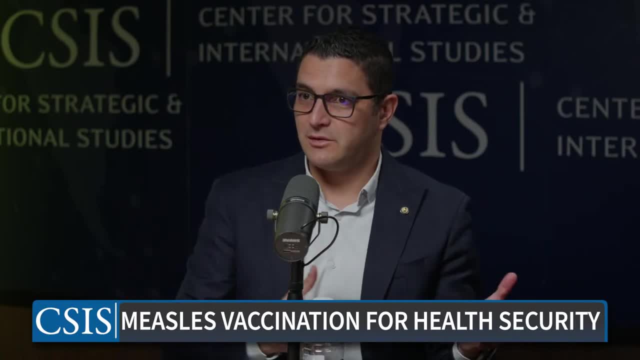 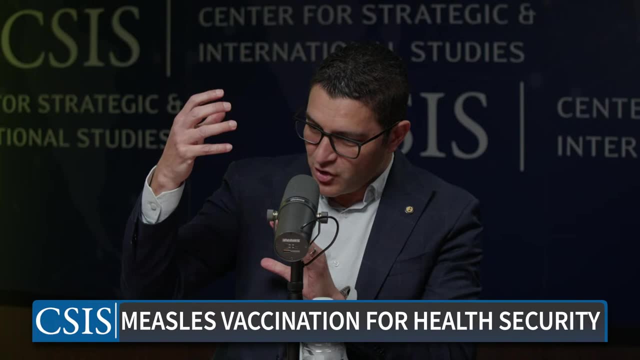 by the pandemic, But now we're trying to recover. you know the, the efforts And really we need to that, Yeah, to really have a coherent coordination at the global level, at the regional level, but at the country level as well. 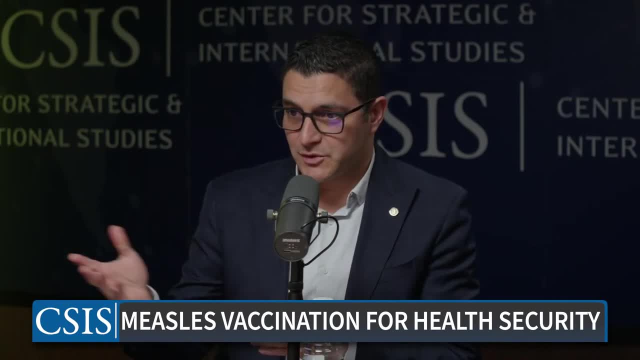 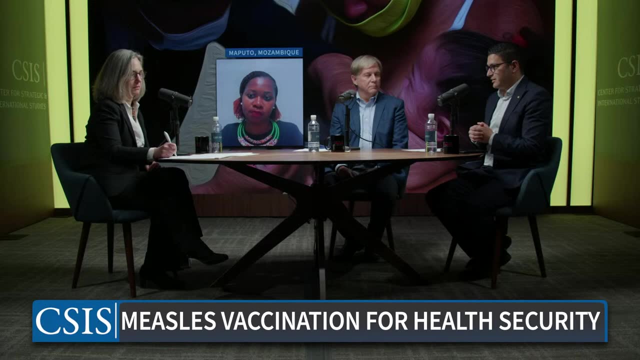 So I think that that's very positive And at the same time, of course, these new kind of technologies, as Bill mentioned, the microarray patches. we have conducted a workshop in Guyana here to see how they see this technology. how can we have some kind of feedback? 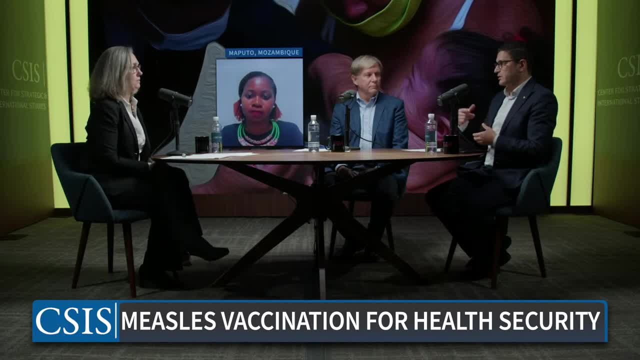 to improve that technology, And now we're going to conduct in March in Brazil another worship about that. So that's something that can really be a game changer, as Bill mentioned. So that's something that is very positive and really have me excited about the future. 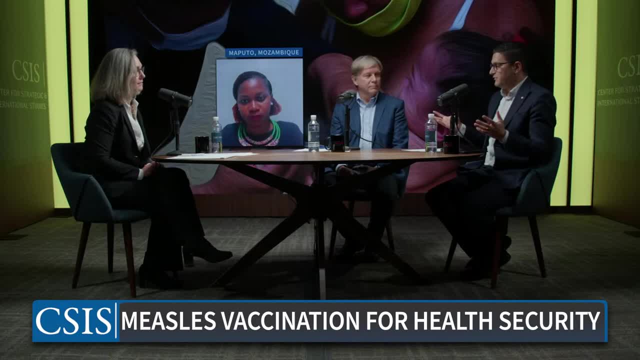 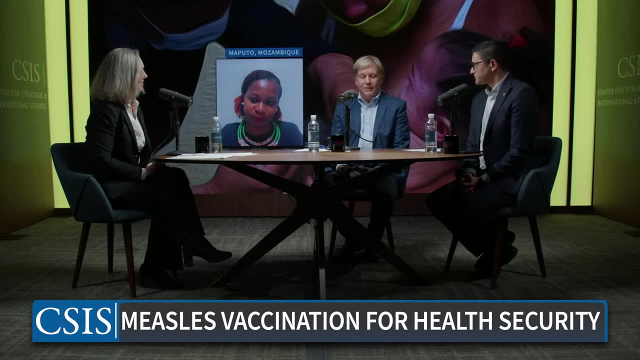 that we could have with this new possibilities of even you don't need a nurse to apply this vaccine. This could be really a game changer at all. So that's something very positive, Bill. Yes, I'll tell you very briefly. I'll just say what I hope to see in the next decade. 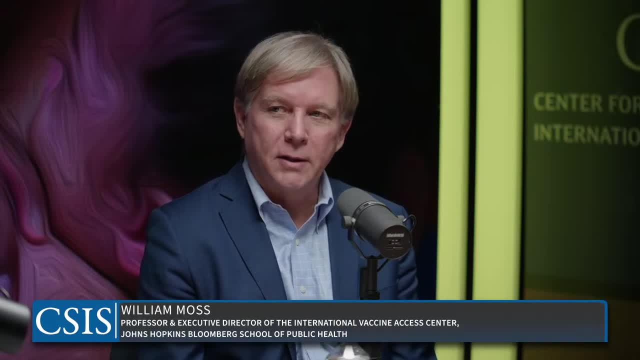 is a real pathway toward measles eradication. We've talked about a number of different strategies: the tools, the technologies. I think we know how to do this, I think we can do it, but we need a clear path to achieving measles eradication. 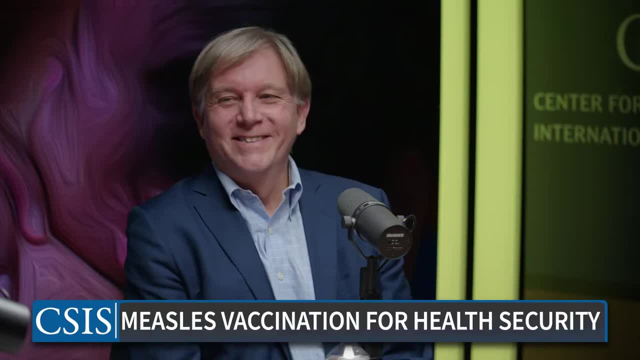 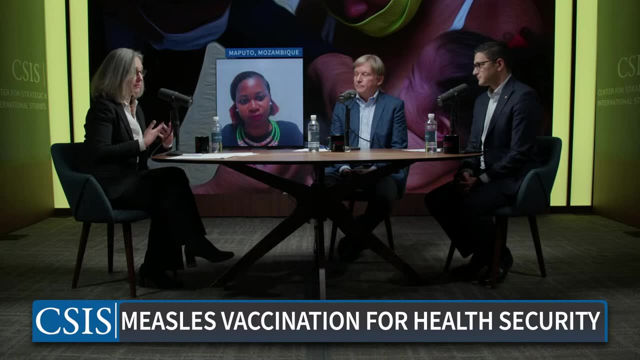 So that's my big hope. So we have technical possibilities, opportunities for greater collaboration, collaboration in terms of financing and economic outlooks, governance, new frameworks and positive options with respect to the challenge of social media, but also positive options in terms of using new social media.